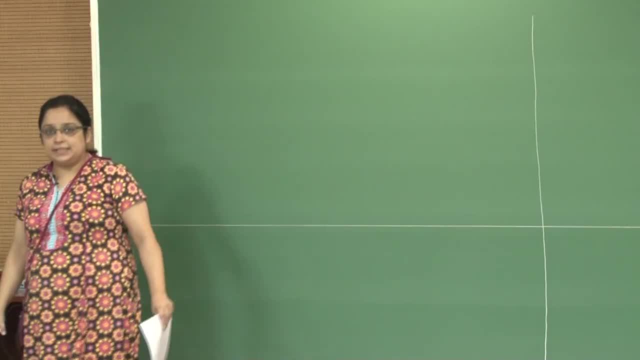 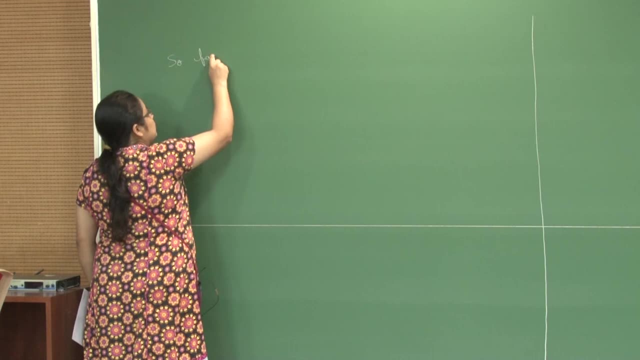 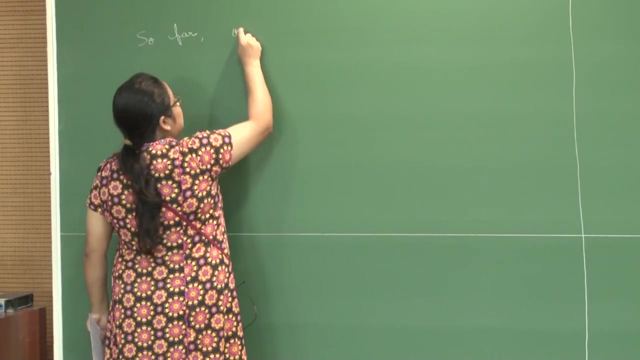 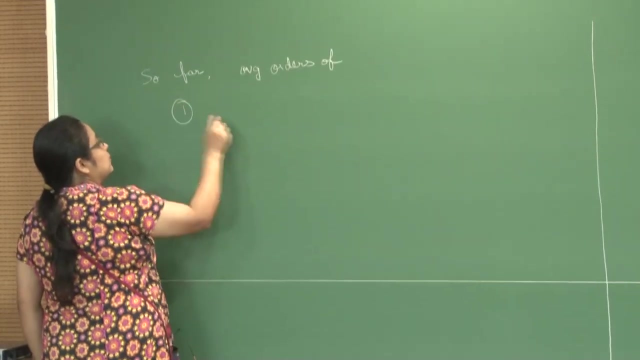 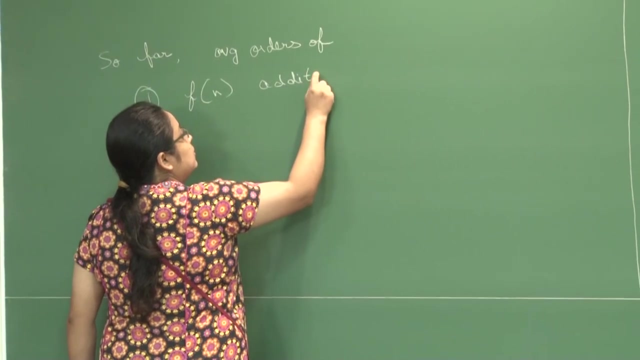 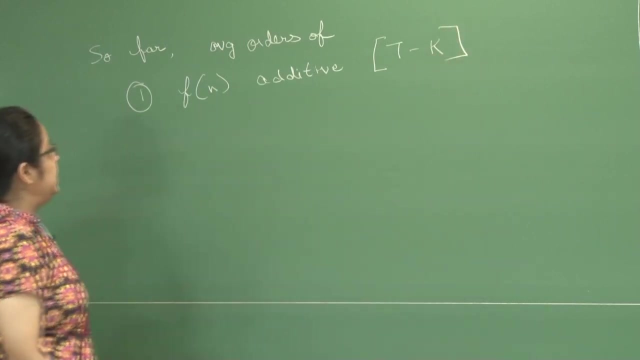 So we resume our lectures again after the mid-sem exam and the mid-sem break. So so far we have learnt about different techniques to evaluate average orders of functions which are additive. So this was the Turan-Cubillius inequality. 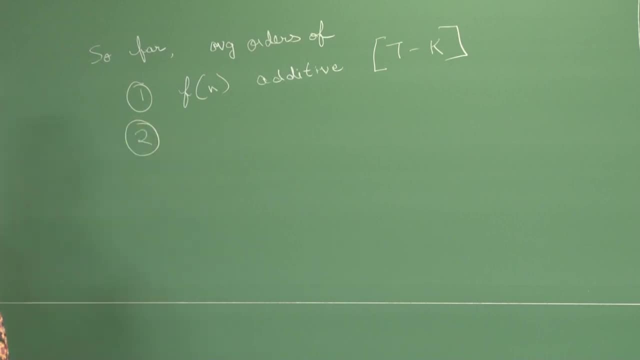 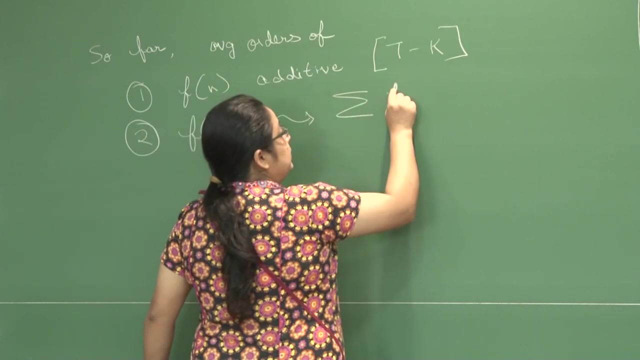 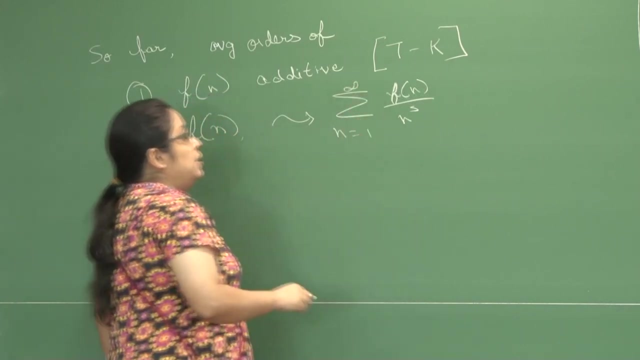 Then we also looked at a technique called Perron's formula, which teaches us how to evaluate average order or estimate it in terms of analytic properties of the Dirichlet series f of n over n to the s, and this technique works very well for suitable classes of arithmetic. 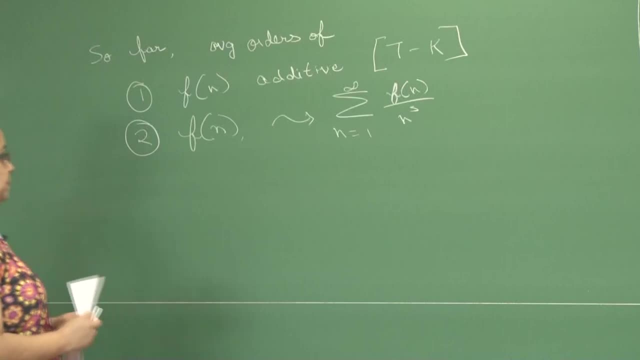 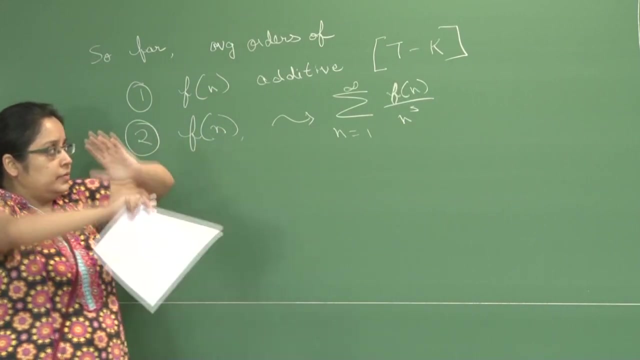 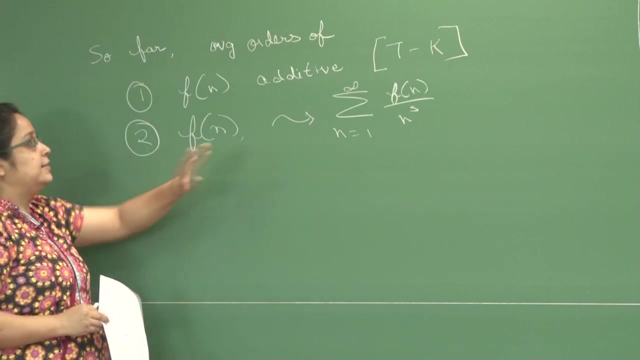 functions, not necessarily additive or multiplicative. The idea is that you should be able to analytically extend the Dirichlet series into a function which is of a nice form. So so far, and we used the second, the latter technique to also derive the prime number theorem. So this is essentially what we have done. 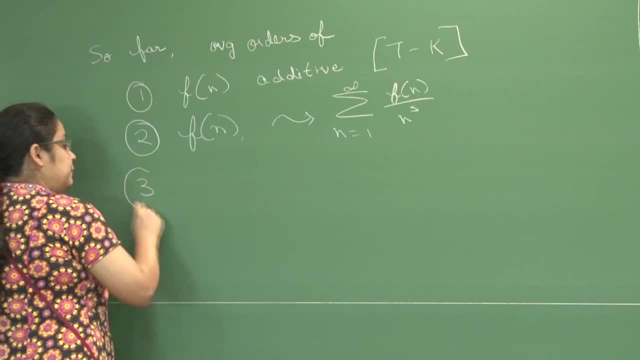 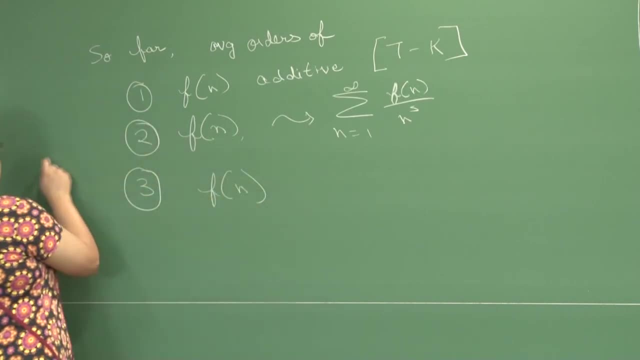 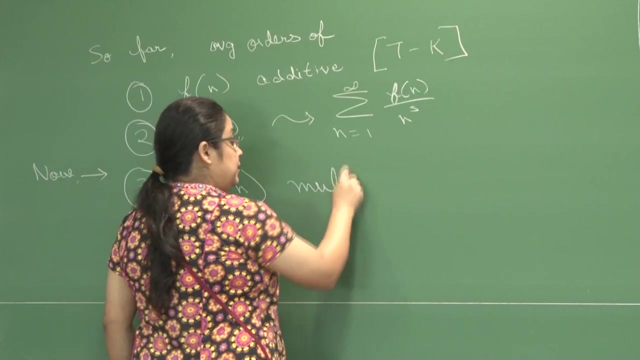 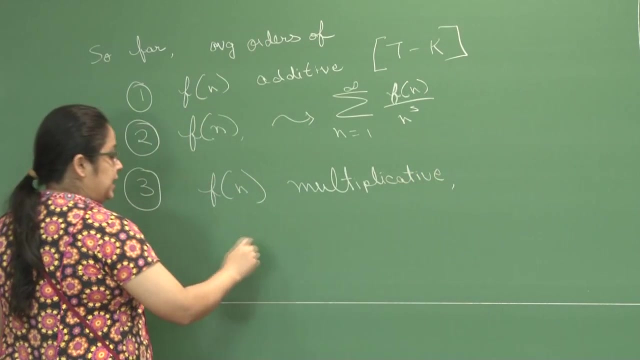 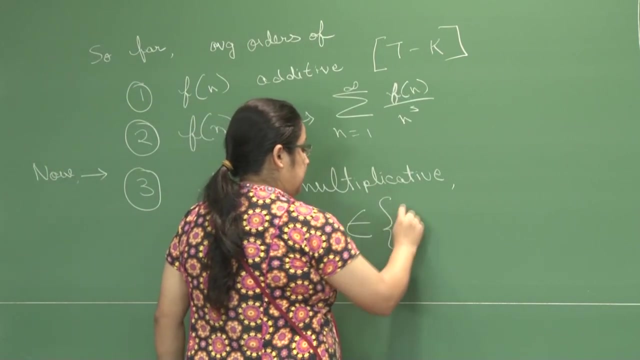 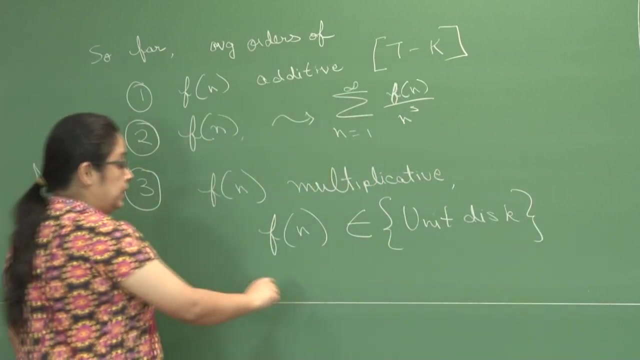 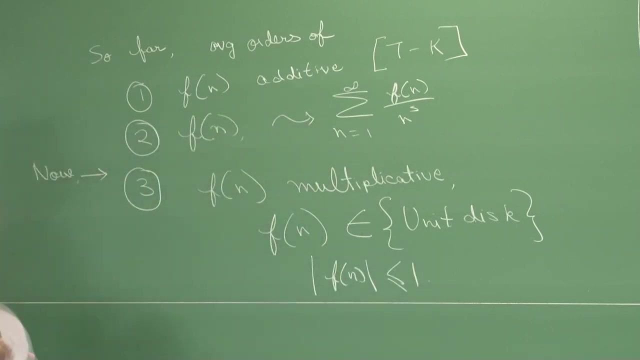 so far. Now we are going to learn some very beautiful techniques to estimate average orders of functions, of functions which are multiplicative and which takes. take values in the unit disc, that is, your absolute f of n is less than or equal to 1.. So these could. 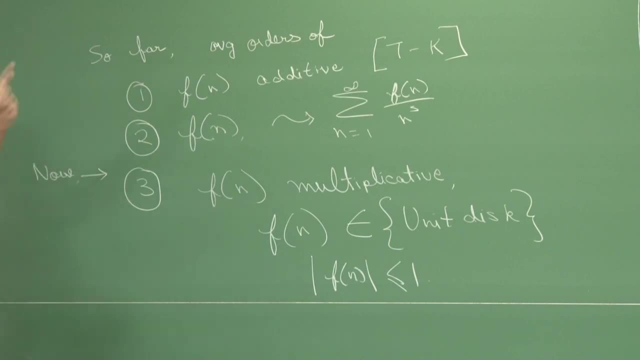 be complex, valued functions, but they lie inside the unit circle. okay, So before we start understanding how to evaluate or how to estimate average orders of these type of functions, let us give some motivation for both these functions. for both these topics- 1 and 2, we had suitable motivation coming from probability, and likewise for the third. 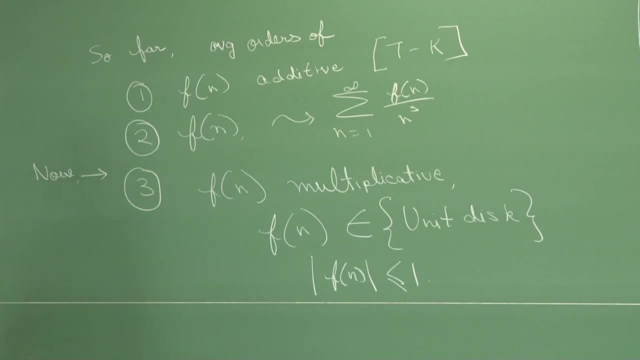 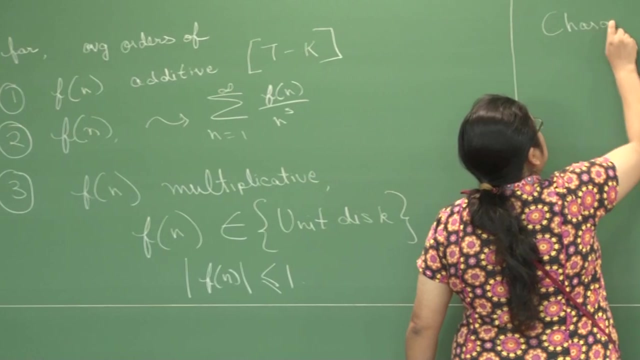 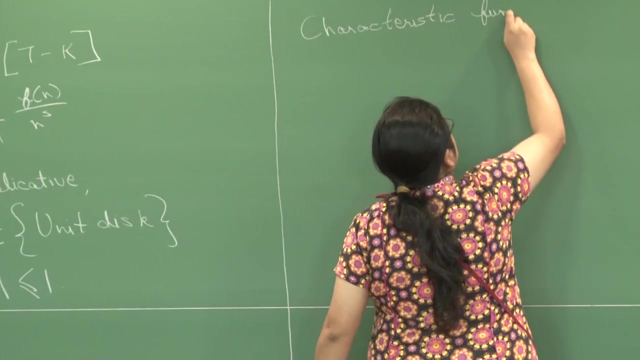 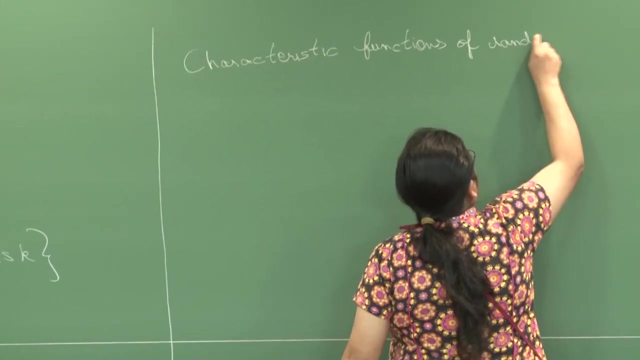 topic. also there is a very nice probabilistic motivation. So for this we have to review quickly the notion of characteristic functions of random variables. So here is the situation: we have a probability space infect a sigma algebra lambda of X equal to 1 combination. 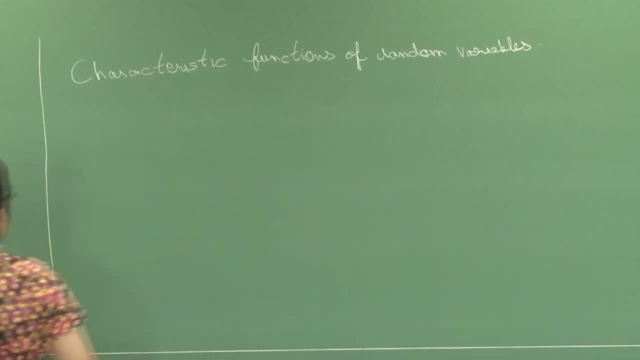 with Naval pressure, X, 1 is equal to Y, So take a kind of one, or would rather take different for the same particular function. familiarize yourself with the transformation. So here the transformation is provided at доб V, negative X starts becoming d minus VxE under e square in the third order direction. 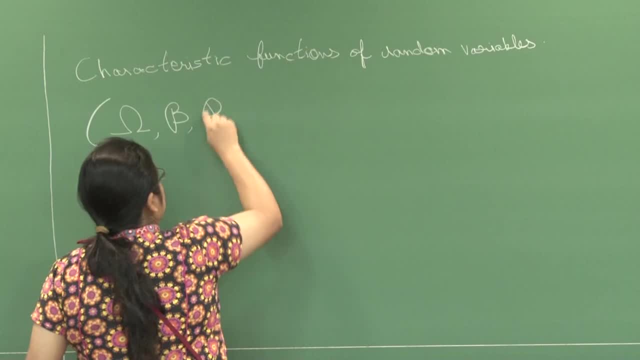 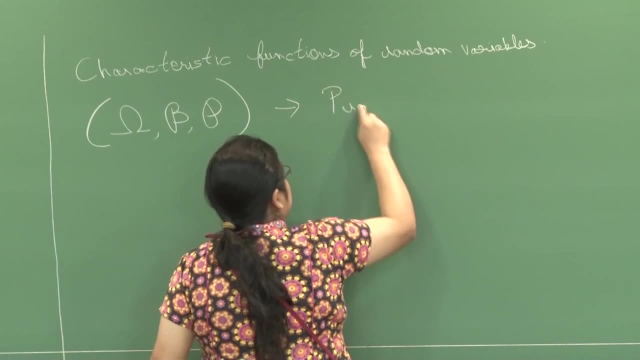 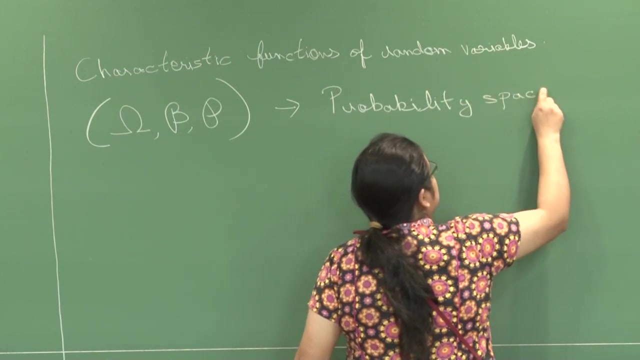 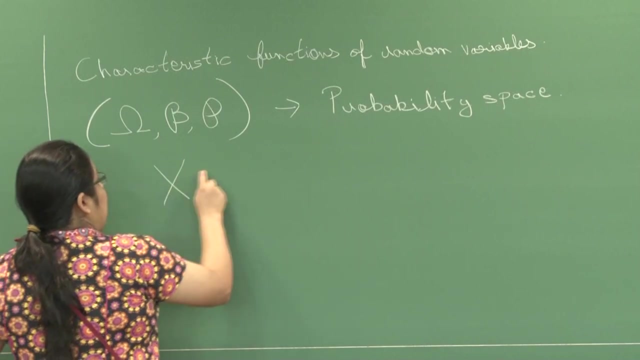 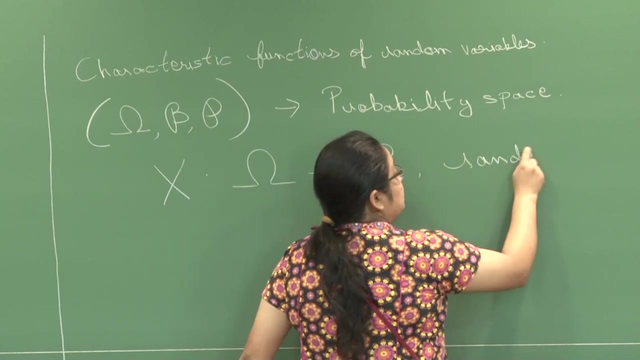 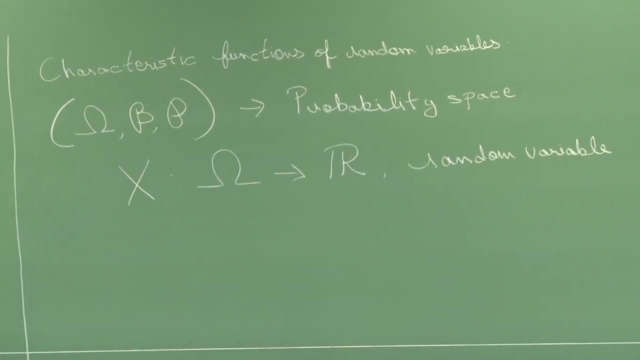 And here you saw that our model is the following: to witness the transition of terms: A to VxE: algebra on omega and a probability measure. So this is a and X. let X be a random variable on the space and let us take real value- random variables Now corresponding to a random variable. 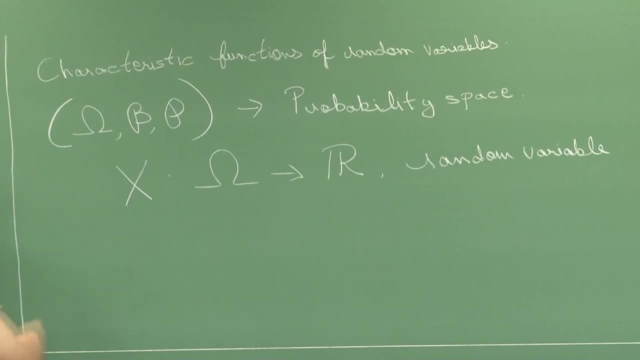 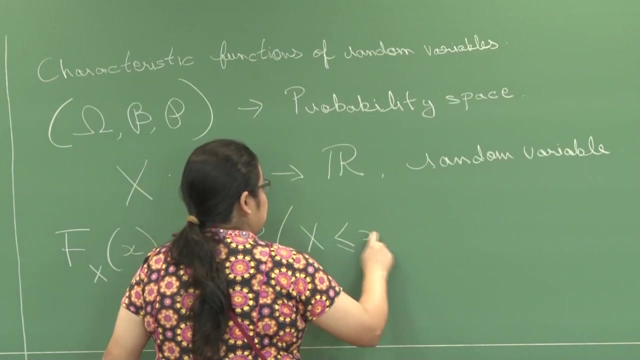 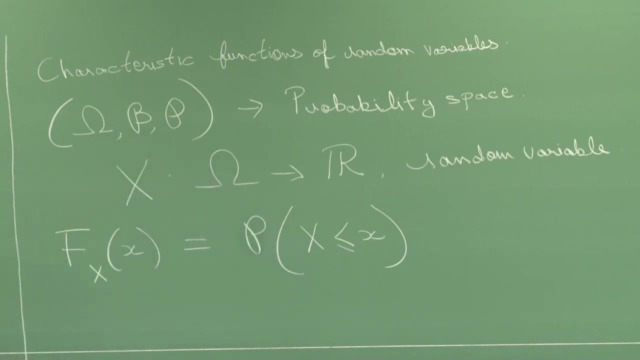 we have the notion of distribution functions, So f sub X of X, for any X in R, for any little X in R. So f sub f of X is the probability. So this probability is the same as the probability here. So probability of capital X less than or equal to X. we all know that this is called. 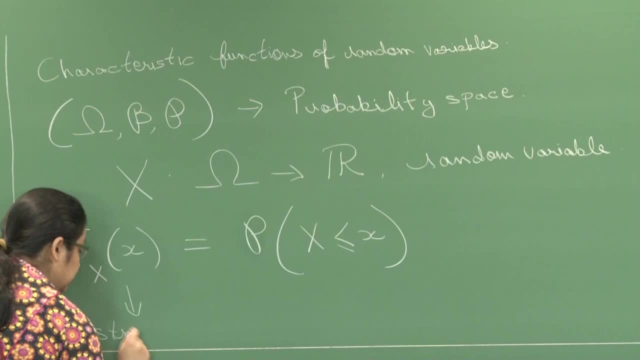 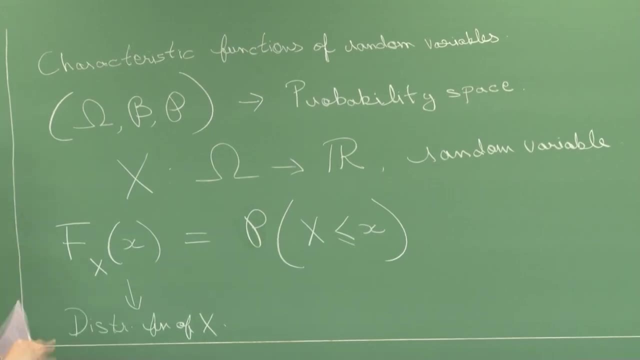 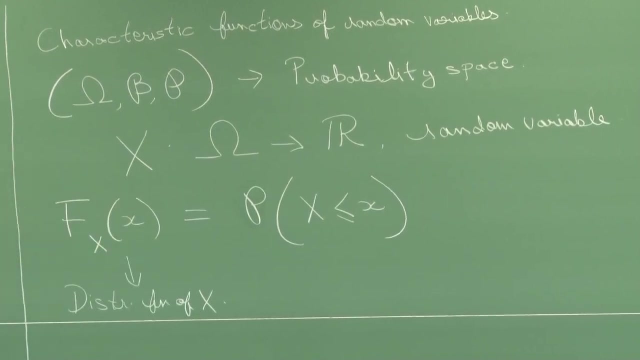 the distribution function of X. Alright, so we want to study. So we want to study the existence of the distribution of X and related to average orders of certain nice functions. So this takes us to the notion of the characteristic function of a random variable. So what is this characteristic? 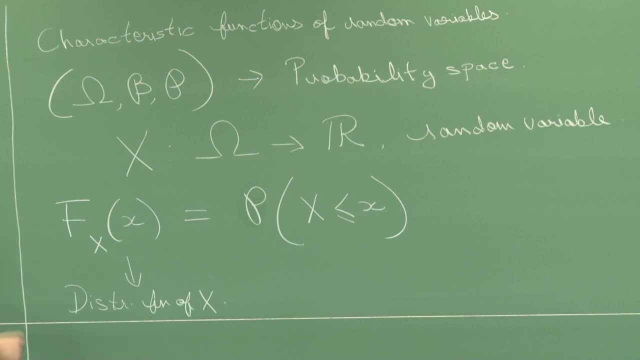 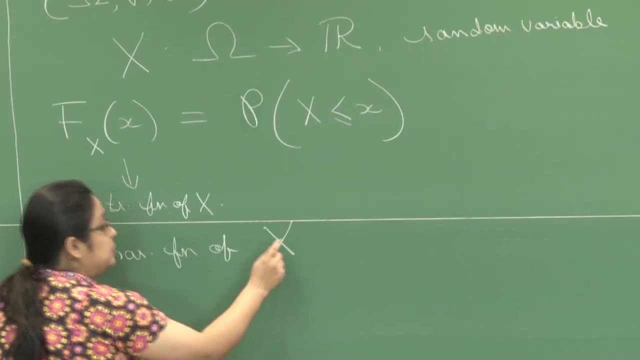 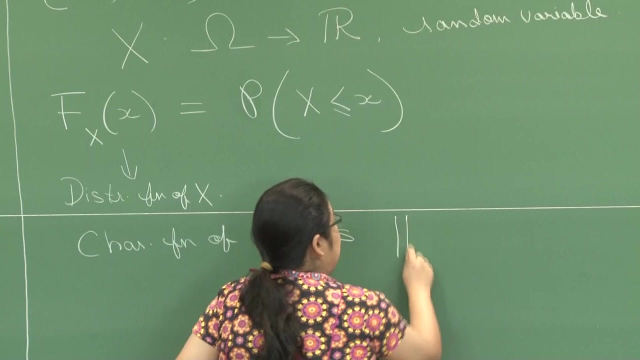 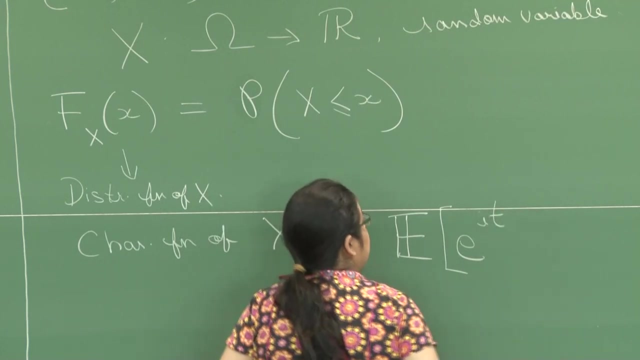 function. It is defined as the characteristic function of random variable X in the probability space as given above. is defined as the expected value of e raise to the i t of the random variable X. So if capital X is a random variable, e to the i t x where for any t, okay. so this characteristic 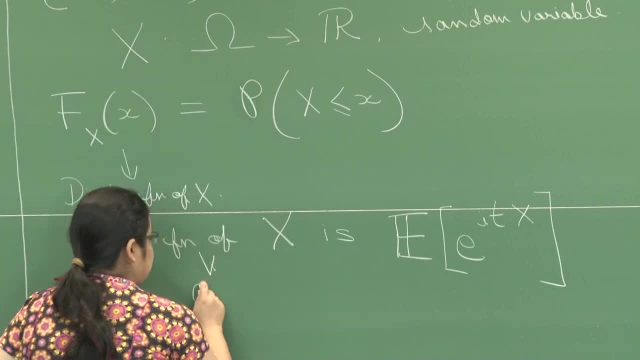 function is denoted as phi of t, not to be confused with the Euler phi function. So phi of t is denoted as the expected value of e raise to the i t x. So what is the importance of the characteristic function of a random variable? before we come, 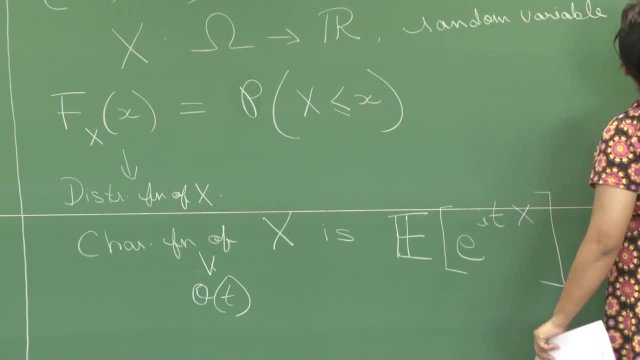 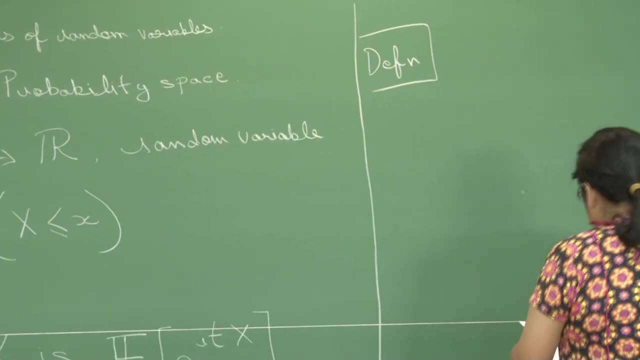 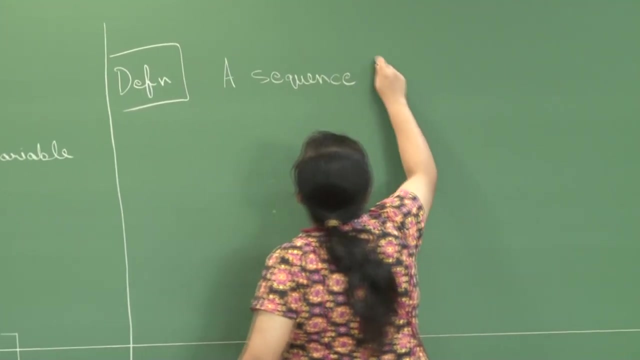 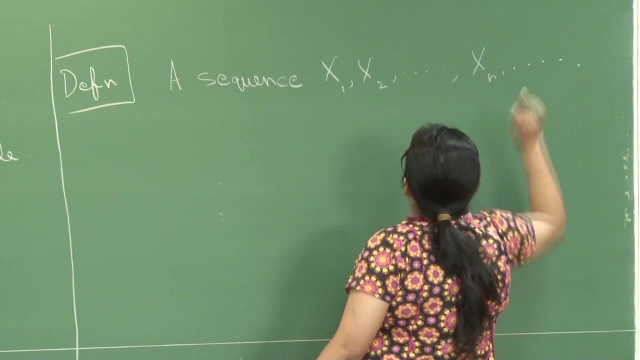 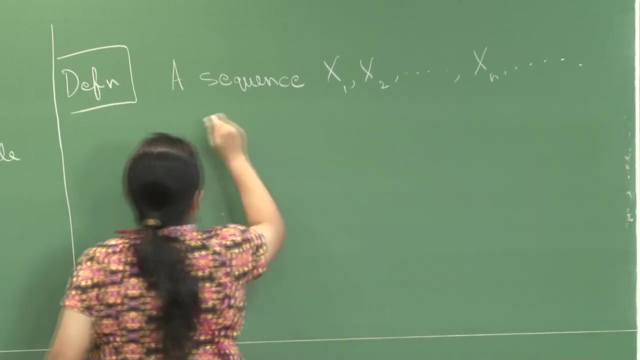 to that. let me just also define Another notion, namely that weak convergence. so suppose you have a sequence X- 2 of random variables, not necessarily on the same probability space. So if you have a sequence. So if you have a sequence, 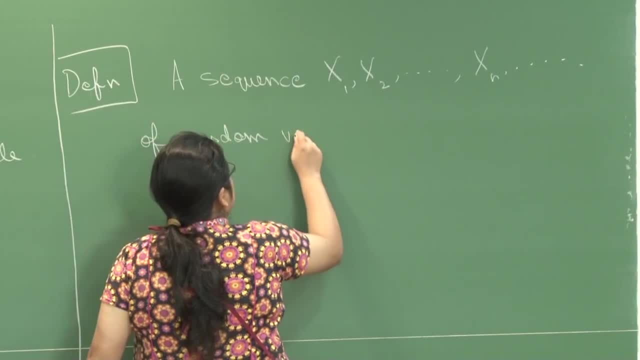 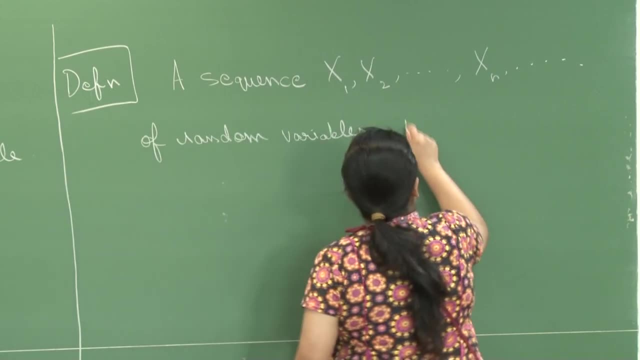 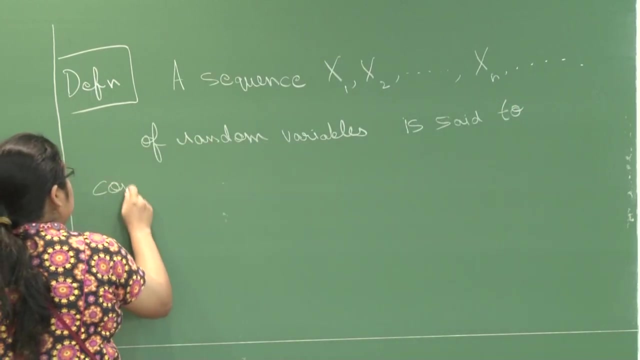 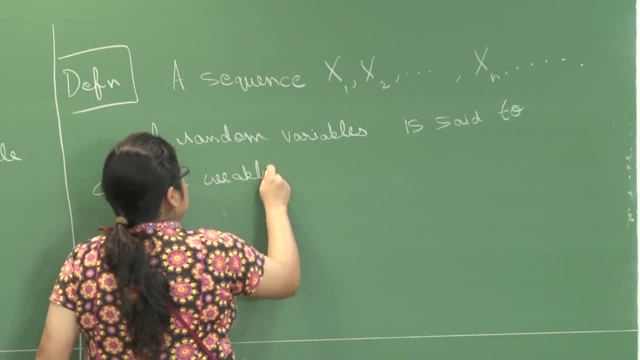 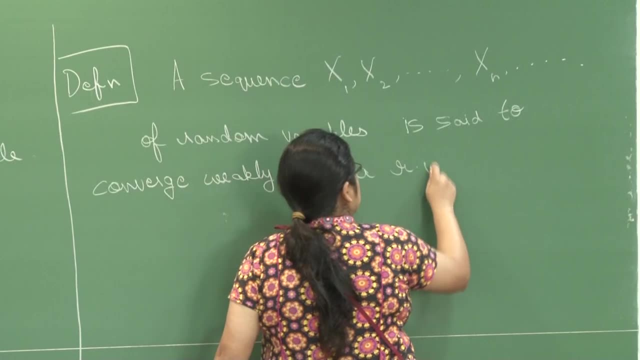 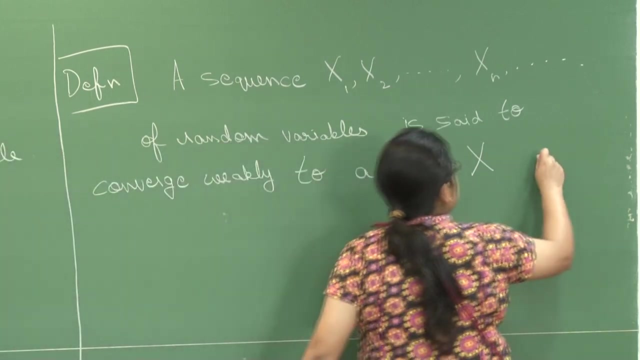 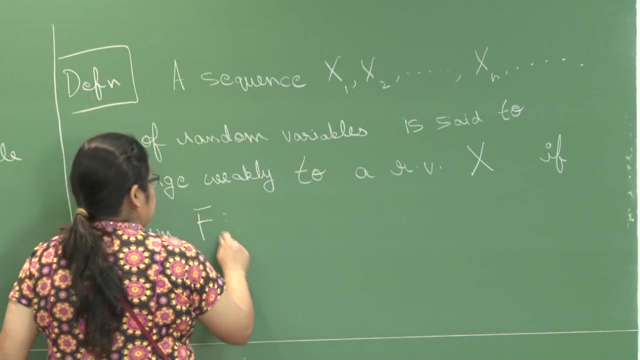 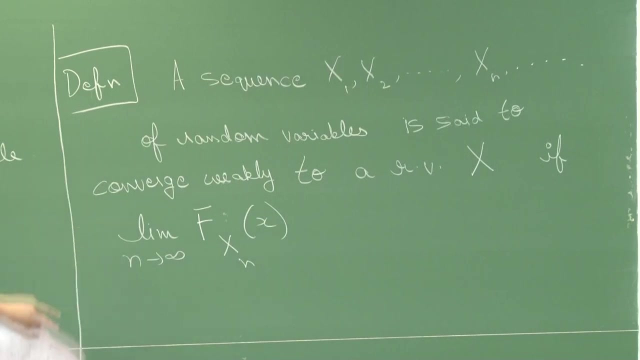 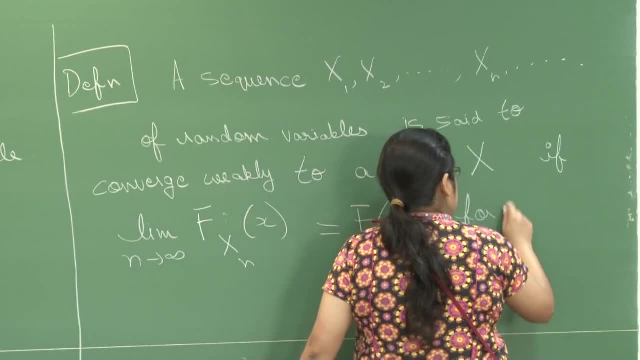 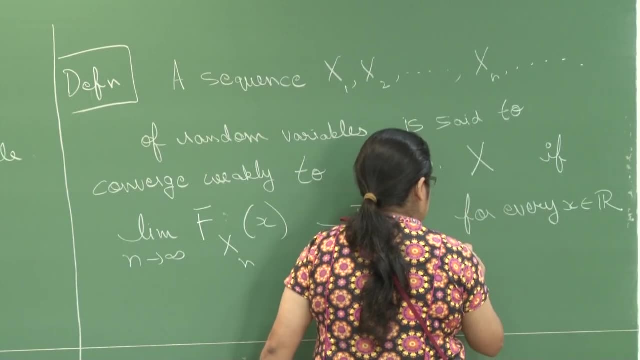 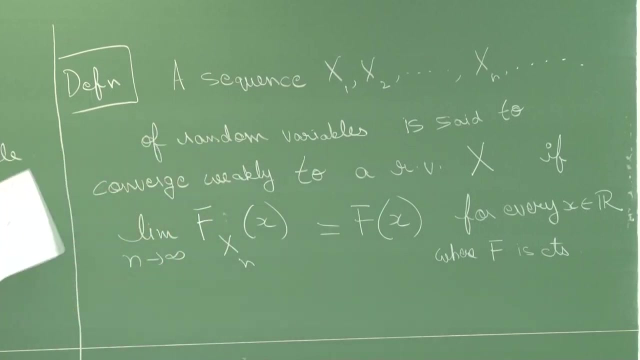 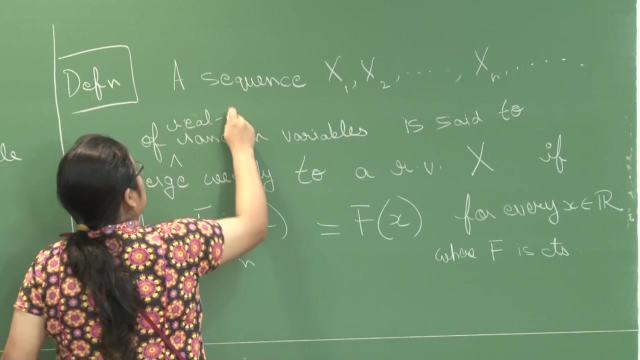 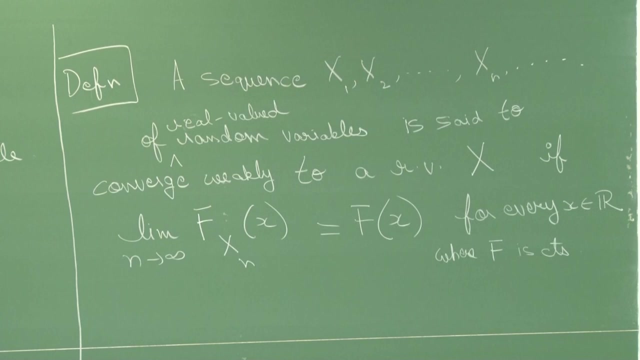 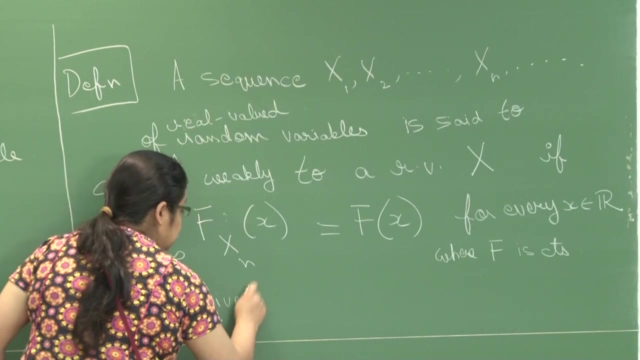 for every x in R where f is continuous, and let us take real value, random variables. So if this happens, then we say that our sequence x, n's converges to capital X. Alternatively, we may also say that the distribution corresponding distribution functions converge weakly to 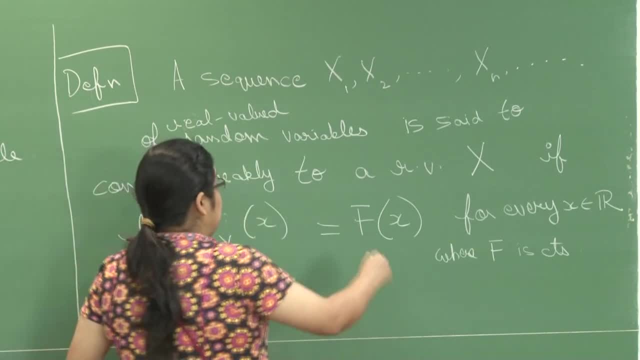 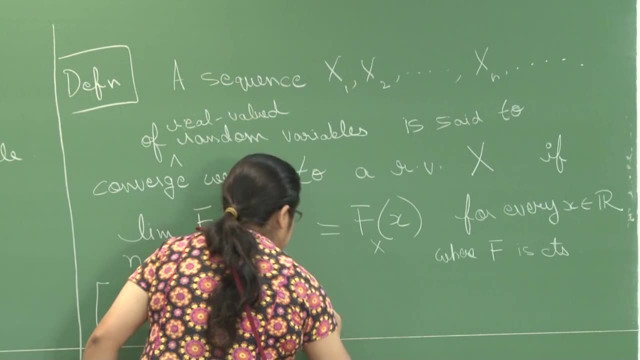 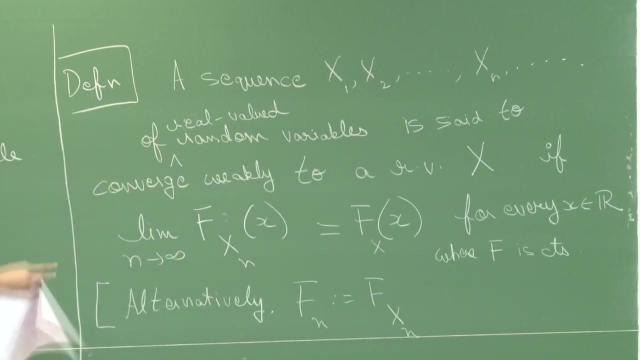 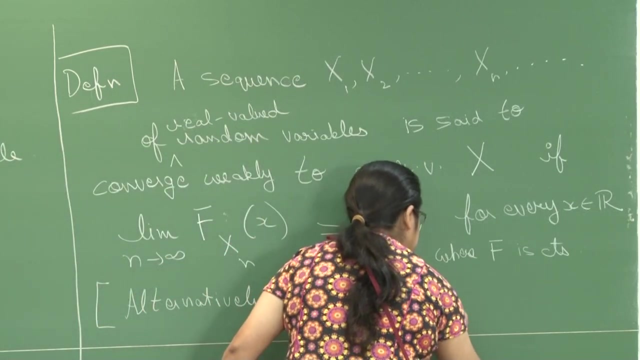 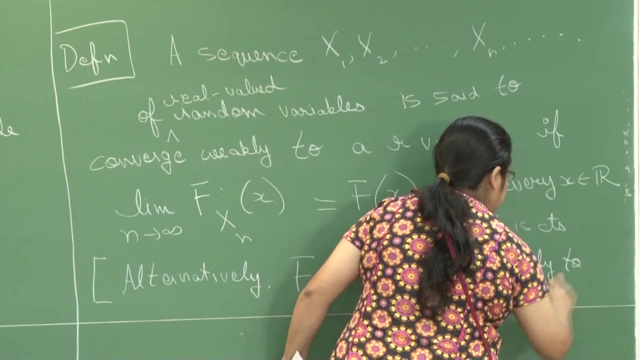 the distribution function of the random variable capital X. okay, So alternatively we have. so we define f sub n to be equal to the distribution function of capital X sub random variable capital X sub n. This we say that this converges weakly to f. There are: 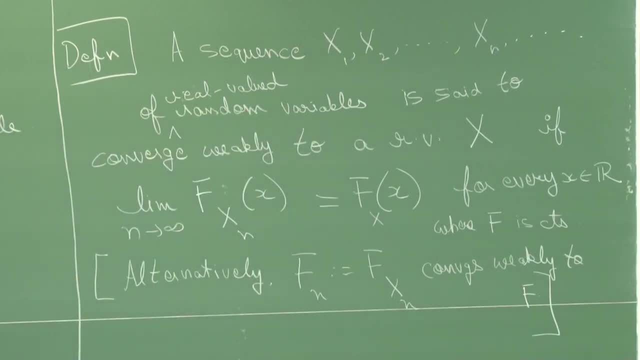 different types of notions Of convergence of random variables. we will be focusing on weak convergence Now. like I said, these random variables do not necessarily have to be defined on the same probability space and, as before, a very natural example comes from probability spaces defined with 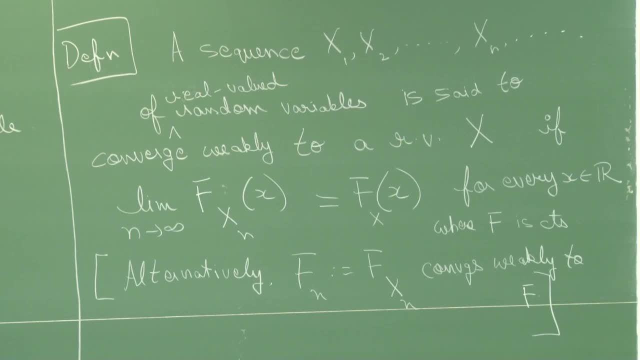 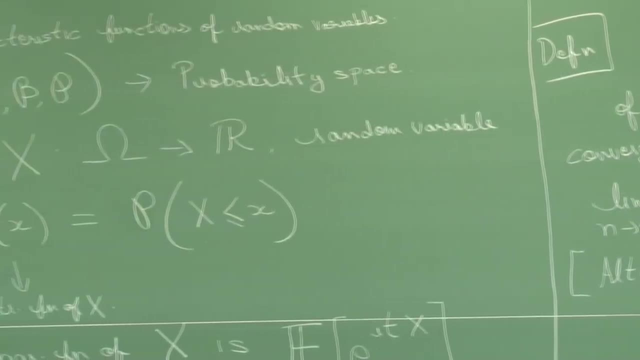 respect to finite subspaces. on sets, Let us take, say, similars. let us say, in the tree for fn, f sub n function. here we are doing some simple work for the f sub n on f sub n 관련 equations. Alright, now I am considering: 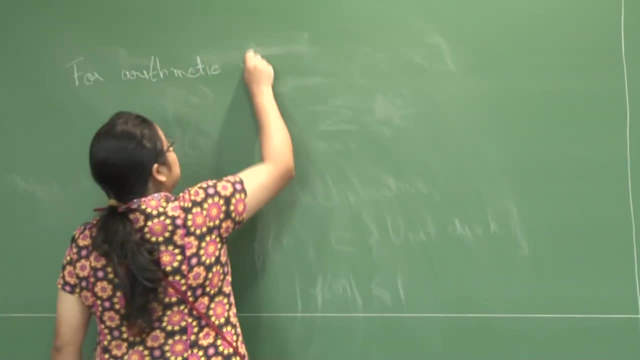 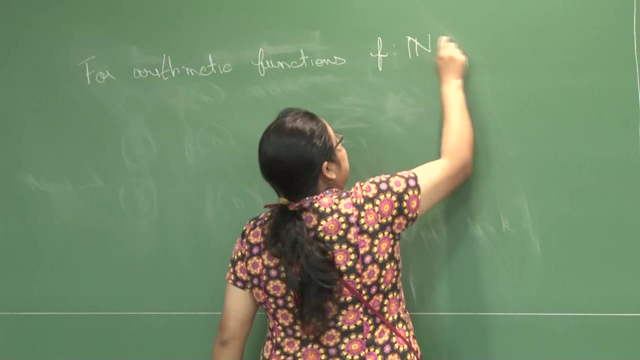 f sub n is classrooms of a large variance. So, for example, which isiu area of x f is actually quite large. Therefore, this is the Works on Mathematic narrations. form with a arms symbol R, and is the order in which the integral of values isцияucverts from f sub. 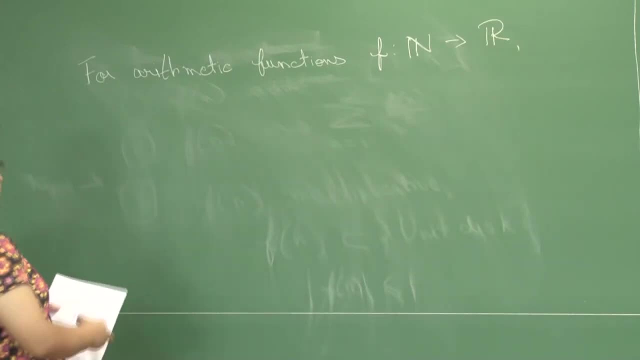 one r maximum and so on, And it is just a very simple rhetorical equation and we would also make the conclusion that f sub n, that suppose, would be equal to f sub n over x minus 4 minus k, plus f plus kd times 1 minus x, And you can blend into these квt. 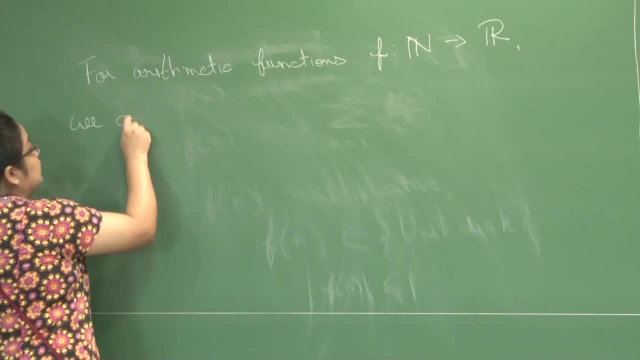 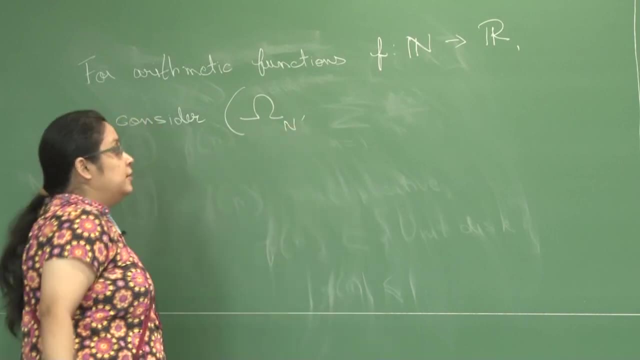 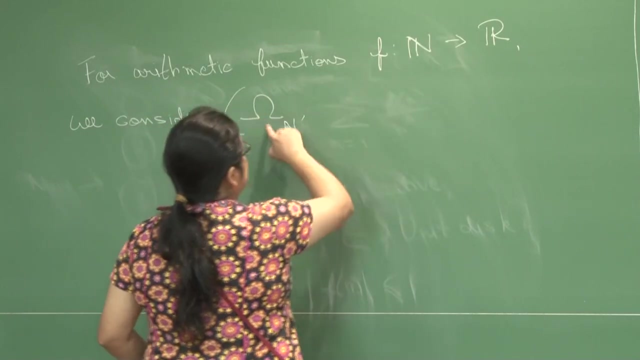 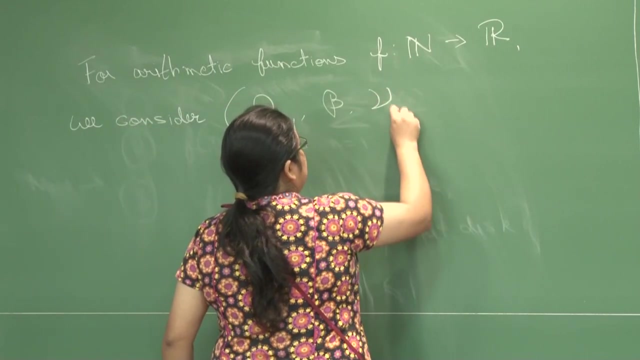 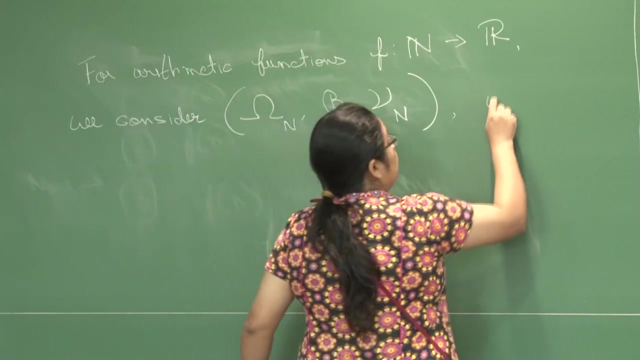 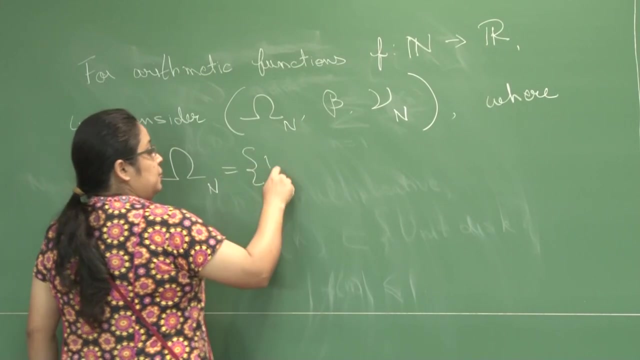 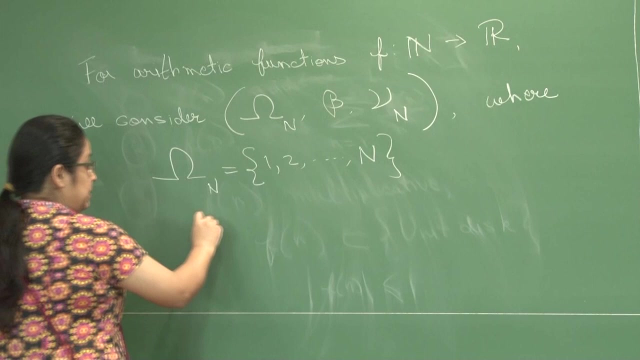 do is we consider the probability spaces omega sub n on- okay, so the set of all subsets of omega sub n, and on each such space we have the probability measure nu sub n where, as before, our omega sub n is just the set 1, 2 up till n- okay, and your nu sub n is defined. 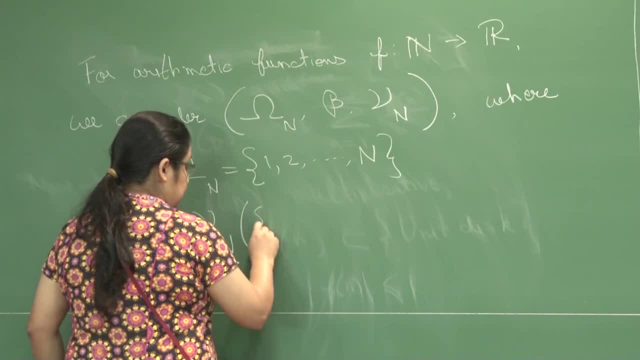 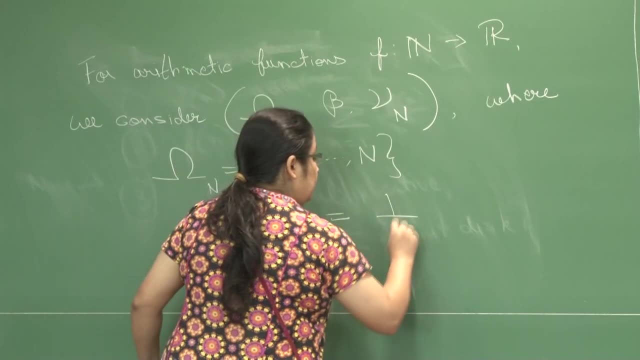 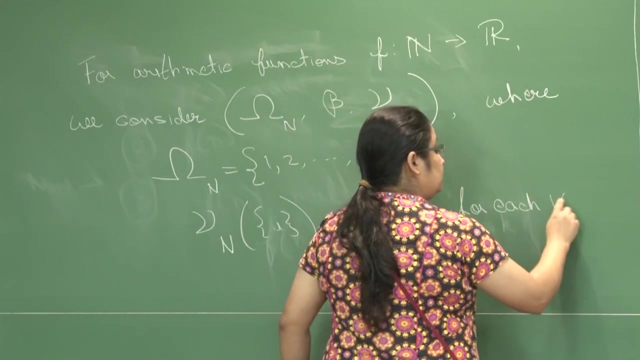 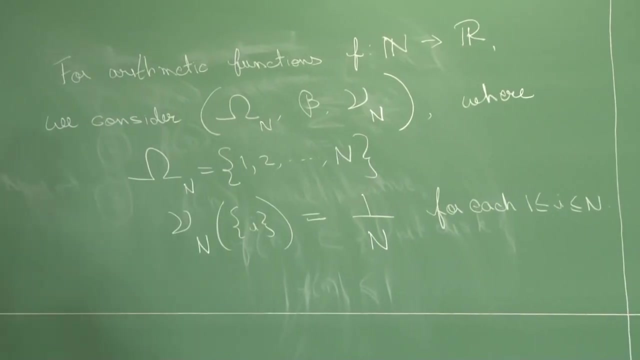 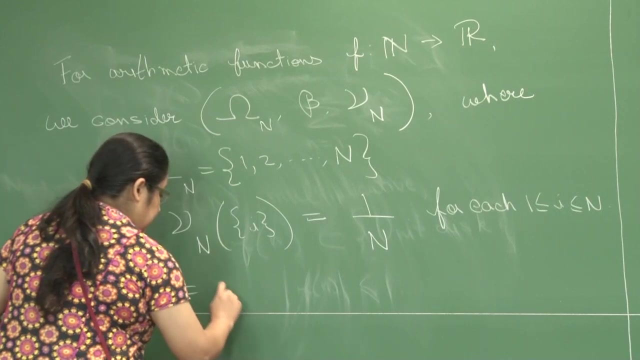 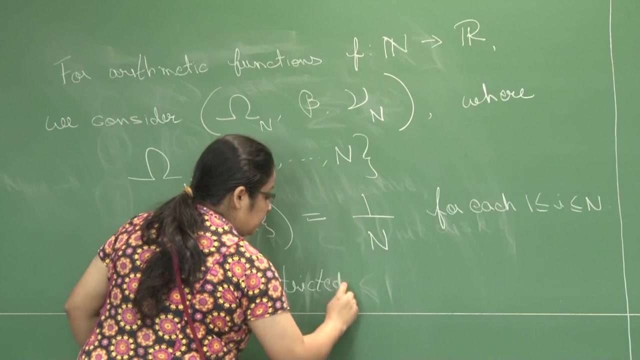 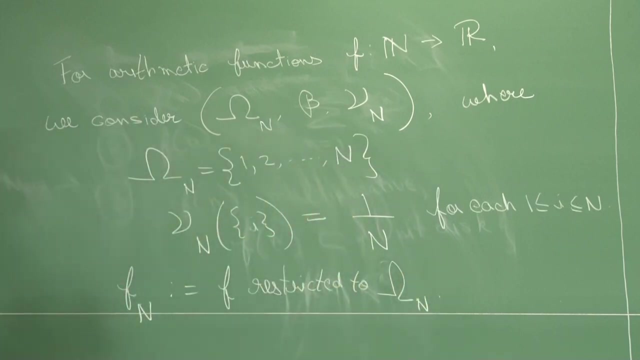 as follows: For any singleton i, it just takes the uniform probability 1 over n, and so our arithmetic function can be viewed as: so f sub n is just f sub n. Okay, F restricted to omega sub n. and so this is how we learnt to view arithmetic functions. 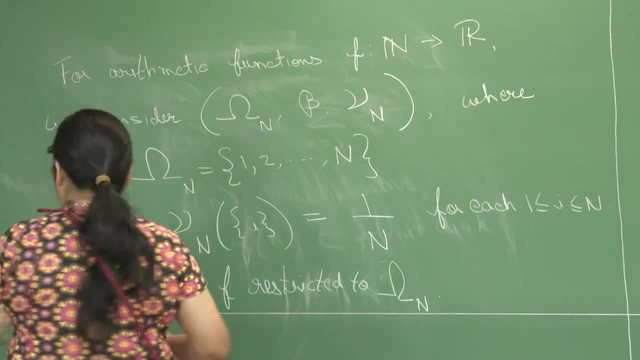 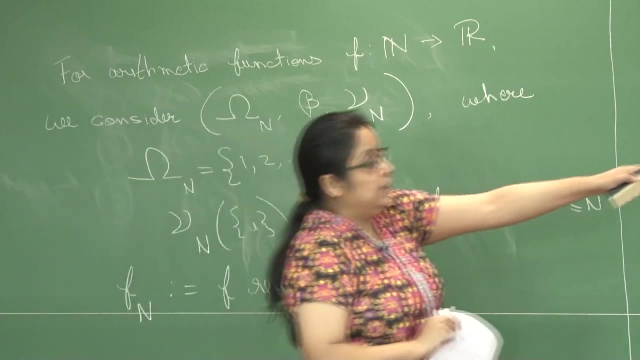 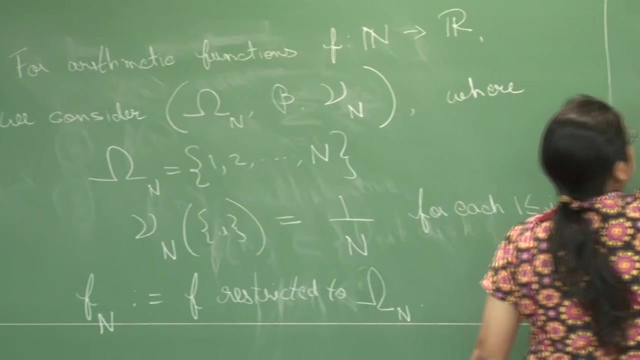 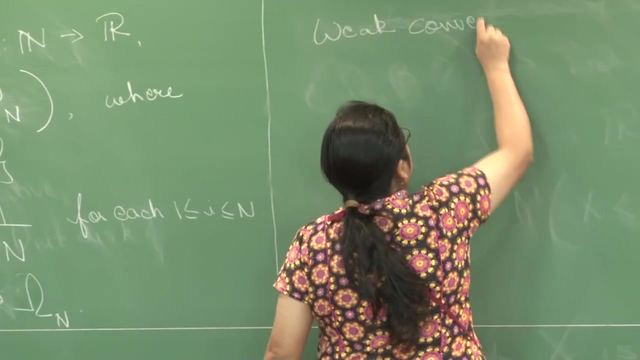 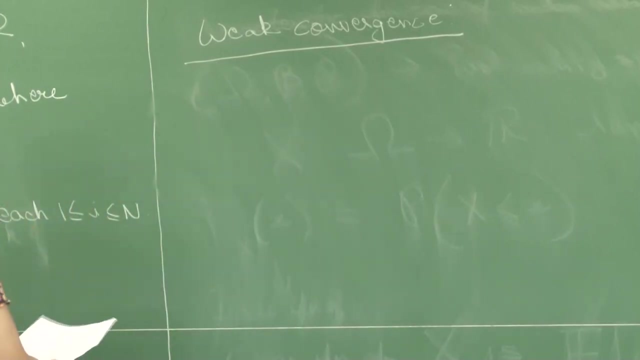 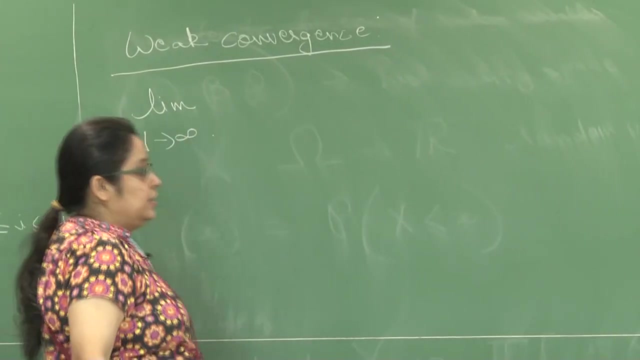 as random variables. This is a brief review, in case you forgot, since we are meeting after a long time. So, with this in place, what does weak convergence refer to? So we say that, so we have. so what does weak convergence here mean? okay, So we have limit as n goes to infinity. okay, of this distribution function here, which is: 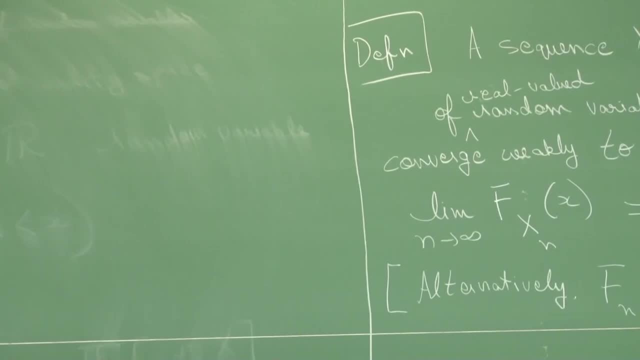 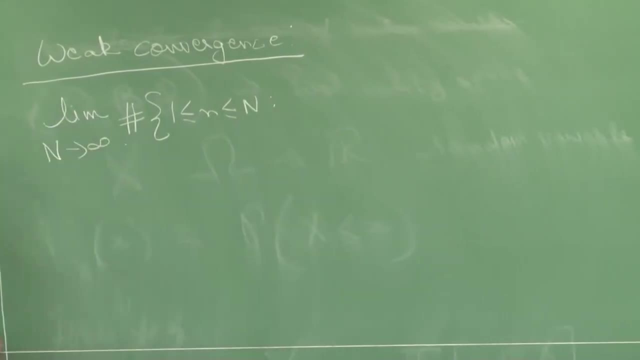 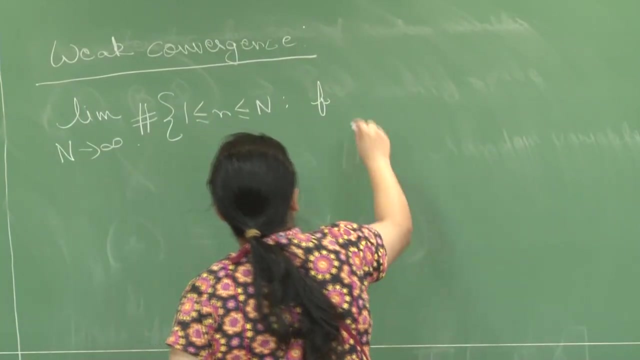 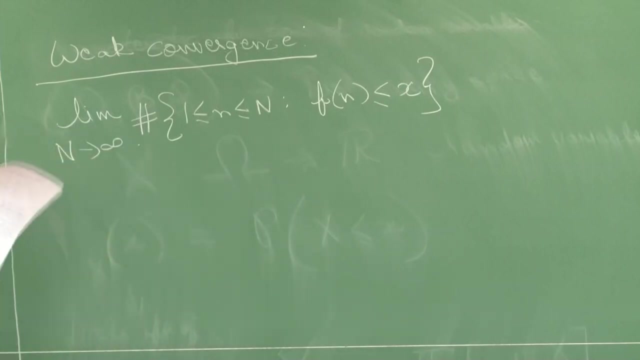 what do you have? We have this: this is just the number of natural numbers up to capital N, for which f of n is less than or equal to x. okay, The question is whether this converges to f sub n. Okay, So what do you have? 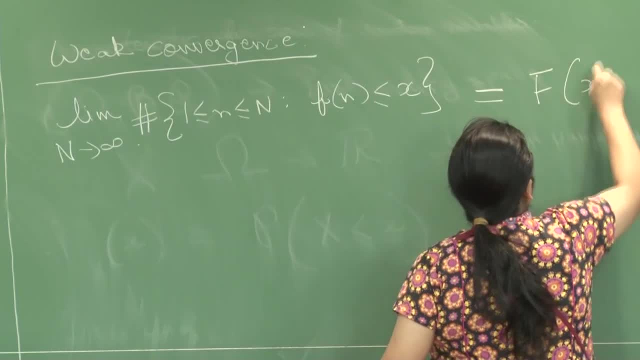 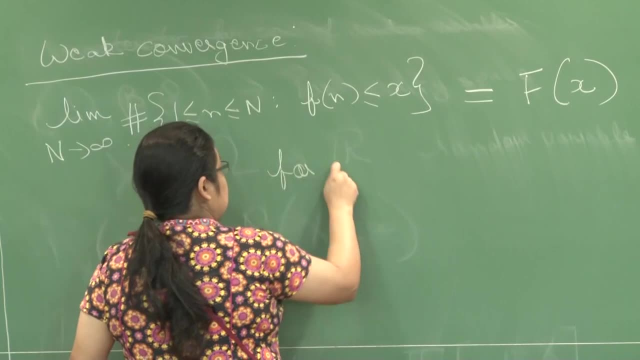 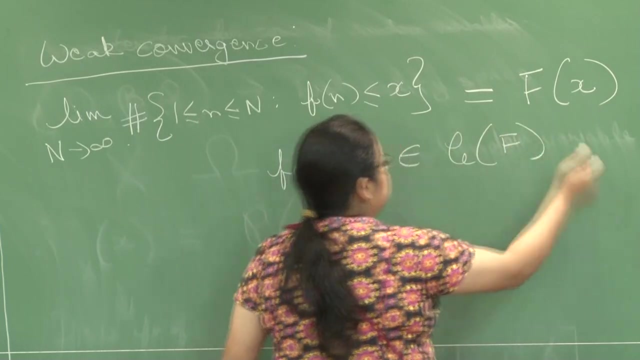 We have this: this is just the number of natural numbers up to capital N, for which f of n is less than or equal to x. okay, And if we have some function, some capital F of x for all x lying in the set of points at which your function f is continuous? 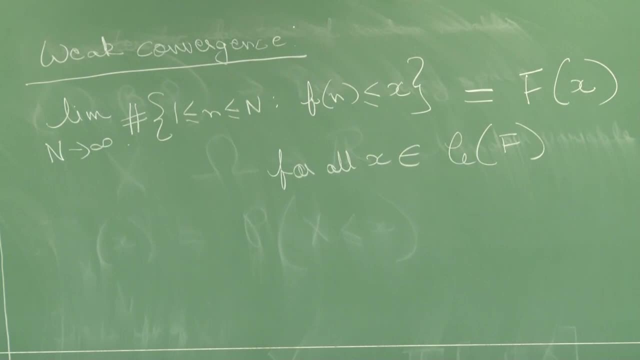 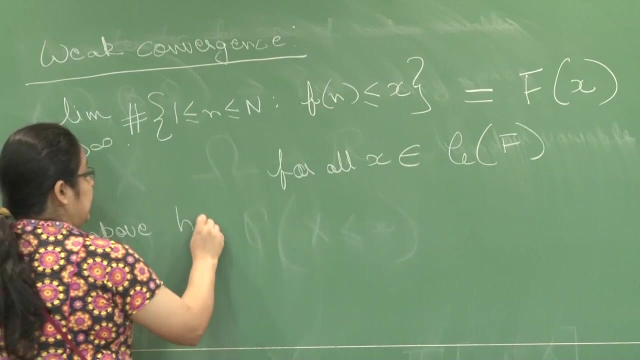 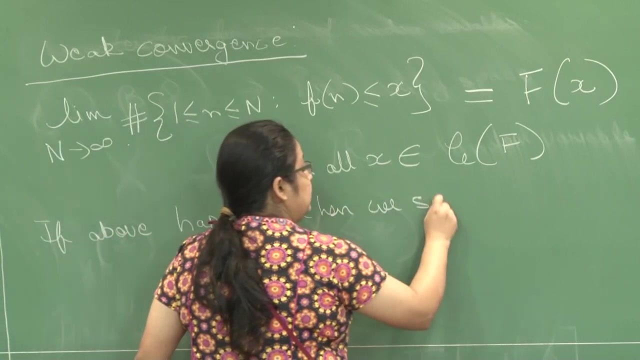 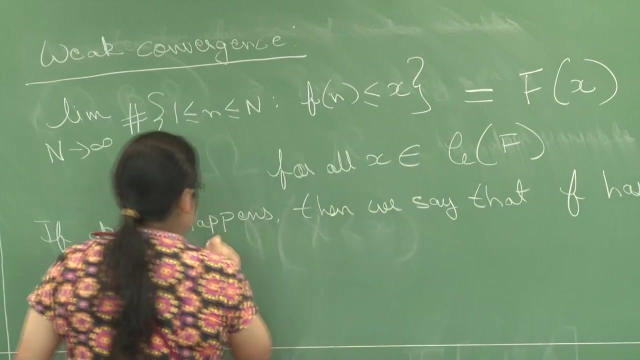 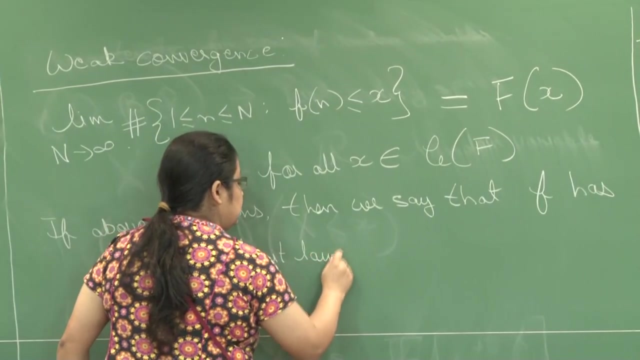 Okay, If this happens, then we say that there is a weak convergence of these random variables to capital F. Another short form of saying This is: If the above happens for some capital F, suitable capital F, then we say that F has a limit law. 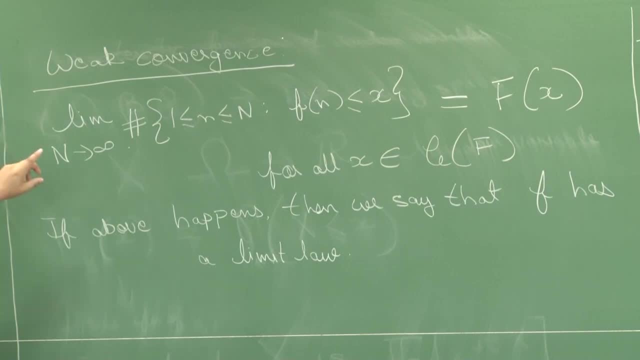 And now what we do is we recall a very important theorem from probability, which I am just going to state without proof, which is which relates the notion of weak convergence to the characteristic functions of our random variables that we are looking at. So this is an important theorem and this gives us the motivation for looking at multiplicative. 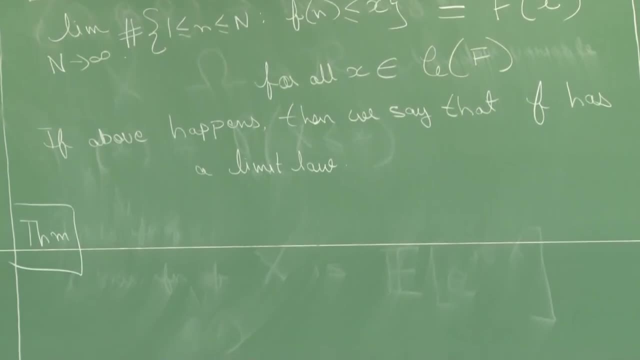 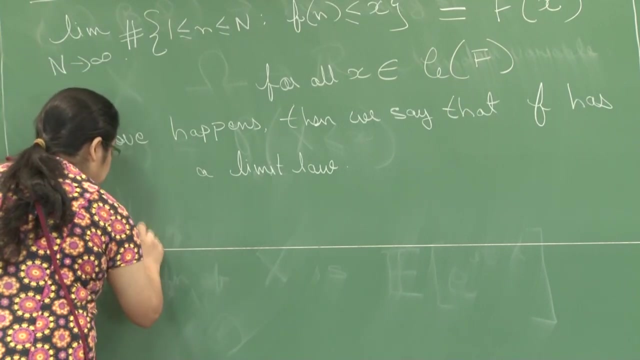 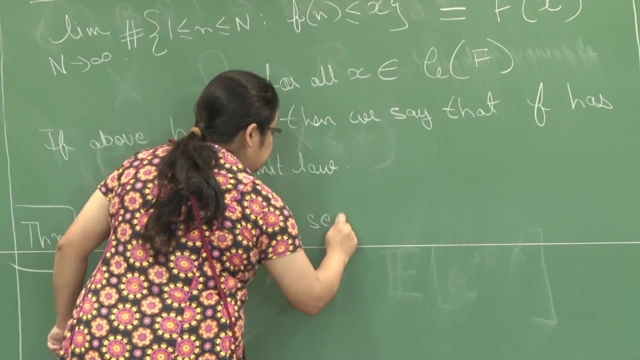 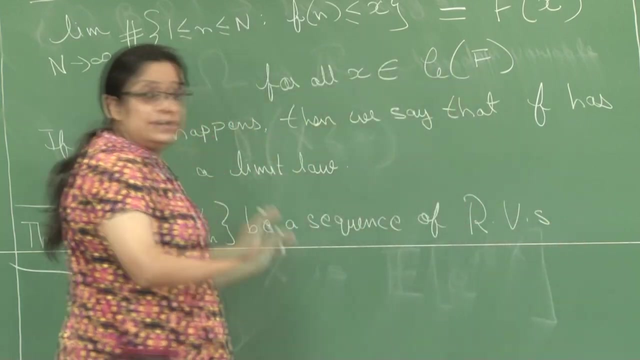 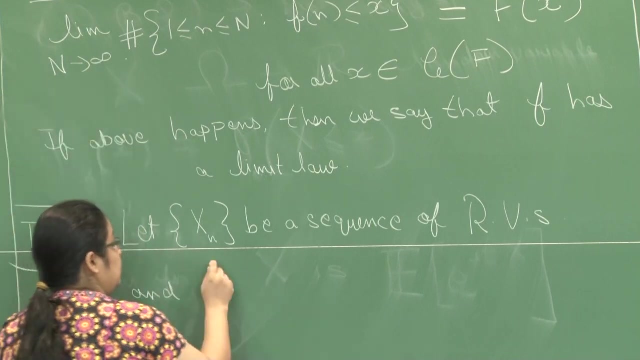 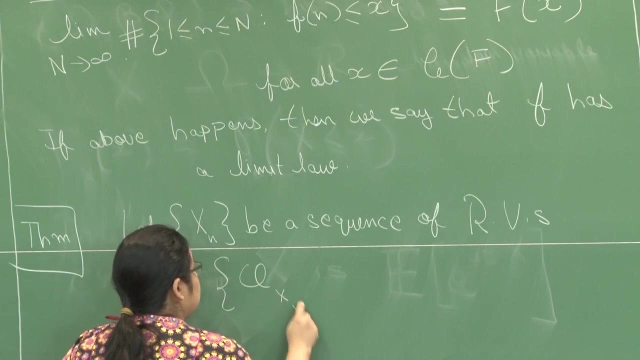 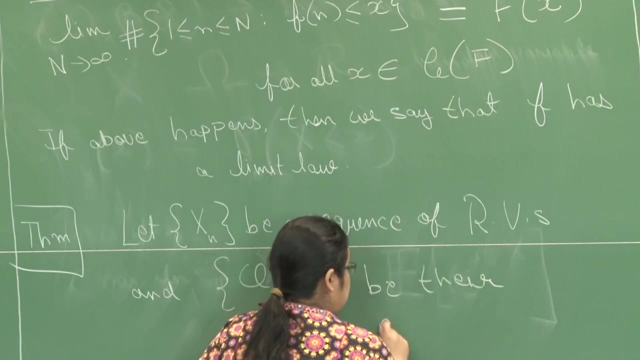 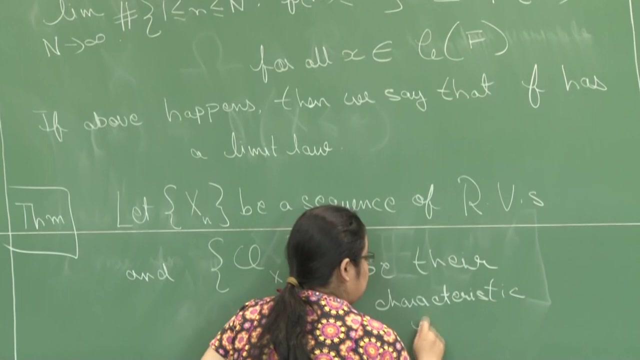 functions which, whose values lie inside the unit circle, inside or on the unit circle. So let us take, as before, a sequence of random variables, not necessarily on the same probability space, and let us take, Let us say, phi, X, sub, n, be their characteristic functions. 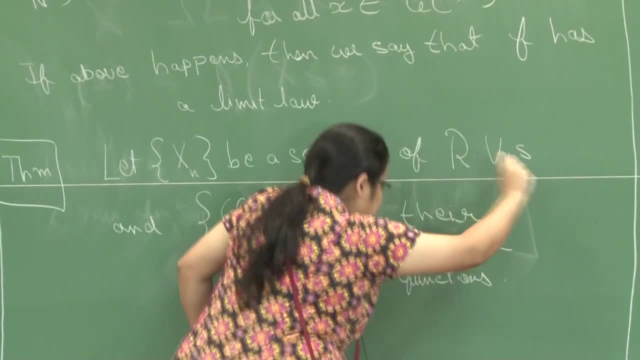 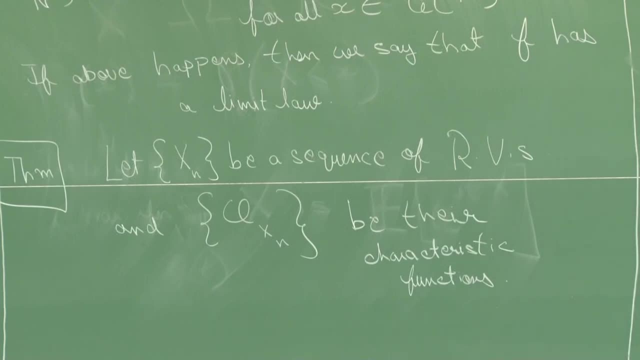 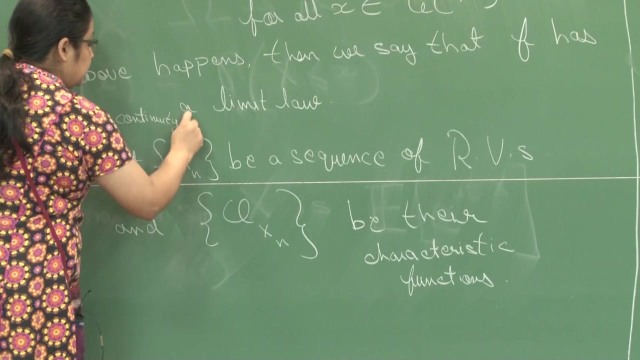 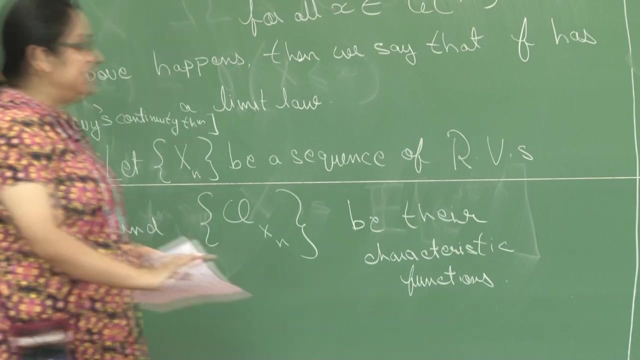 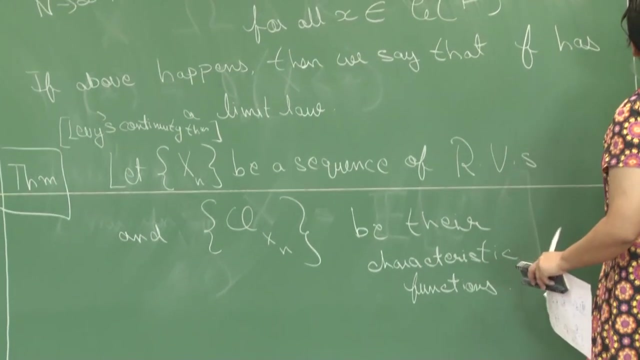 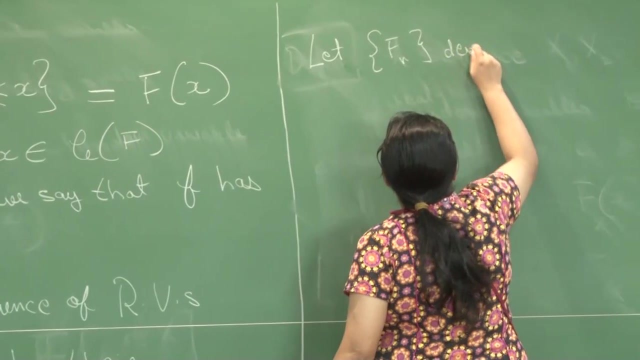 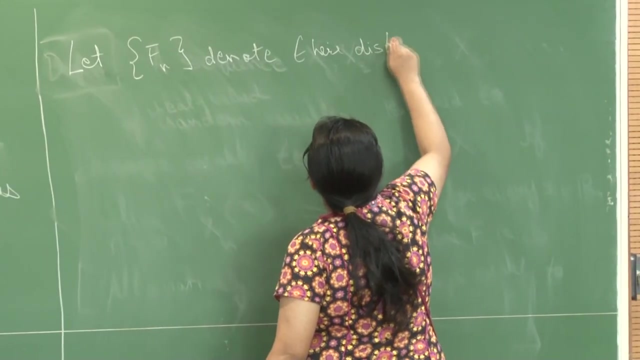 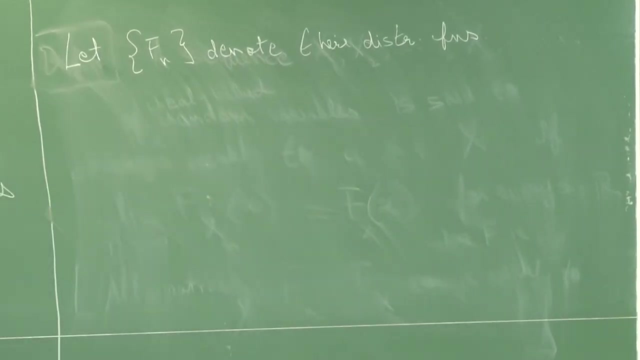 Okay, So this theorem, which is? it, tells us that. so this is called Levi's Continuity Theorem. okay, so I think the correct pronunciation is Levi's. I will confirm before the next class. So suppose you have this. so let F sub n denote the distribution functions, then our: 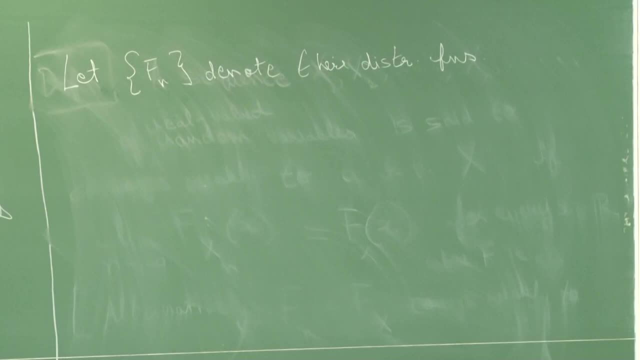 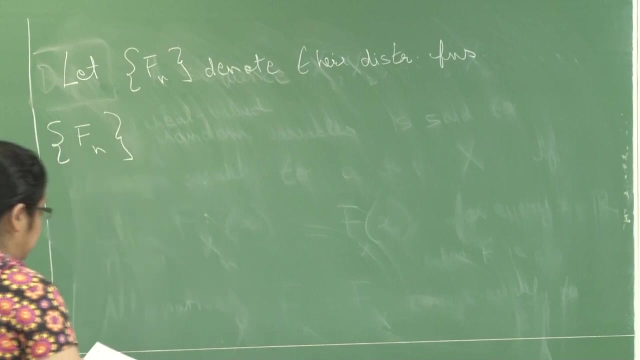 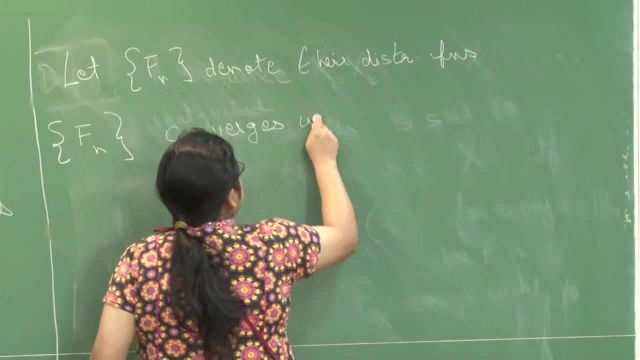 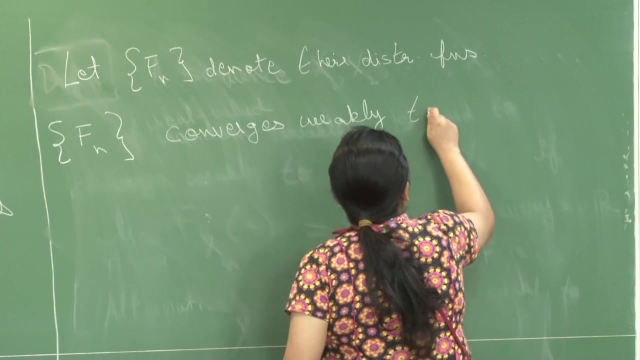 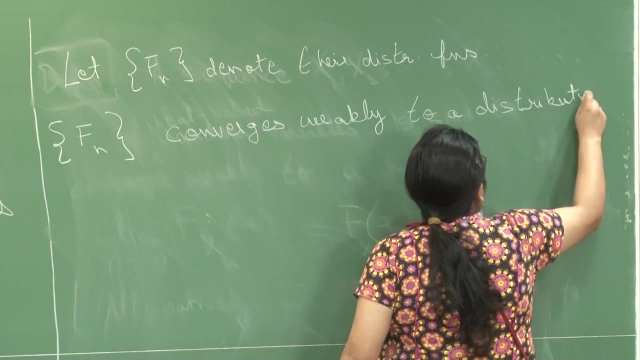 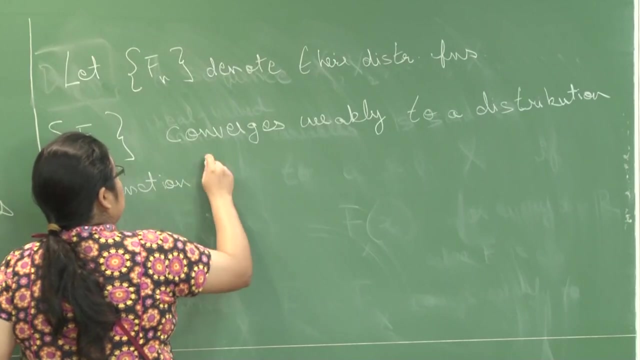 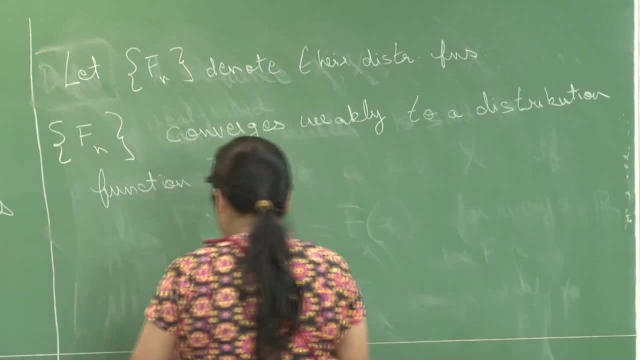 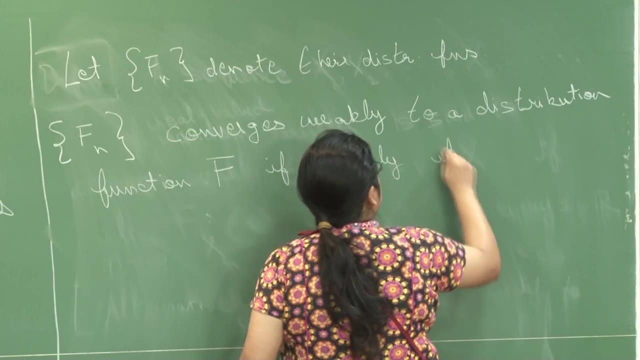 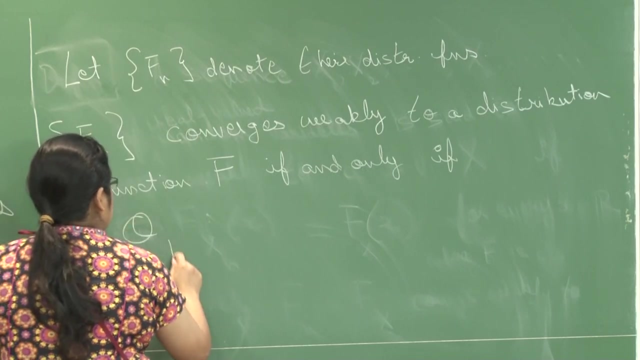 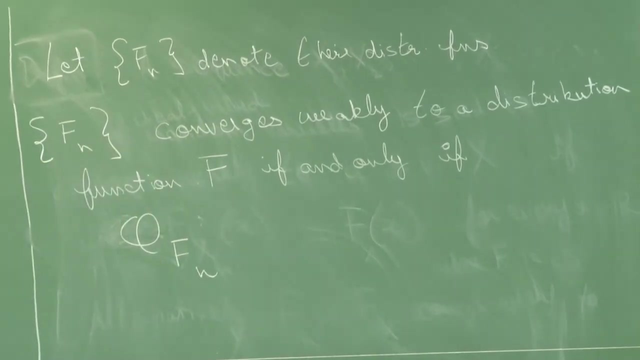 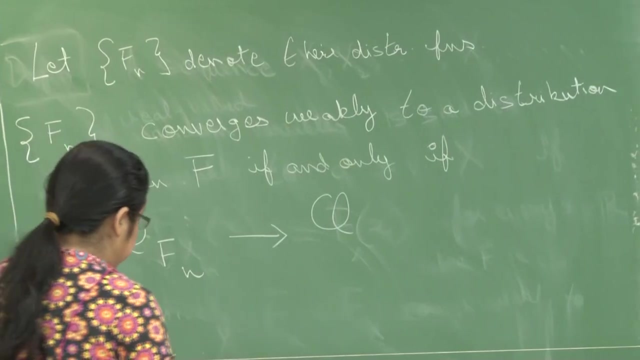 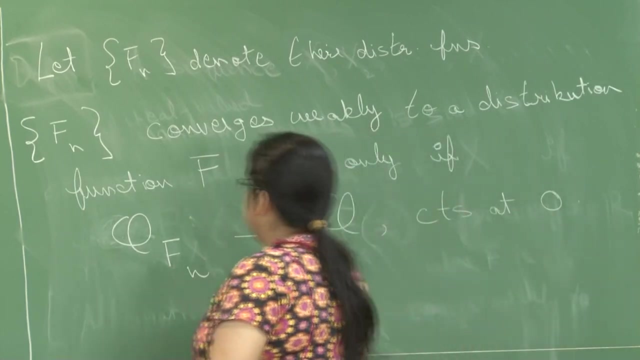 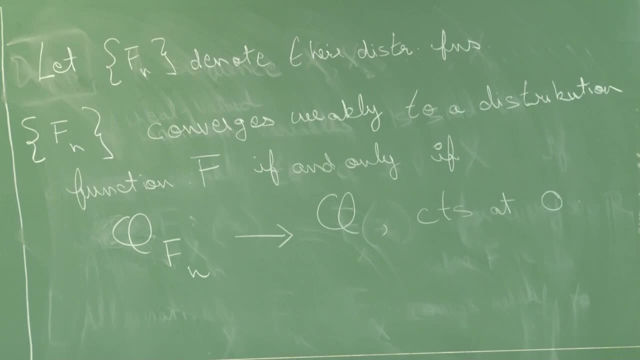 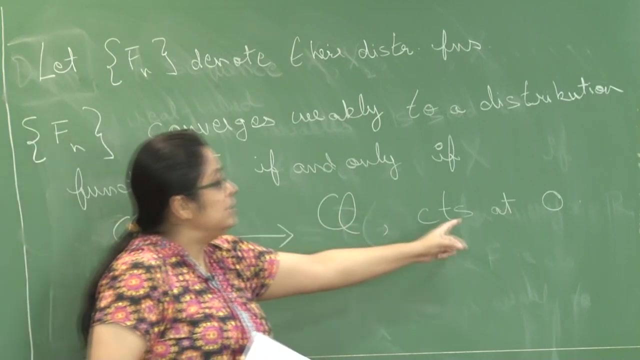 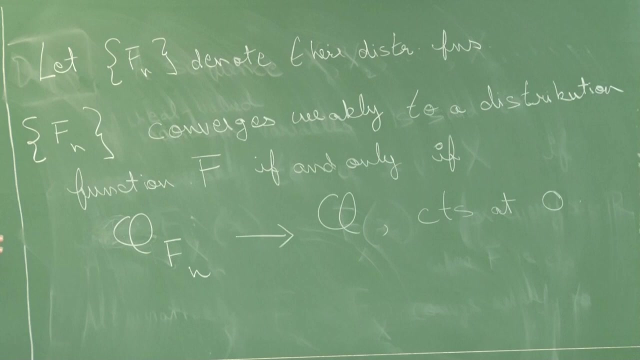 of distribution functions f sub n converges weakly to a distribution function, f is equivalent to saying that their corresponding characteristic functions converge to a function, some function which is continuous at the point 0. So in order to study weak convergence, we can translate the study into the convergence of our characteristic functions. So this is where the motivation. 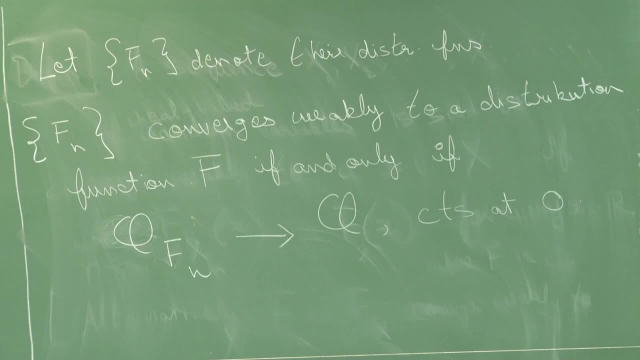 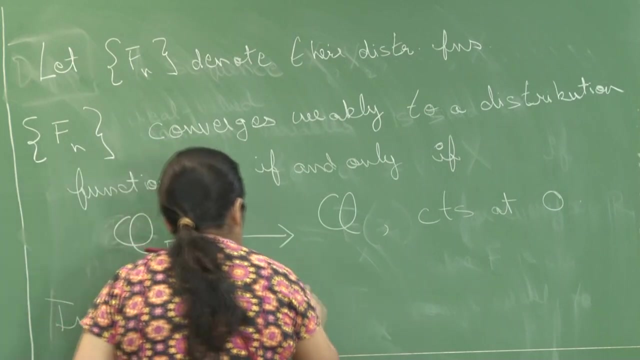 comes from. and now, if this happens, okay. So if you have your characteristic functions converging to some suitable function which is continuous at the point 0, then in this case, this function phi, is significant in the sense that it is turns out to be the characteristic 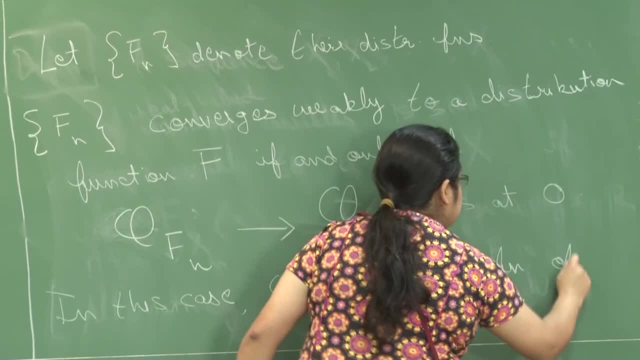 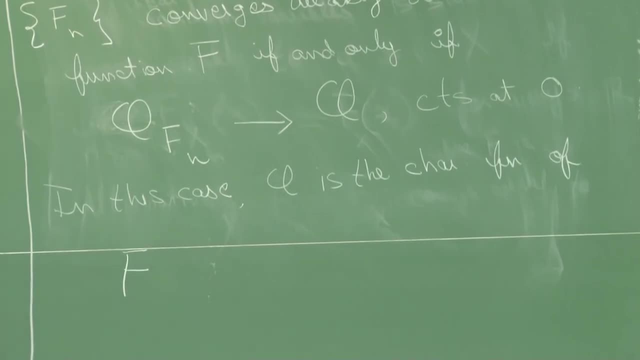 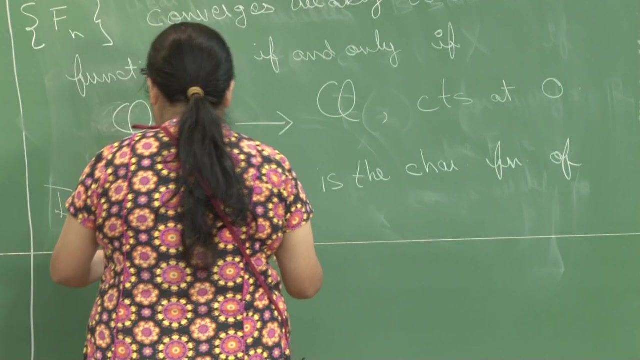 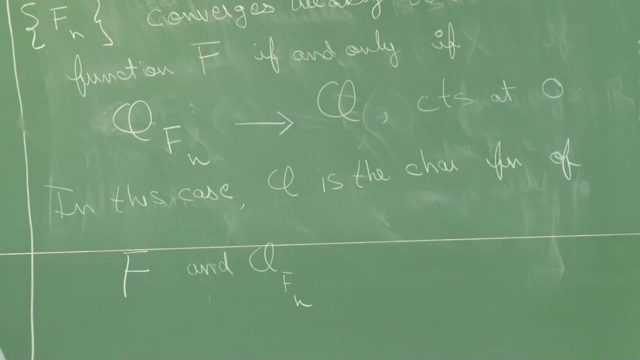 function of capital: F. Okay. so to say that f n converges to f is equivalent to saying that phi f n converges to phi f and your phi sub f sub n- okay. So if you have that phi sub f sub n is converging. 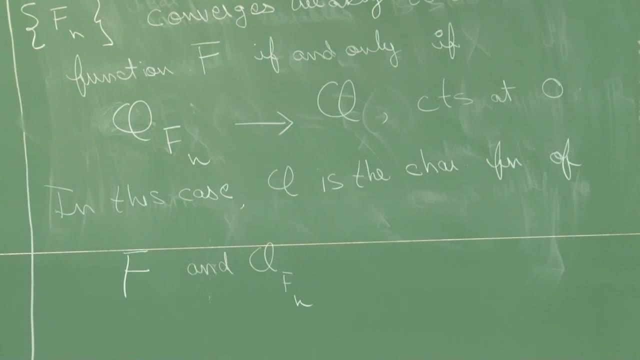 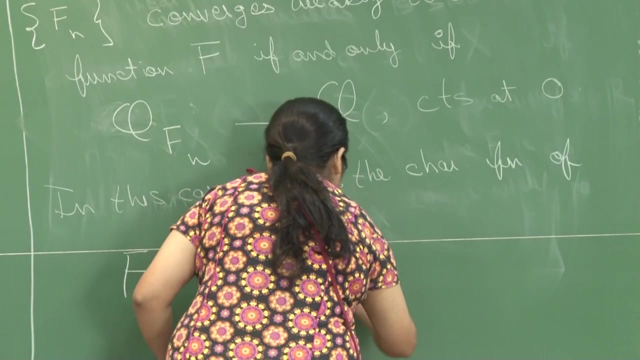 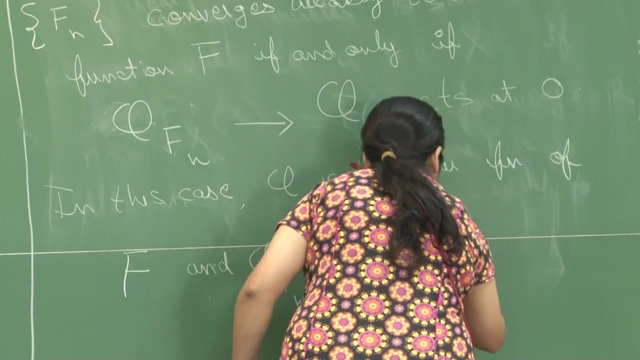 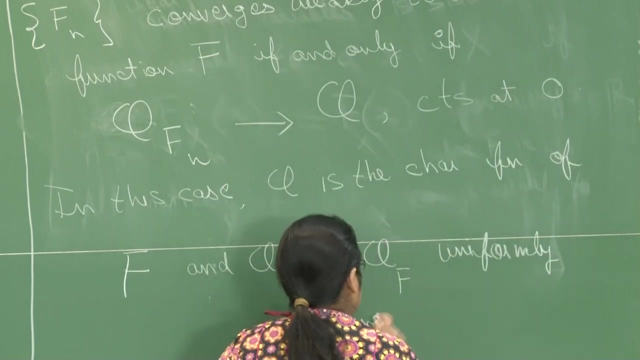 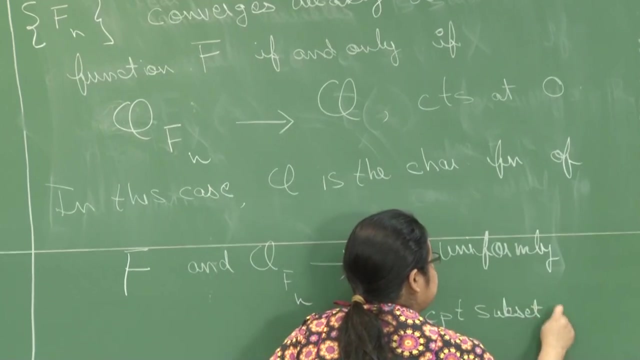 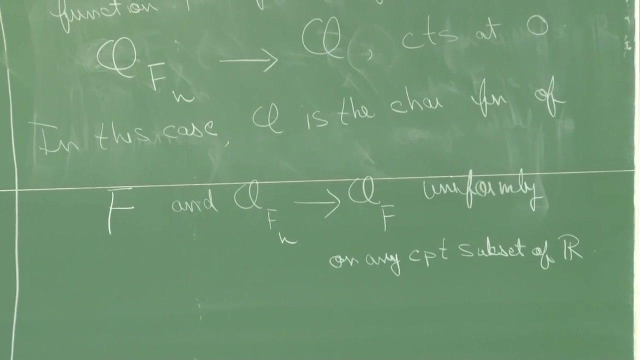 to phi, which is continuous at 0,, then this convergence is in fact uniform in any compact subset. Okay, So this convergence of phi sub f, sub n to phi sub f is uniformly convergent. This convergence is uniform on any compact subset of R. alright, Now, in the context of the 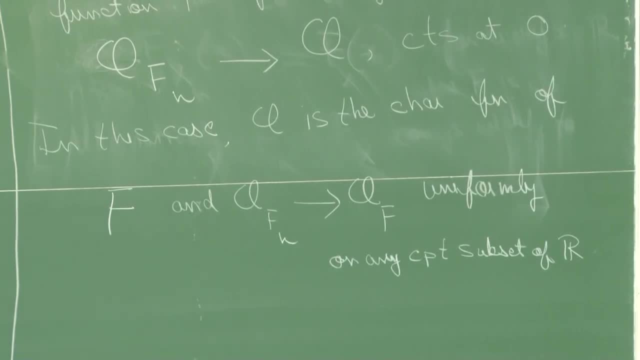 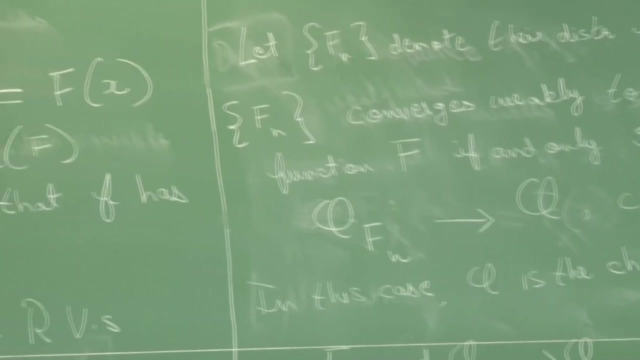 arithmetic functions we are looking at. if we wanted to apply our continuity theorem to that context, then what we have to study is the characteristic function. So you have some function f, okay. So what you need to do is you need to study the expected value. 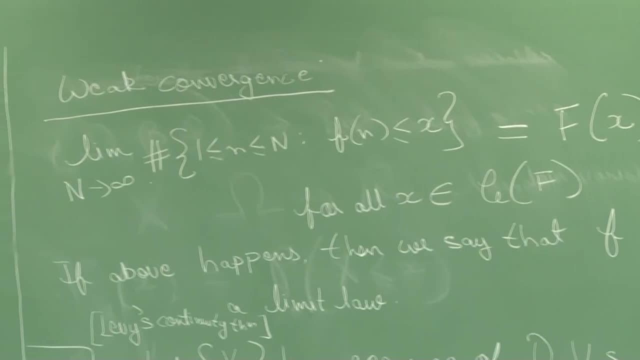 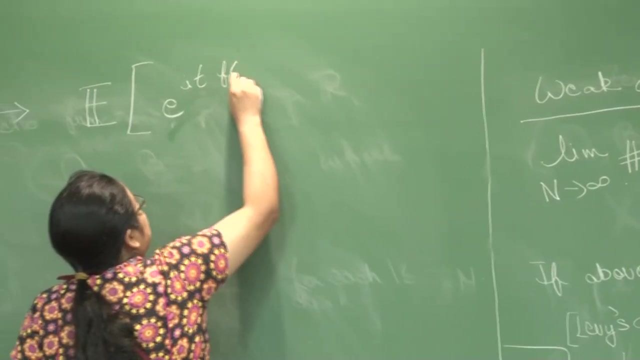 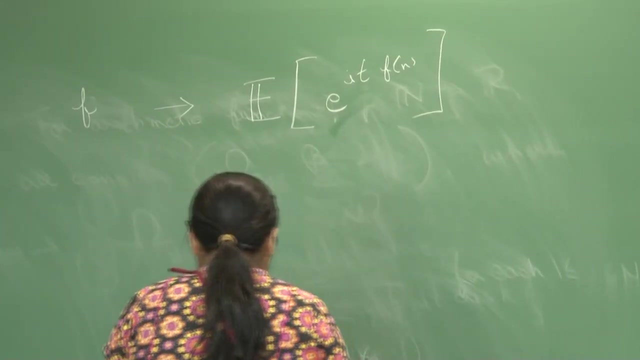 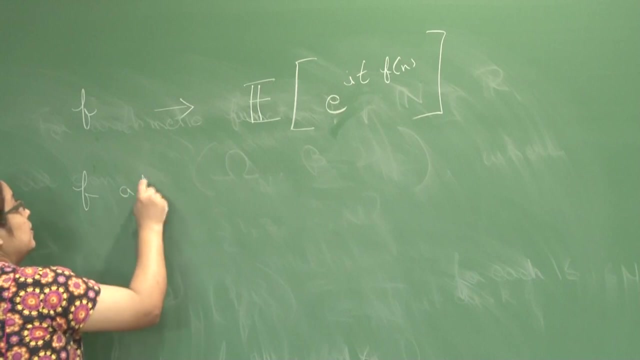 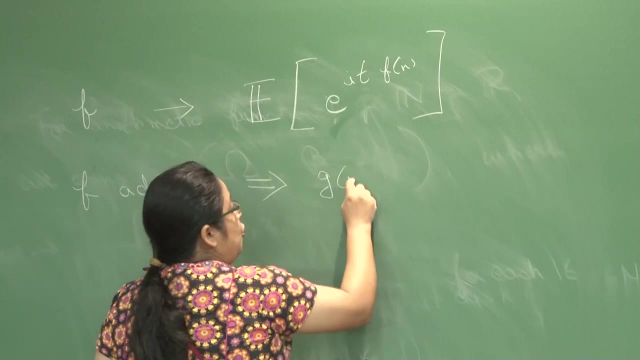 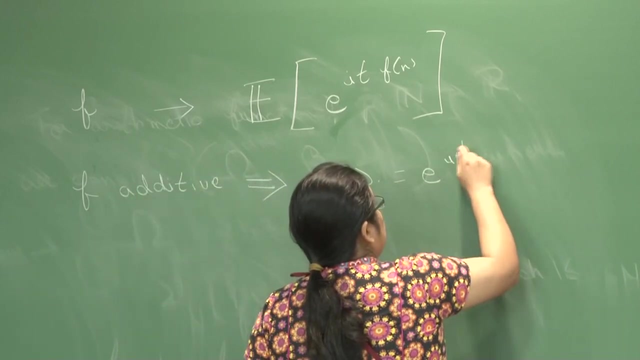 of f as a function, Okay, Okay, Okay. of e raised to the i t f of n. right, And notice so if you have. if f is additive, it implies that the function g of n, which you define as e, raised to the i t f of n, where t is any real number, okay. 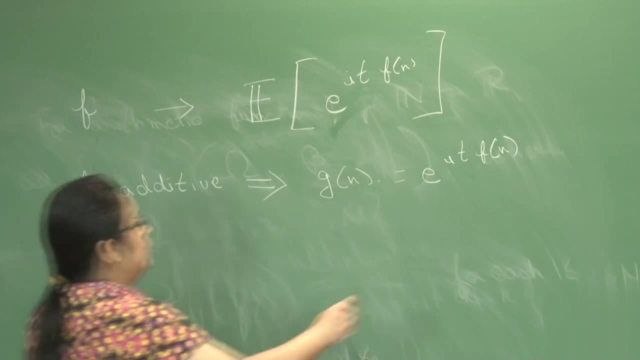 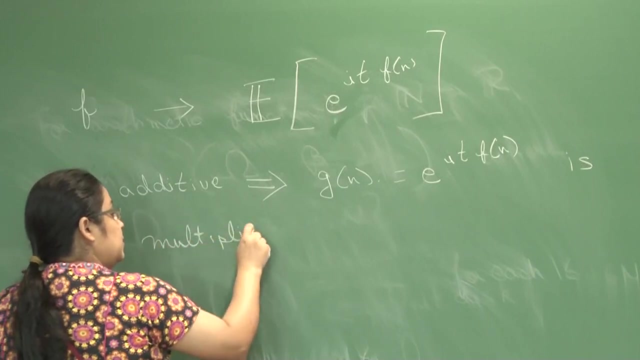 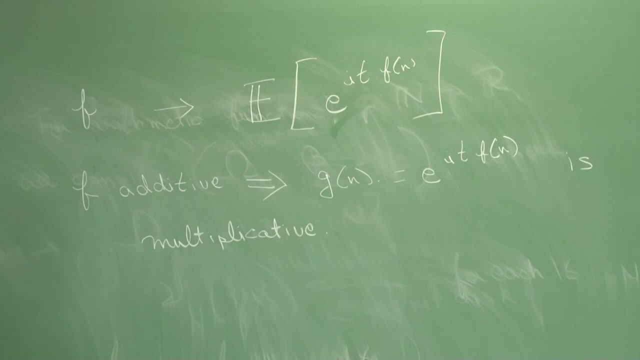 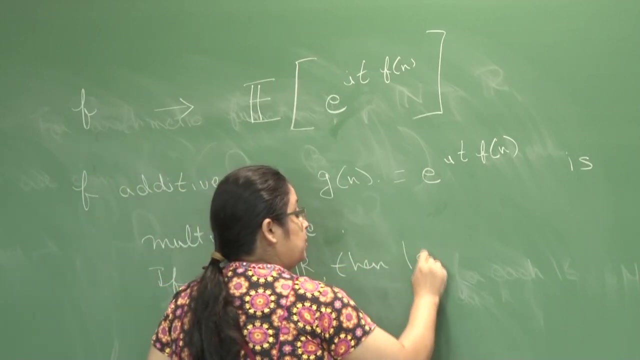 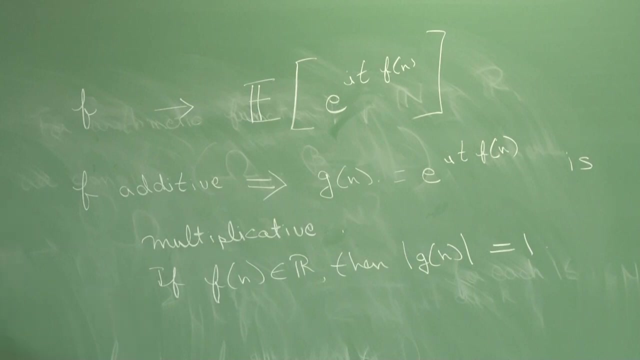 This function will turn out to be multiplicative. And if your function f is taking values on the real line, then clearly i t f of n is absolute, is exactly equal to 1, right? So that is why we want to study functions which are multiplicative. average order. 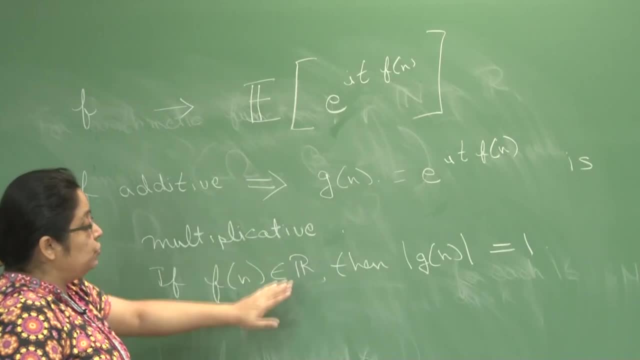 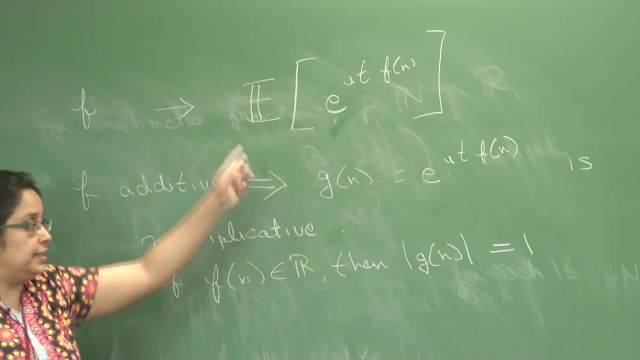 So expected values are average orders. So we want to study The average orders of functions which are multiplicative and whose values lie, in this context, exactly on the unit circle. But we generalize this a little bit and address those functions which are multiplicative. 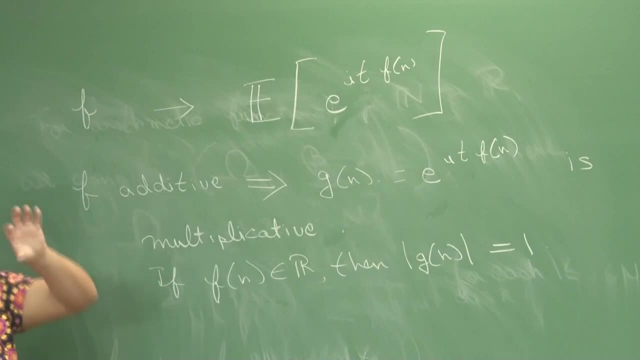 but which take values not only on the unit circle but also inside the unit circle. So this leads to a set of very beautiful theorems, and we are going to initiate the study today. Okay, Okay, Okay, Okay. So the first theorem in this context is DeLange's theorem, which states the following: 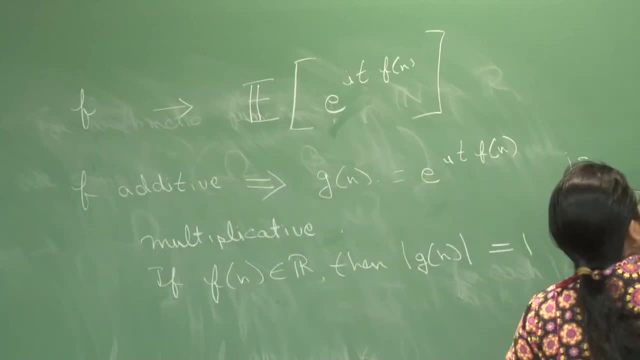 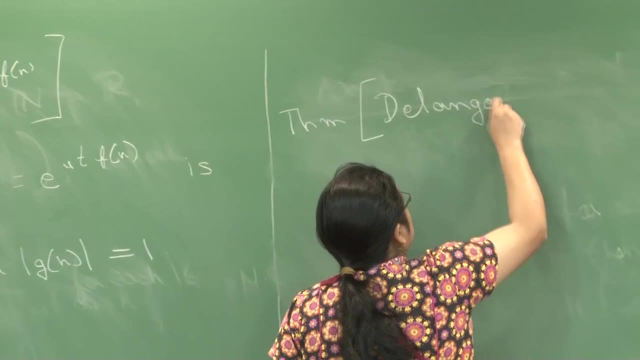 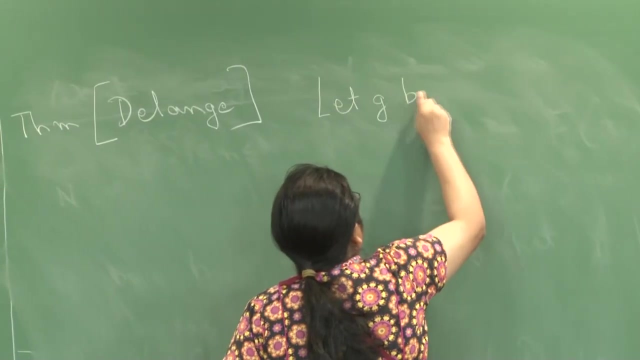 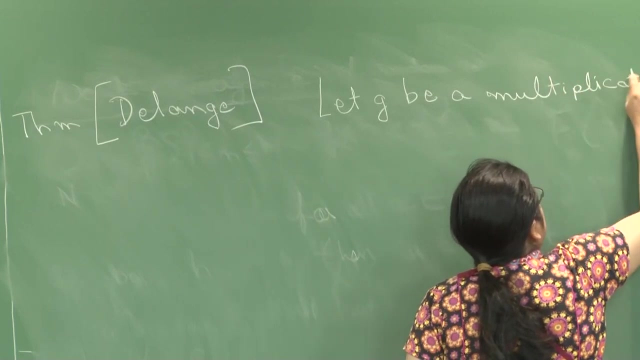 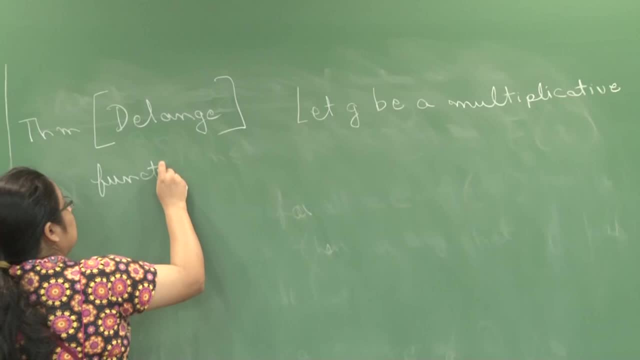 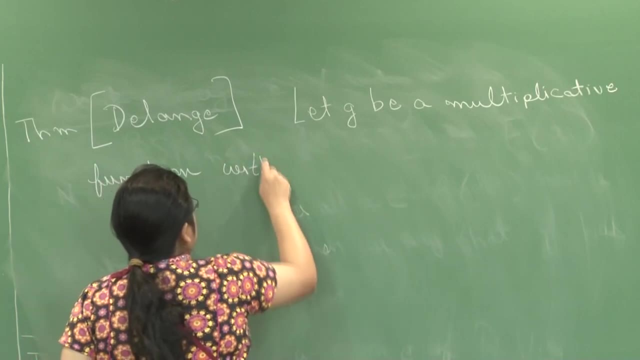 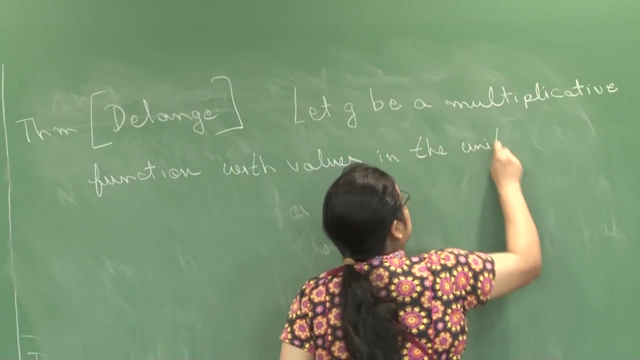 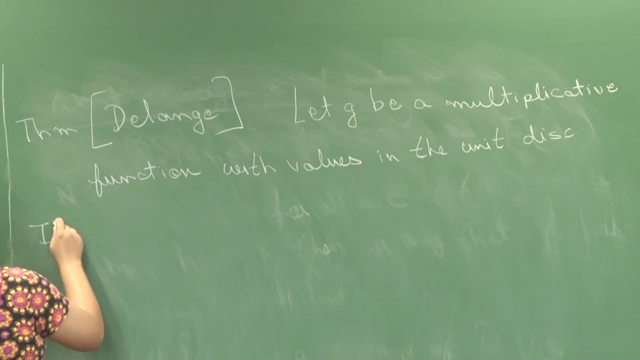 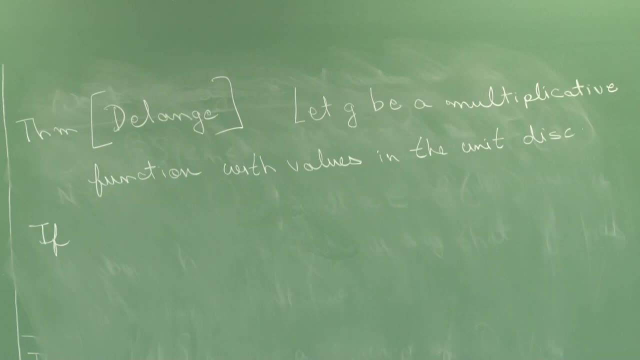 be with the help of the notion of Euler product. they can be studied in terms of their values at primes and prime powers and, continuing in that direction, it would be enough for us to prove a theorem or prove a condition for G with respect to its values at prime numbers. 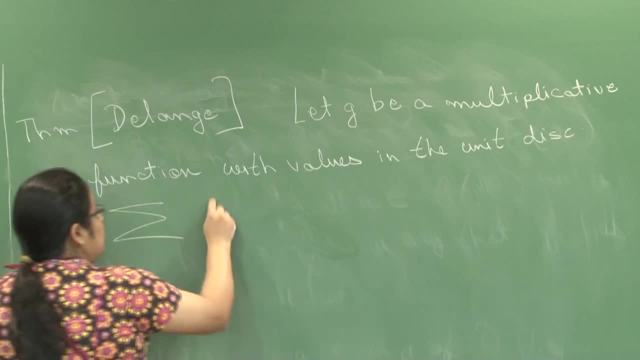 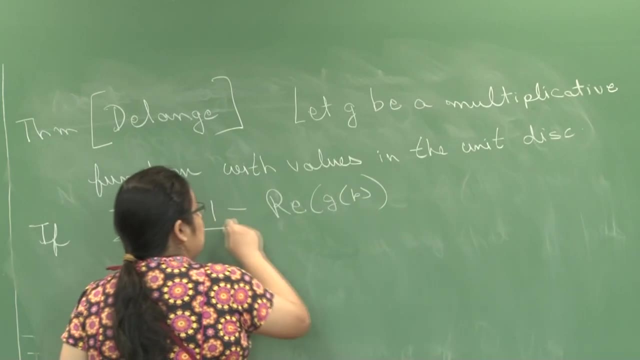 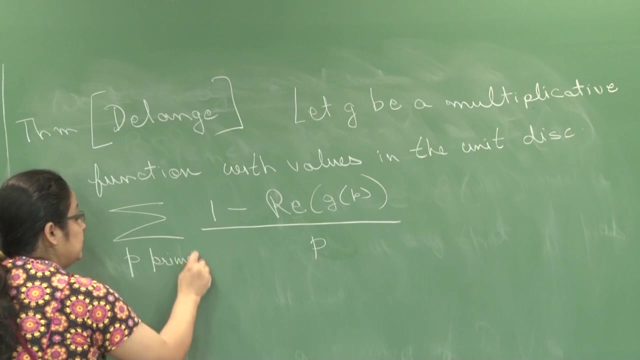 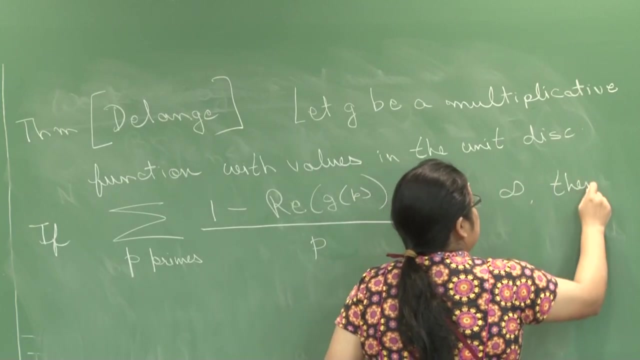 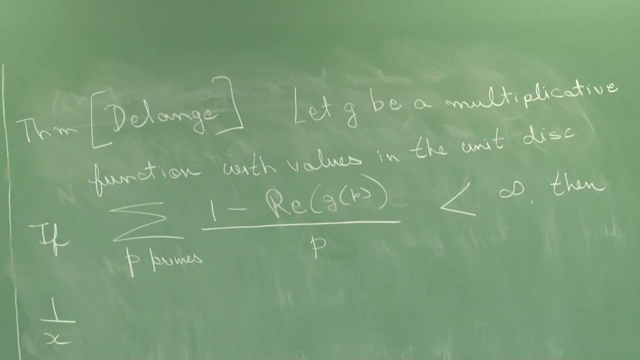 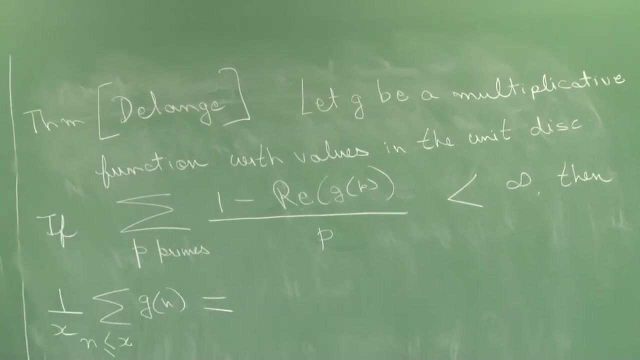 So if the following happens: if the sum 1 minus the real part of G of p over p, as the sum runs over all the primes, If this is finite, Then the average order of our function G of n is equal to the following product: 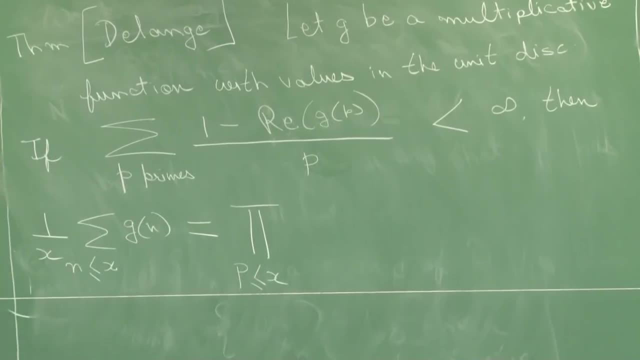 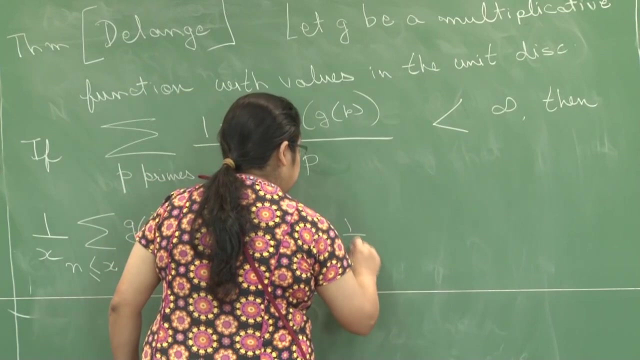 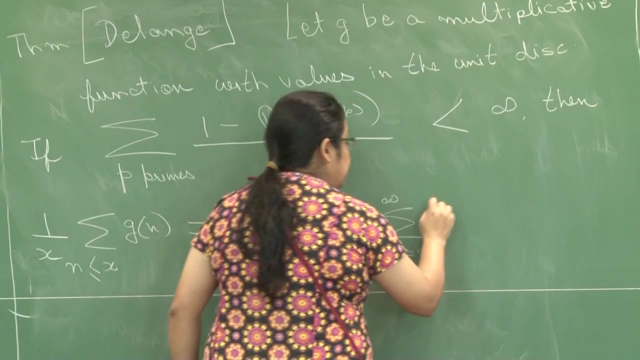 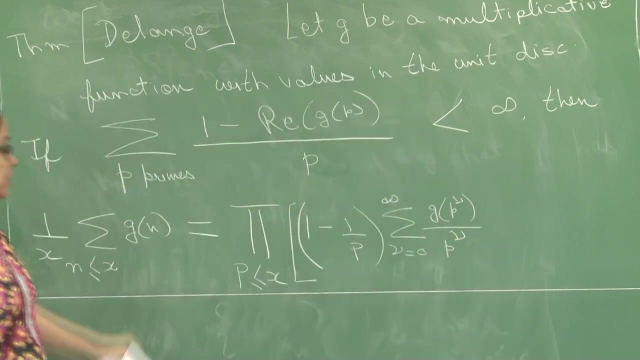 So the product runs over all the primes up to x and you have, for each such p, you consider 1 minus 1 over p into summation nu, going from 0 to infinity G of p raise to the nu. If you have this, Ok. 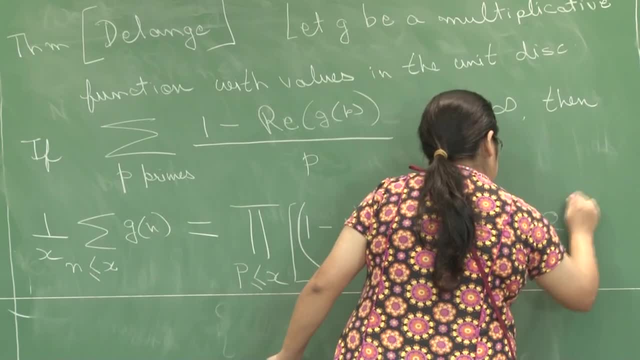 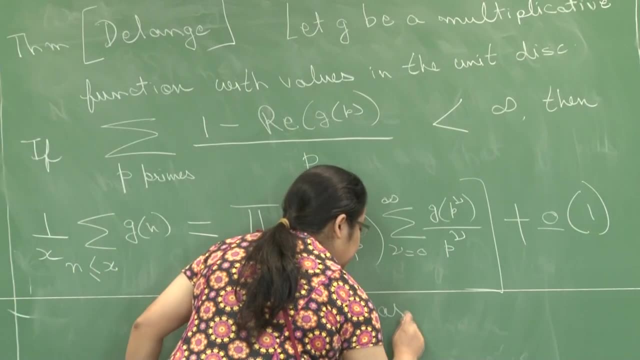 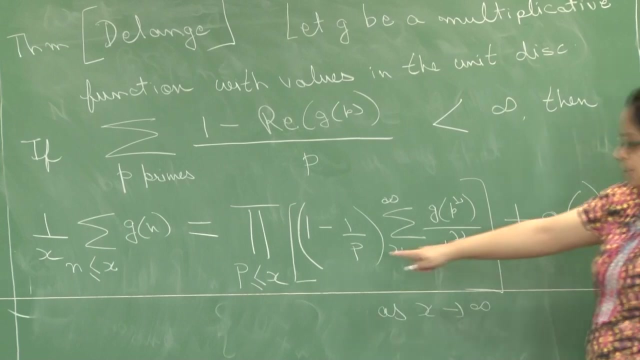 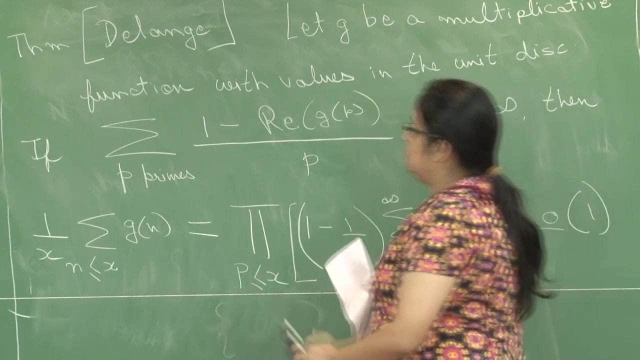 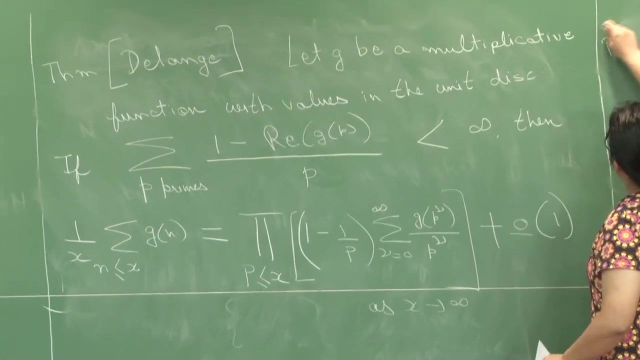 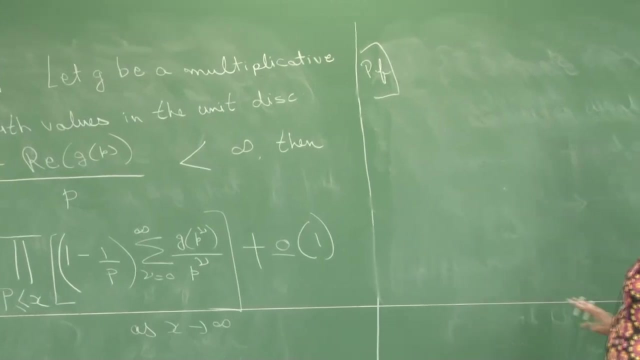 then as x goes to infinity. Now why would you even guess something of this form? The proof will make it clear. okay, So here is. so here is what we do. if you want to prove this theorem, Let us first sketch the main points of the proof. So what we do is instead: 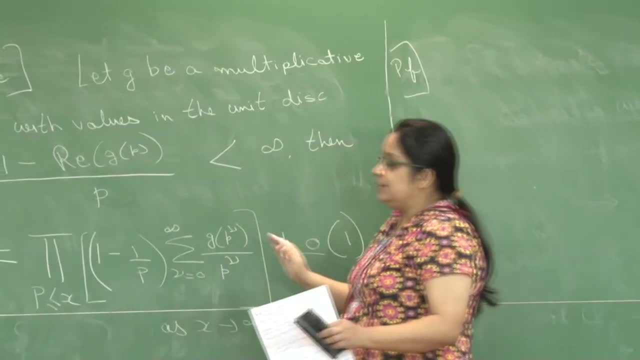 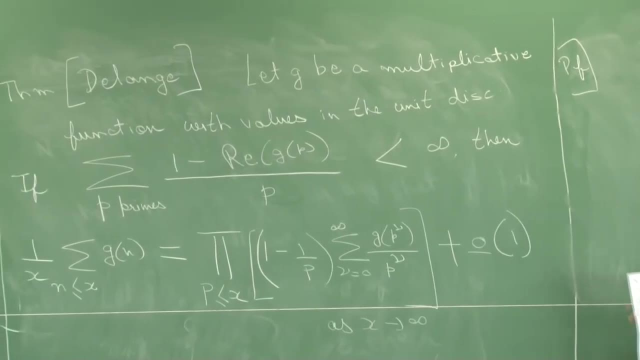 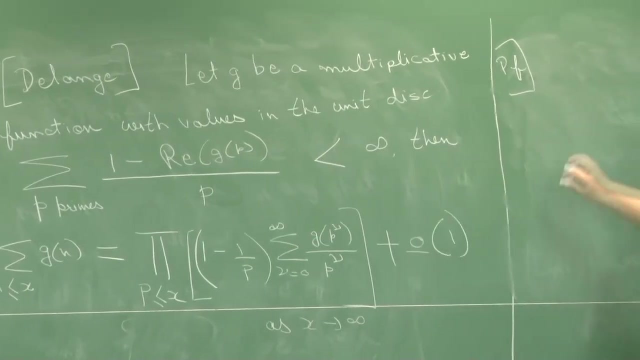 of looking at G of n, we consider certain whatever like nicer forms of G. So this is what we do. So for each, let us take so step 1, so I am first going to tell you briefly what are the main steps. 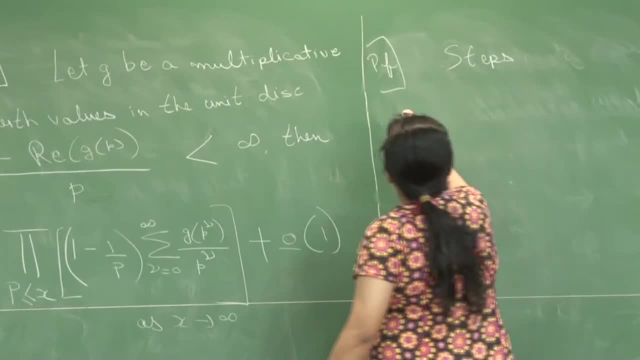 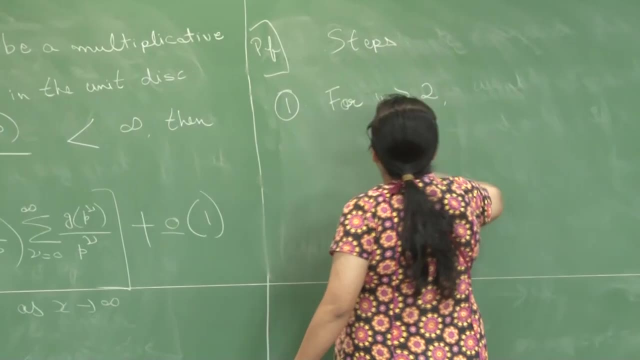 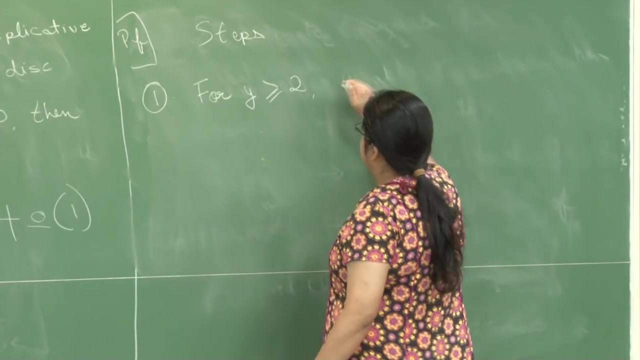 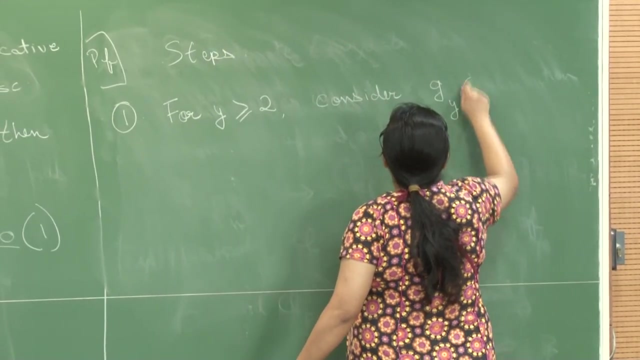 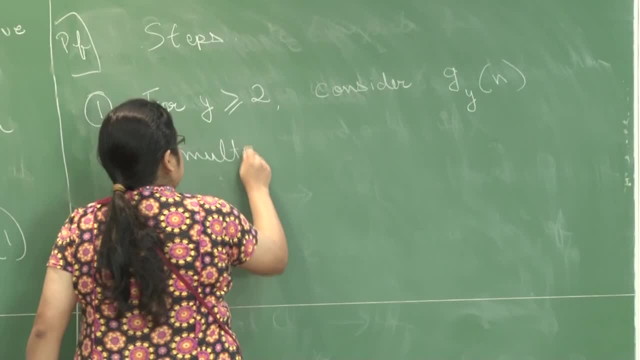 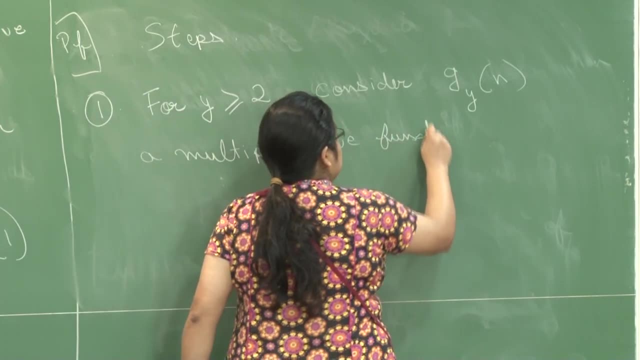 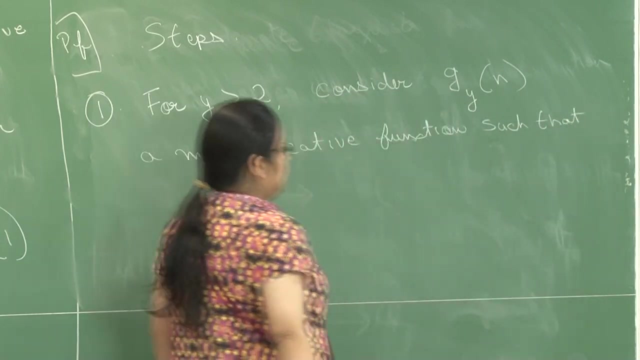 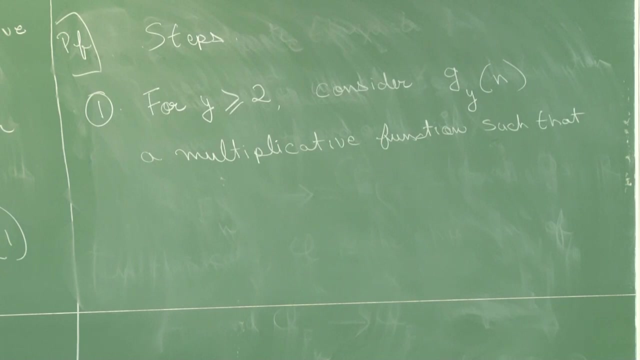 here we have a say f and d, We have z and n. So let us take Each of these local f and z became equal to G of n. Let us Such that. how do we define? to define a multiplicative function, it is enough to define it at its 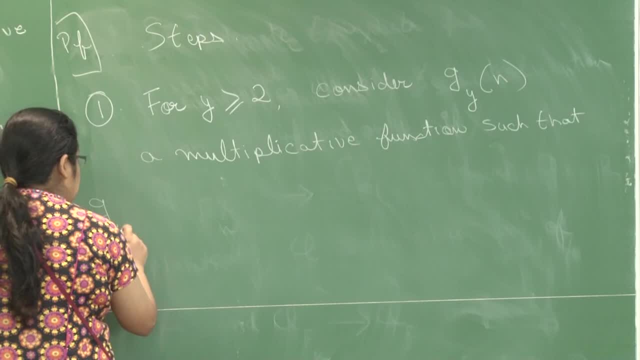 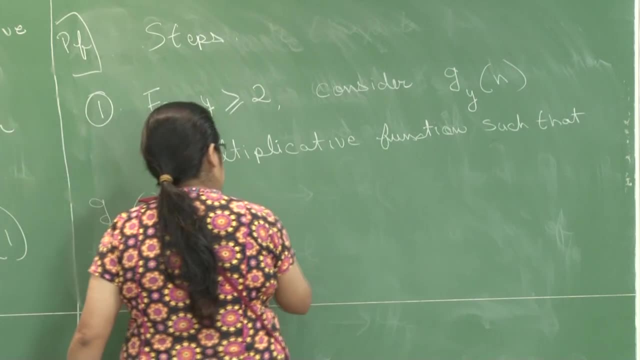 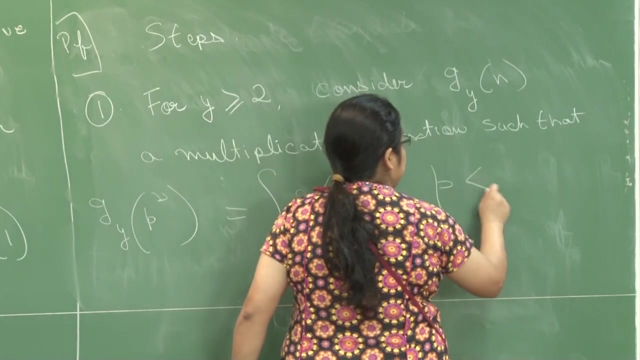 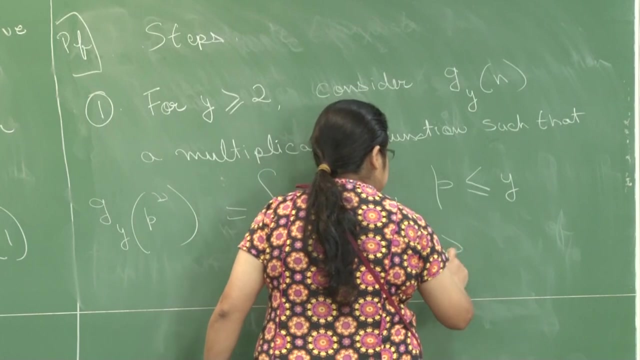 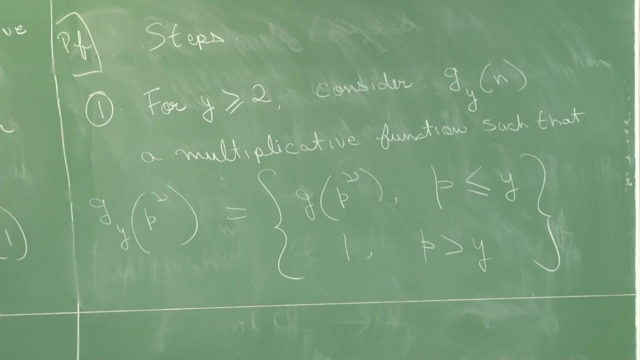 prime powers: g sub y of p raised to the nu. any prime power is equal to g at p raised to the nu, provided your prime is bounded above by y and it is 1 if p greater than y. So this behaves in some form. this is, you can think of it as some kind of a descent of y. 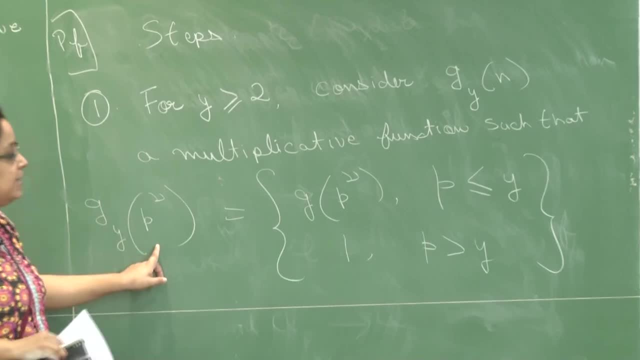 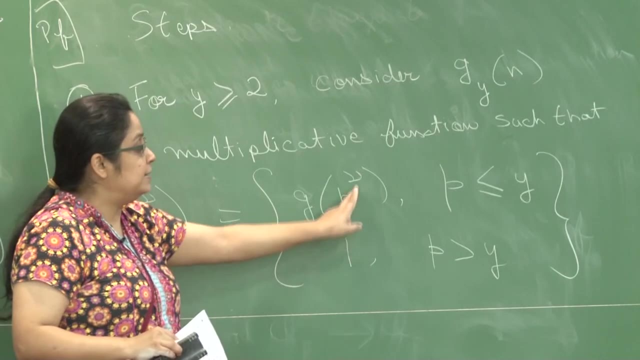 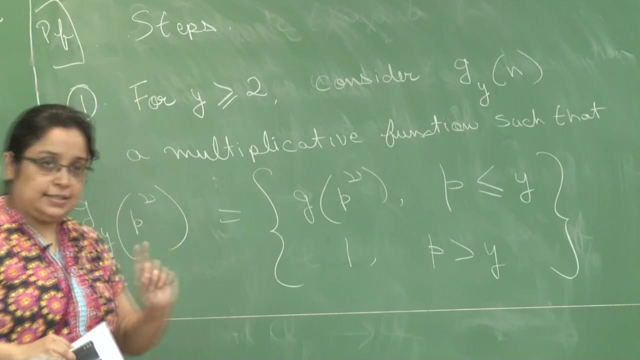 of g, where now it is taking exactly the same values as g at those prime powers where the primes are less than or equal to y. I am not saying that the prime powers are up to y- prime powers could be very, very big- but that prime p itself has to be less than or equal. 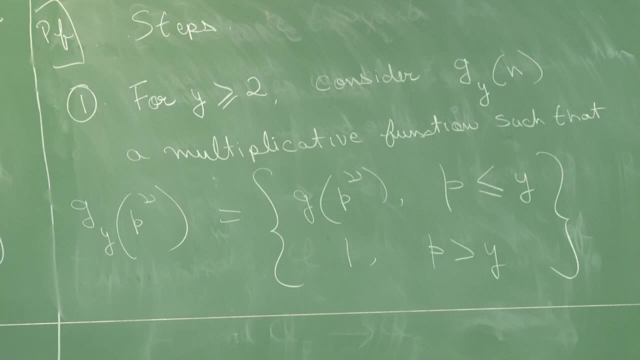 to y. okay, Now, if so, you can define this function, g sub y of n, as follows: once you know how it behaves at prime powers, you know how it behaves at all the natural numbers n, and, of course, you also know that g sub y of 1 has. 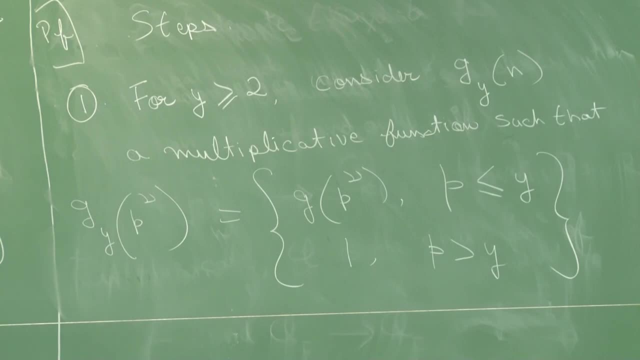 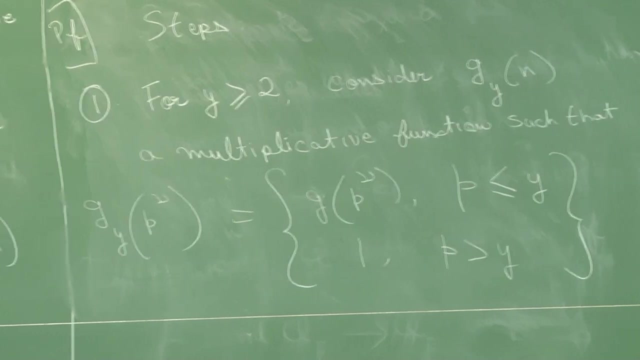 to be equal to 1.. So, given this, what we do is we are able to show that the mean value of g sub y of p, raised to nu, is very similar to the mean value that you want to take here. okay, So we show that. 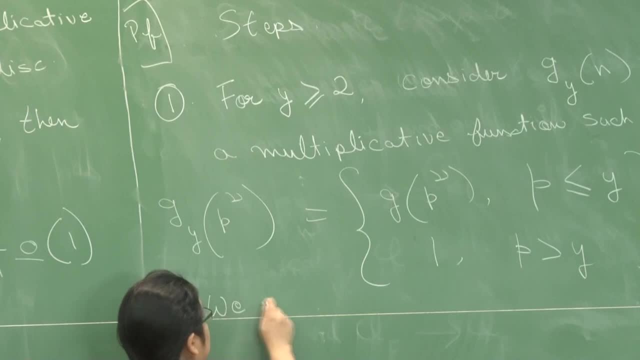 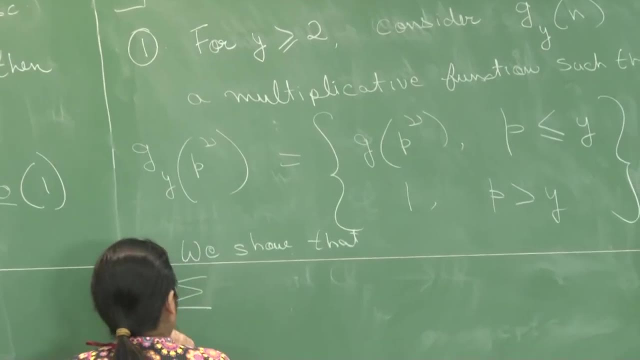 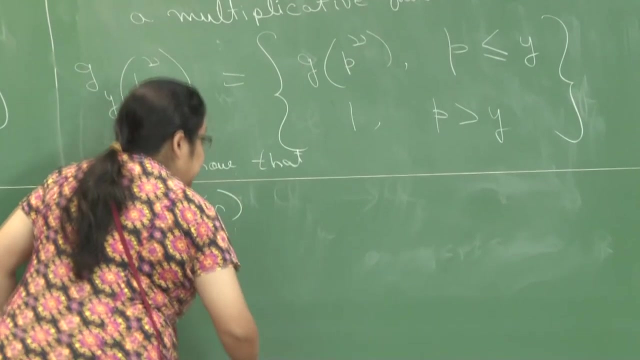 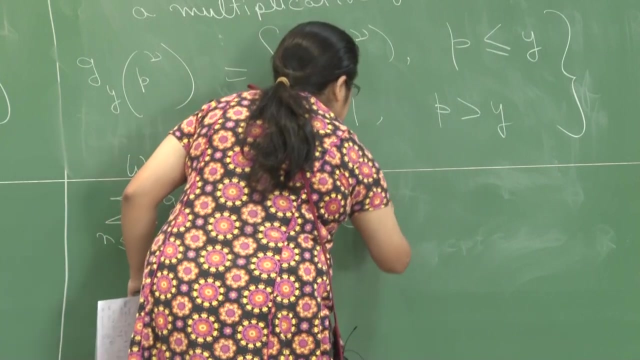 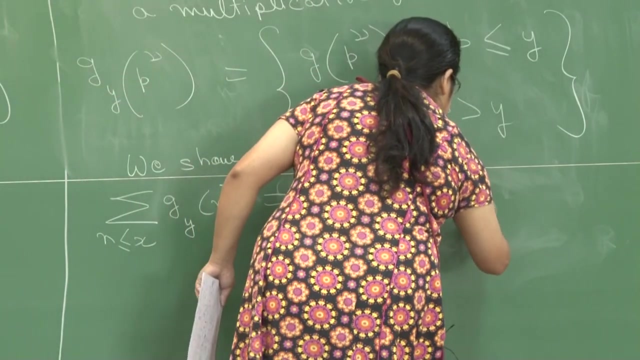 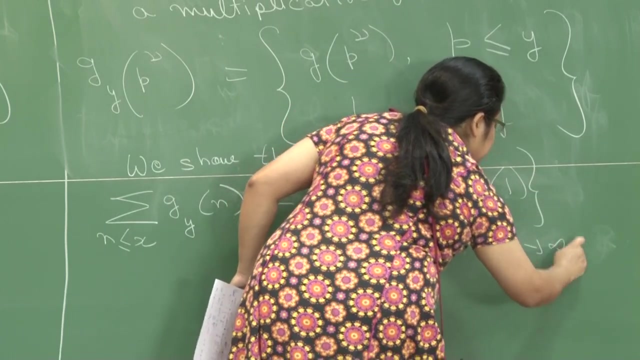 Summation n up to x of g sub y of n. okay, it turns out to be equal to x times a function, m of g sub y, Which I am going to define Shortly, plus little o of 1, as x goes to infinity, where what is m of g sub y is defined as the. 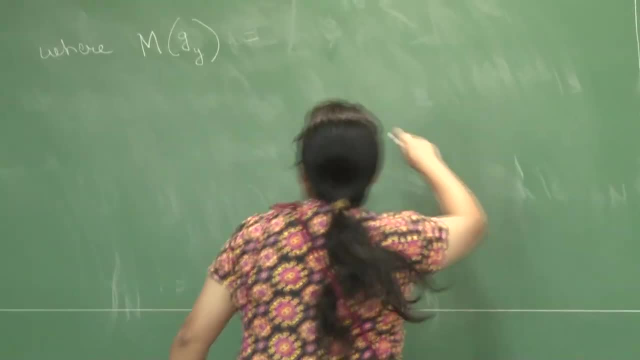 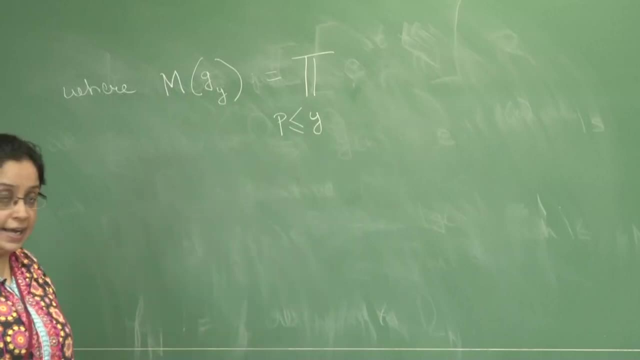 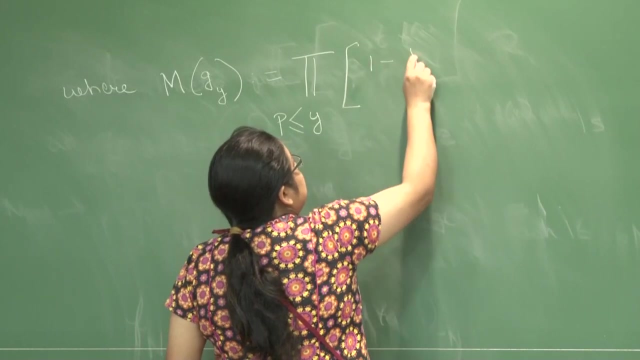 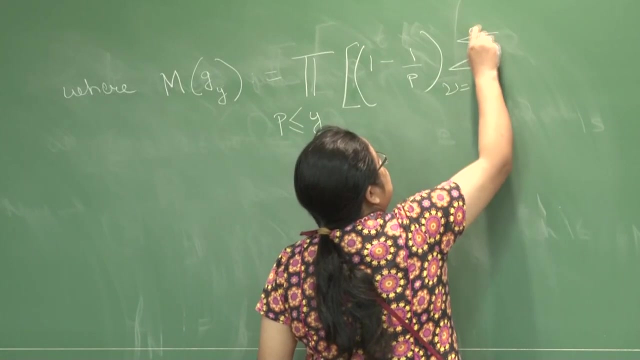 function. you have the same product but with the products with the primes running up to y instead of x. okay, So suppose you have 1 minus 1 over p into summation nu, going from 0 to infinity g of p raised to the nu over. 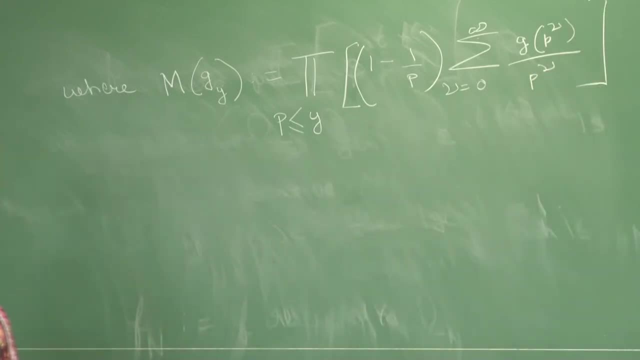 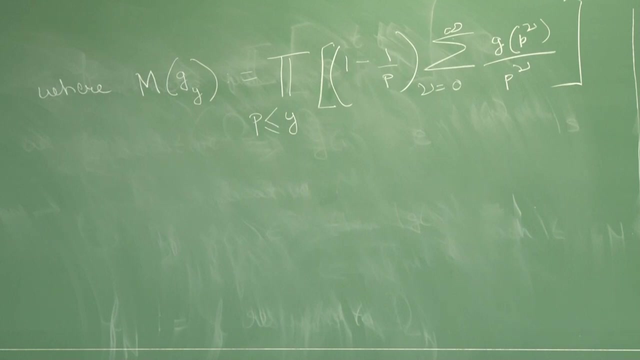 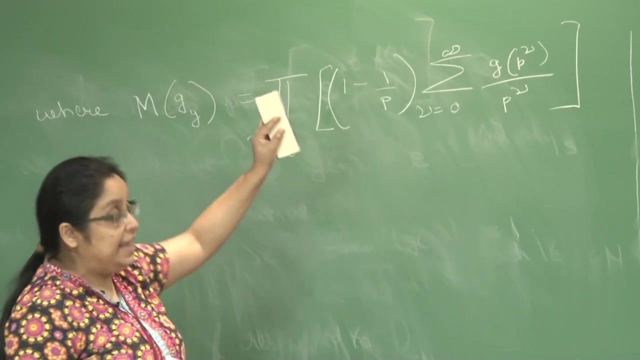 p raised to the okay. So what we show is that the essentially what this is saying, this, this equality here- okay- Is saying that, As This: this function m of g sub y is the average order of your function g sub y, and that is. 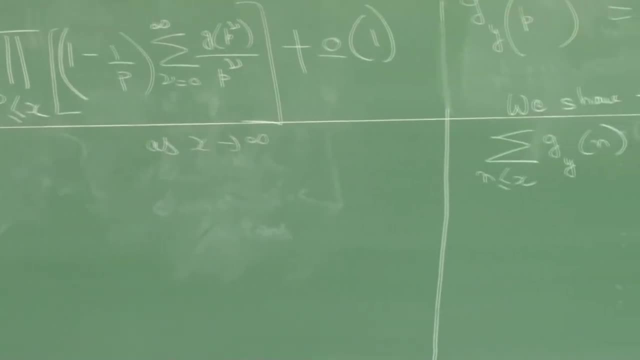 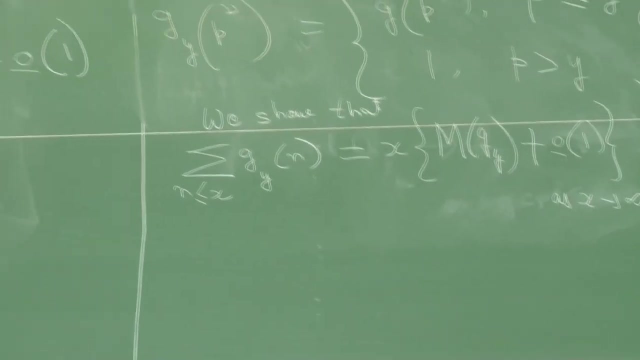 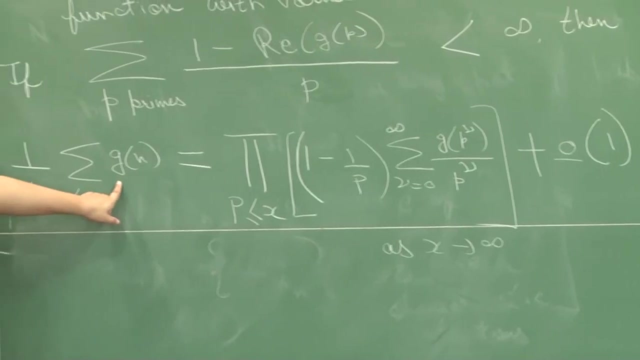 why we denote it as m of g sub y, m referring to the word mean. okay, So the mean value of g sub y is this function. then what we show is that our g sub y's are actually good approximations to g, And therefore what happens as y goes to infinity? 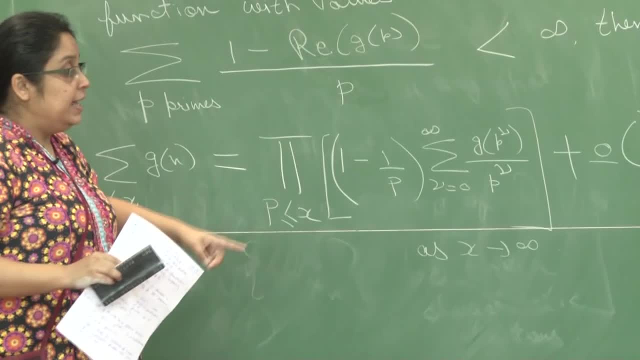 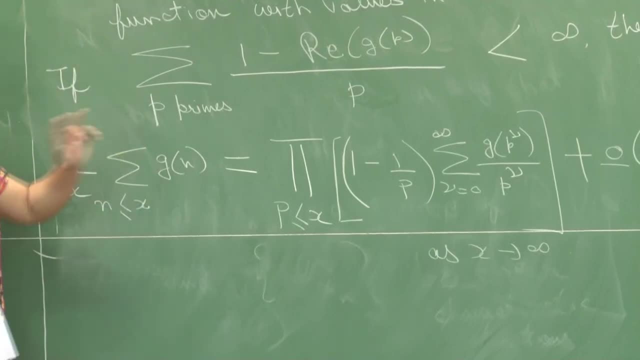 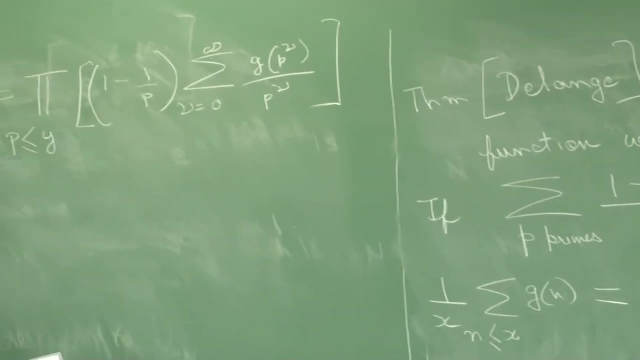 So that is why we denote it as m of g, sub y. m, referring to the word, mean okay, And therefore what happens as y goes to infinity is that you end up getting the corresponding equality for your big function, the universal function g. okay. So next step, what we show is the following: 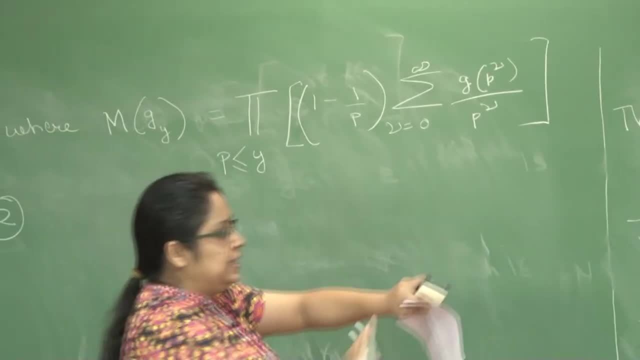 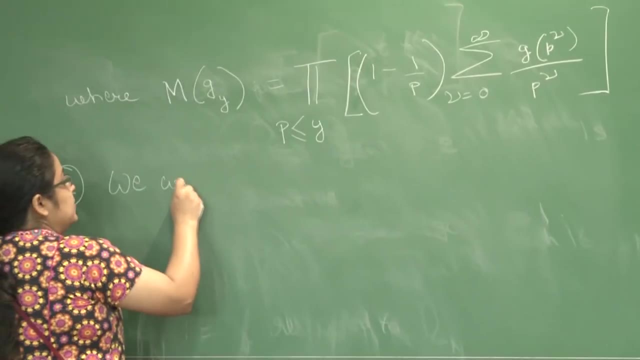 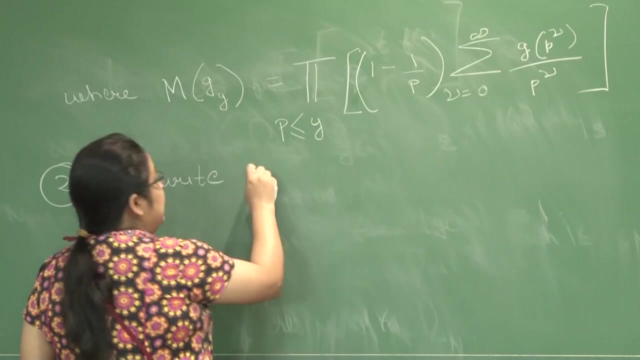 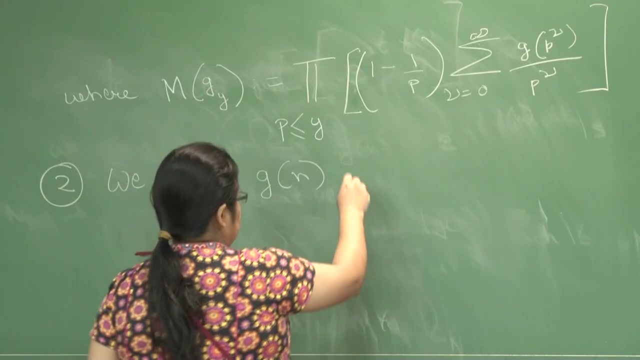 So this looks a little strange, but let me explain. so what we do is we take, so we write. Suppose you have a function which is a complex valued function and you also know that It is taking values on or inside the unit circle, then we write. 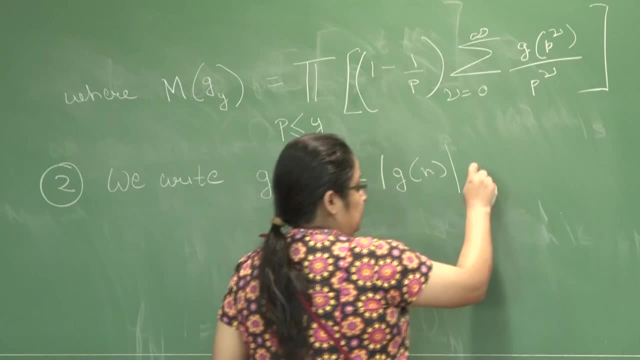 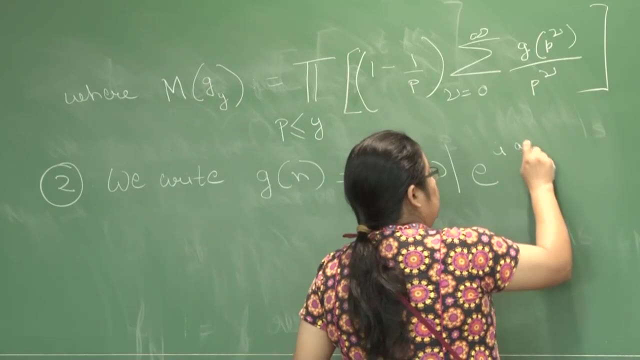 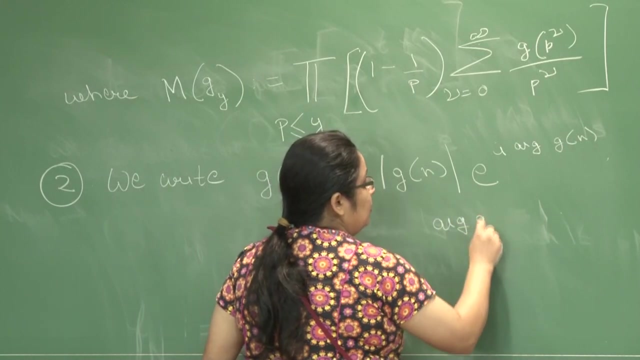 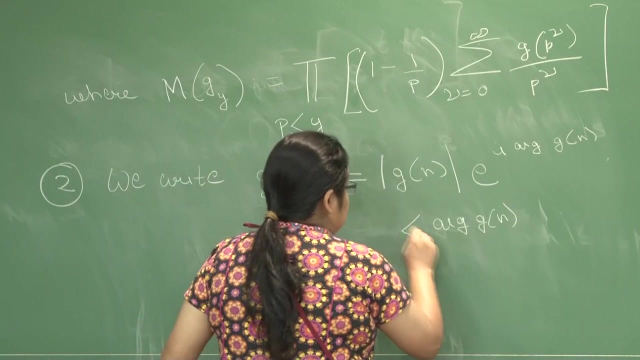 This as absolute of g of n, raised to the e, raised to the i times, what you call the argument. Okay, So what we do is we define this as m of g of n, where you choose your argument. okay, this is just the corresponding angle. what I mean to say is that 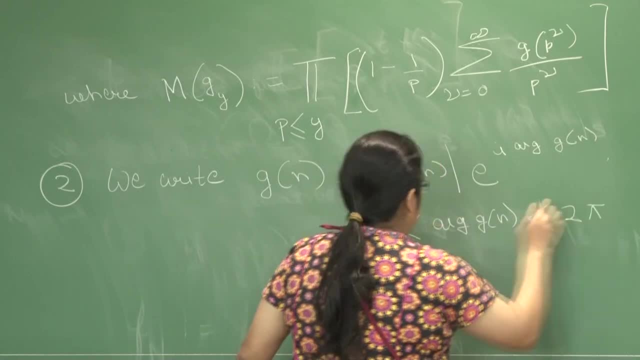 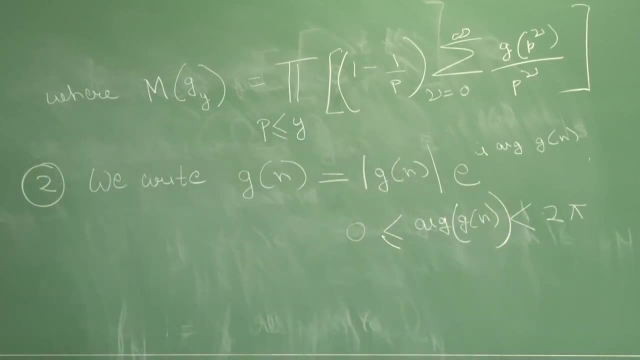 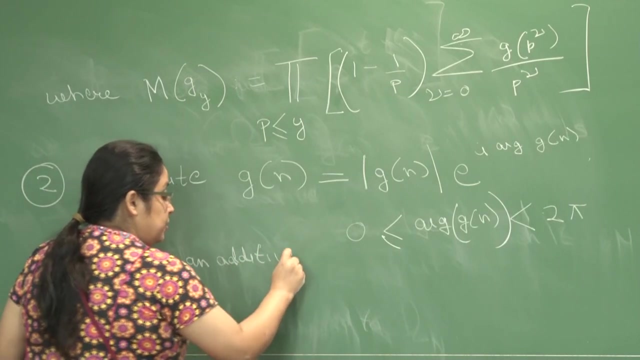 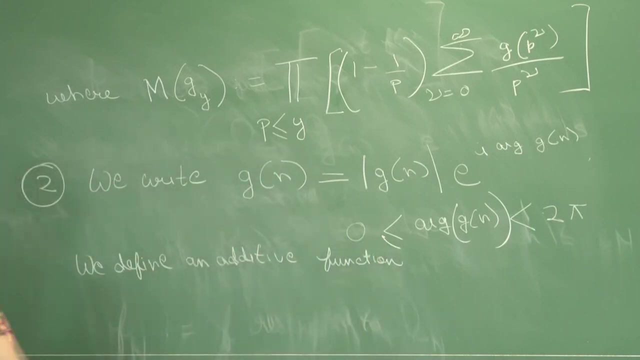 So this lies between 0 and 2 pi. okay, all right. So with this in place, now what we do is we define An additive function. Let us call it theta of n. as follows: This theta of n. again, to define an additive function, it is sufficient for us to define. 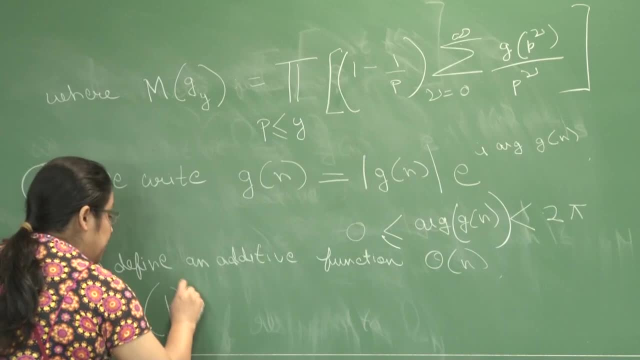 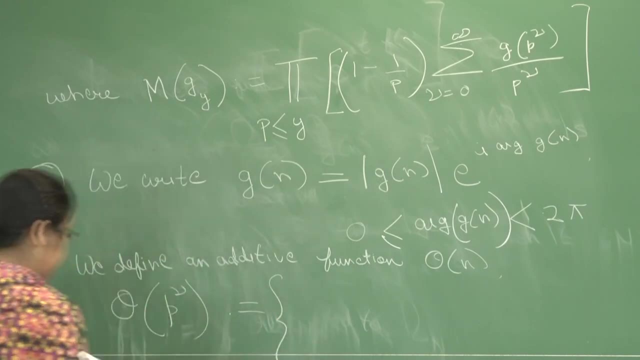 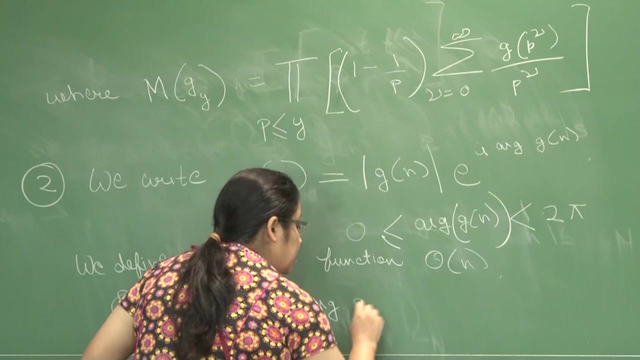 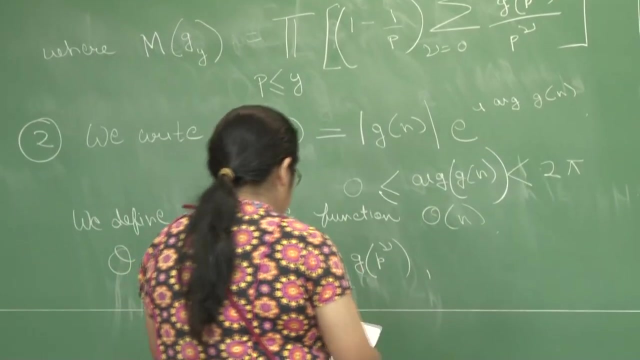 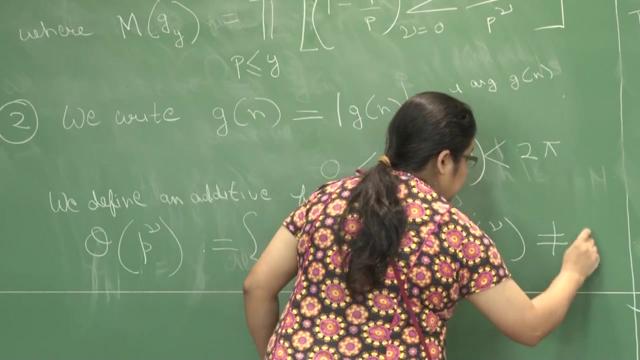 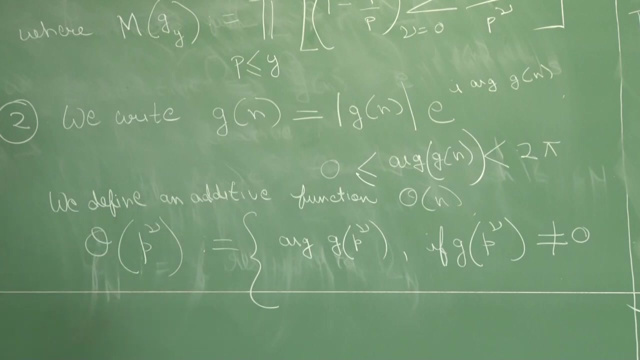 it at prime power. Okay, So for any prime power p raised to the nu, theta of p raised to the nu is defined as our angle corresponding to g of p raised to the nu. okay, Where your, If you have g of p raised to the nu not equal to 0, then the corresponding angle is your. 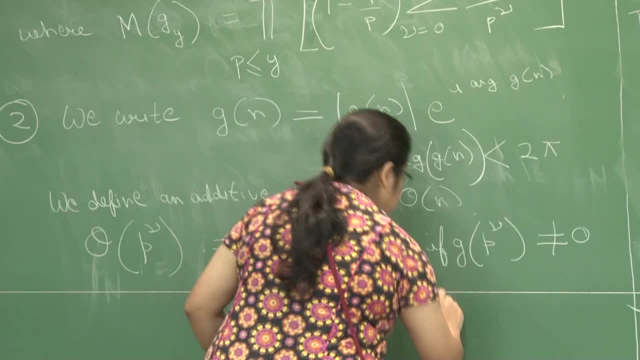 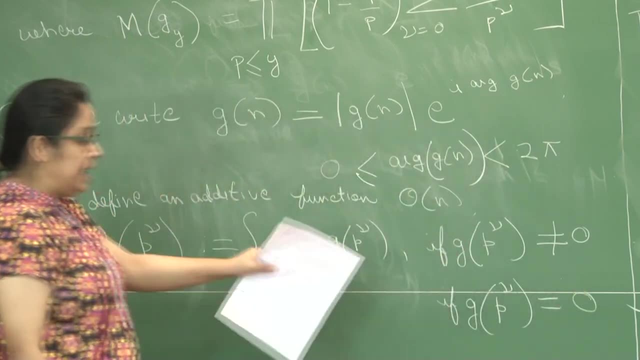 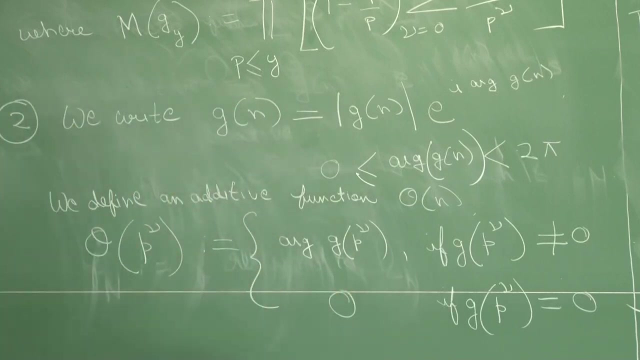 theta, and if G takes the value 0 at a prime power, p to the nu, then you just take this to be equal to 0.. Alright, So suppose you have a function which you define at prime powers in this way. you can then consider a more general additive function coming from this. this, the corresponding function. 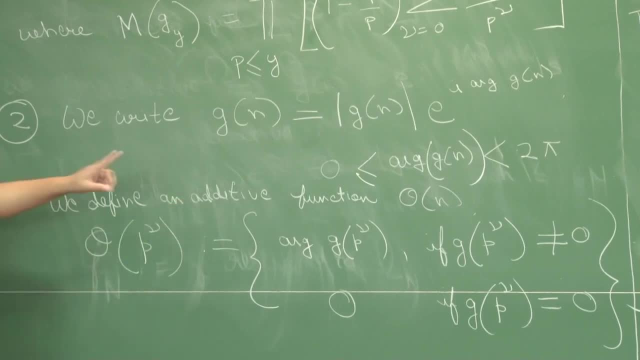 defined at the prime powers. okay, So with this, what we do is exploiting the fact that your theta is an additive function and applying the Turan-Cubileus inequality. Okay, So what we are doing is we are taking these two values and we are giving them the value. 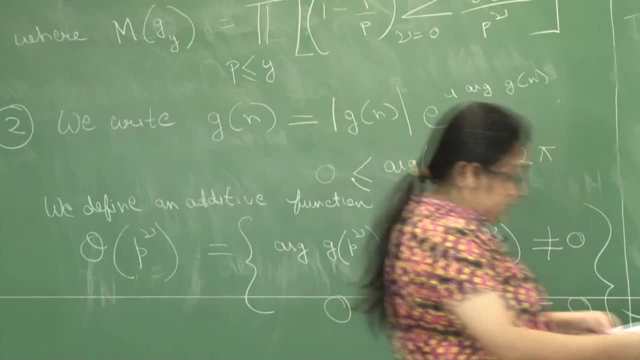 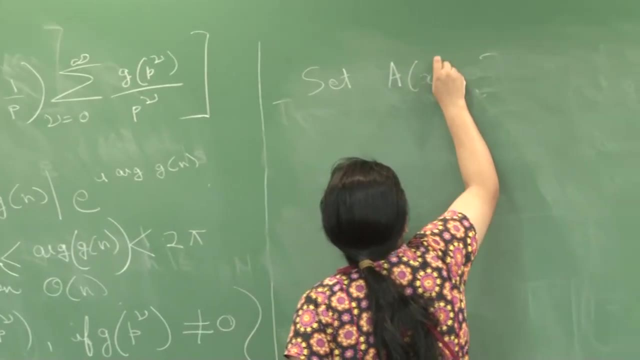 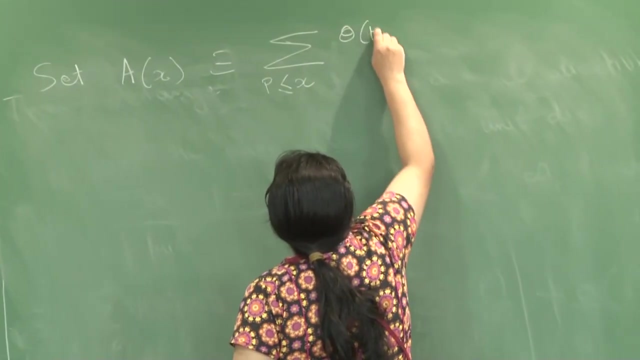 and the maximum value of theta of p. Okay, Now we are going to do a very interesting thing. Let us take the lambda of theta of p and we are going to take thepassive power of theta of p. There it is, So we need this lambda that is equal to. 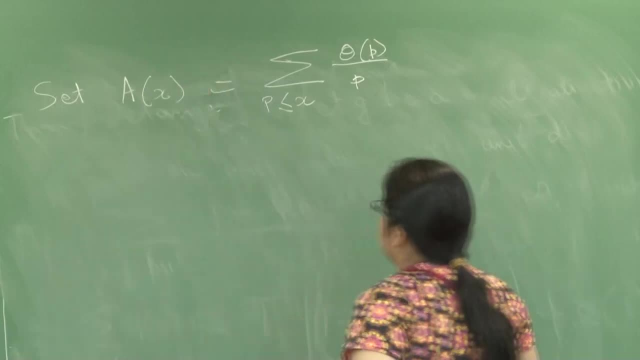 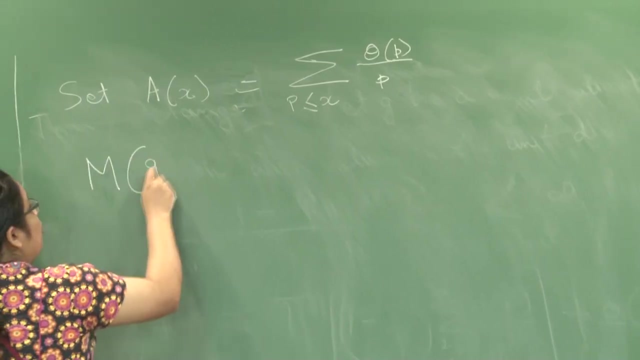 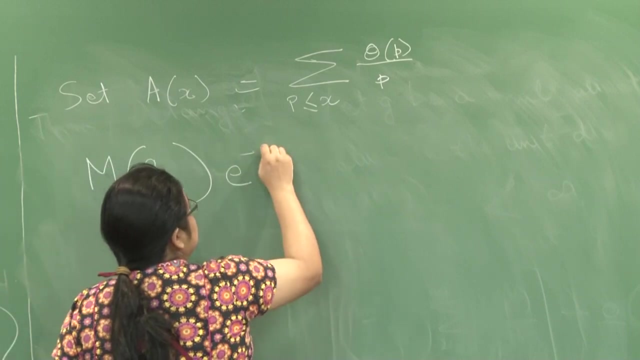 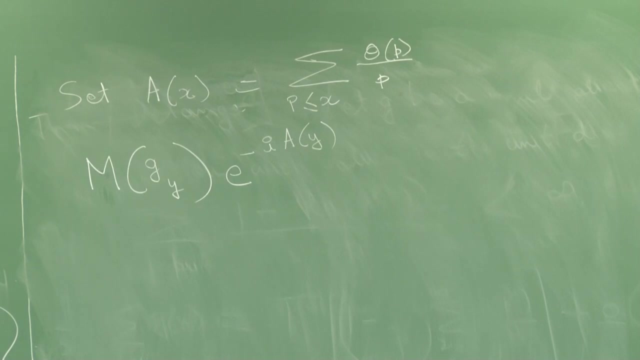 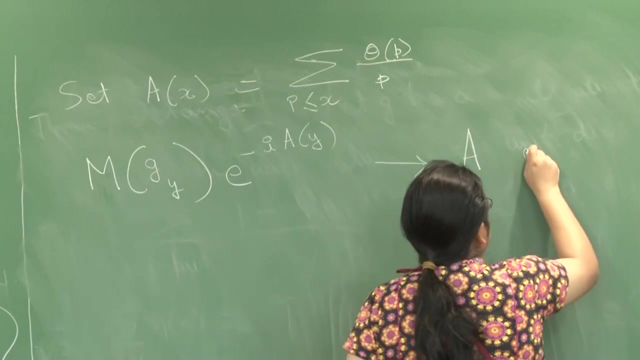 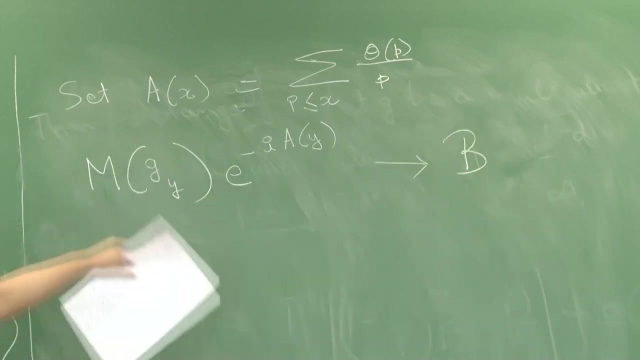 Okay. So then it turns out that our M, the mean value of g sub y times e, raised to the minus i times capital A of y, it converges to a finite limit. let us let us say some A, as not to confuse with the. let us let us call this limit B, as y goes to infinity. 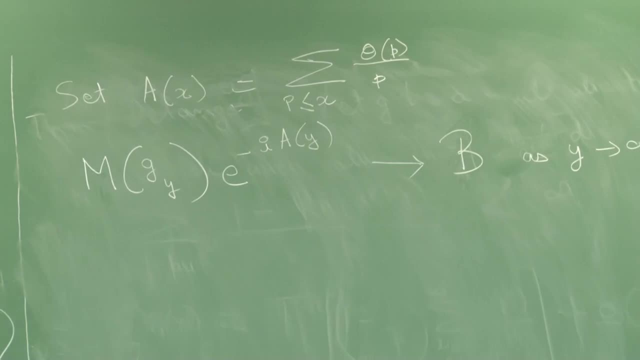 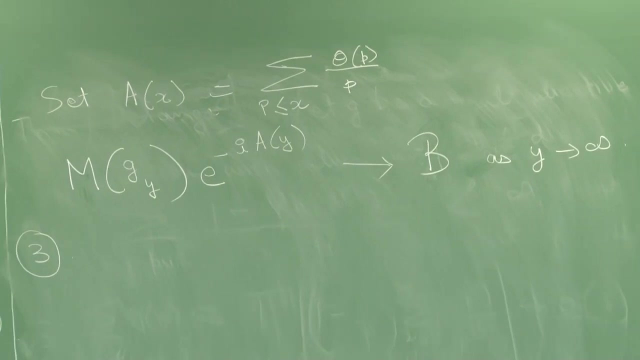 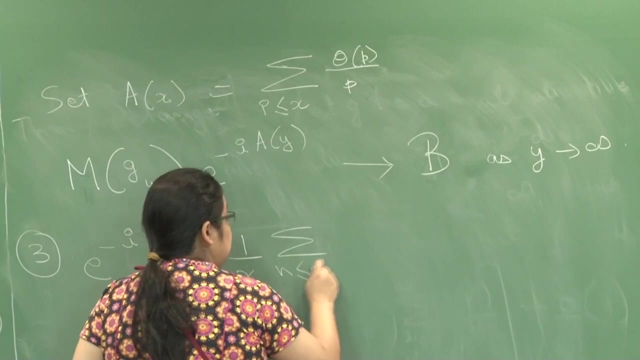 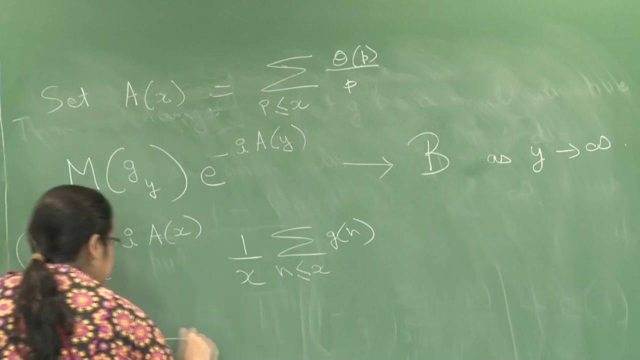 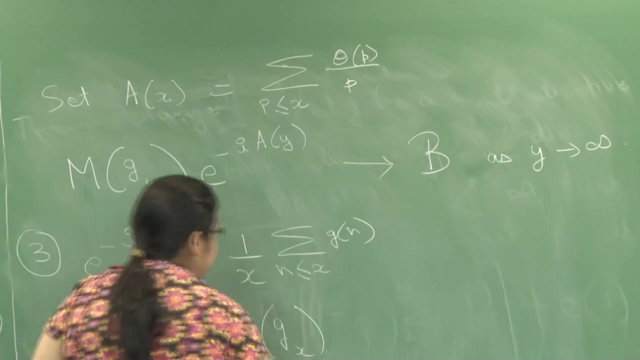 This is the. This is really the step where most of the work happens. and finally, we make the observation that if I take e raised to the minus i times A of x, times 1 over x, into summation of g of n, This converges to M, the mean value, the M of g sub x as defined before, for y equal to x. 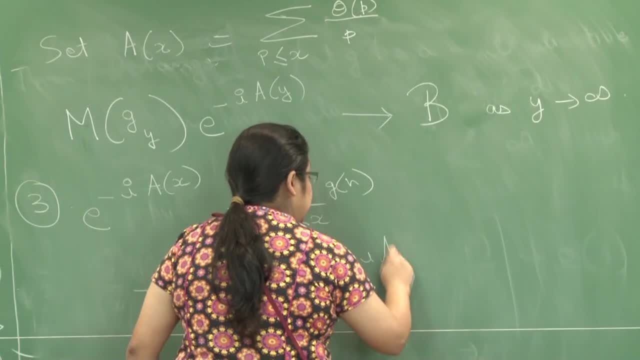 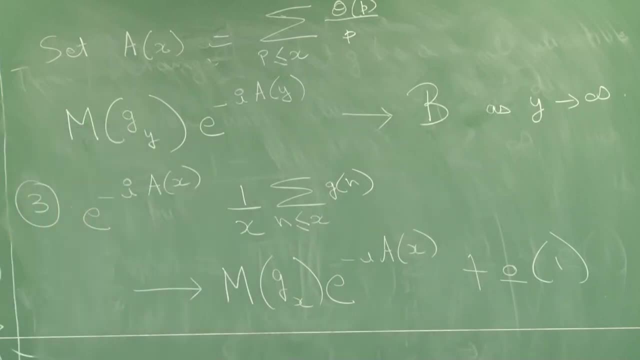 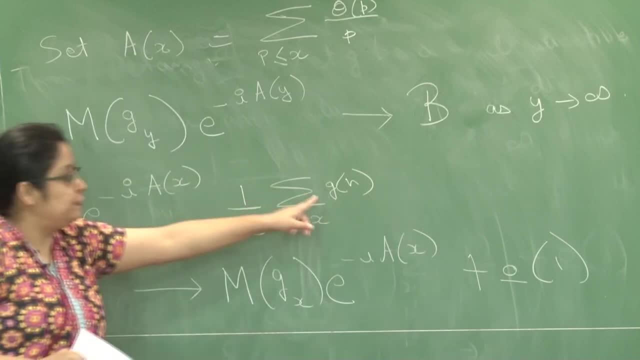 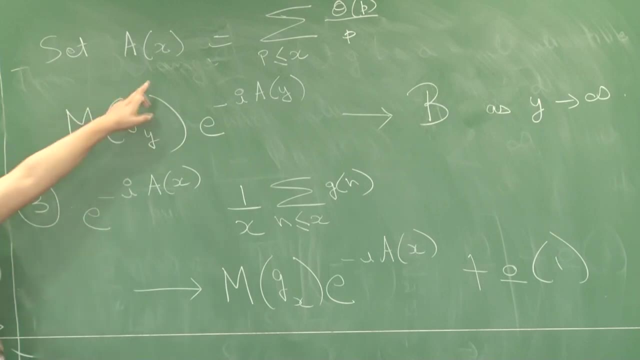 that the average order or the mean value of g of n multiplied by e to the minus i A of x. A of x is the suitably constructed function, gives you something nice, and from this you can deduce immediately that your 1 by x. 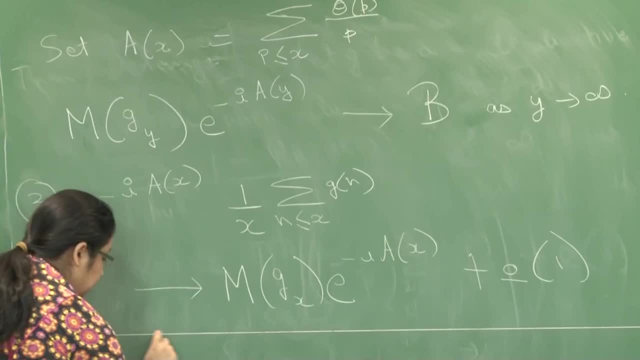 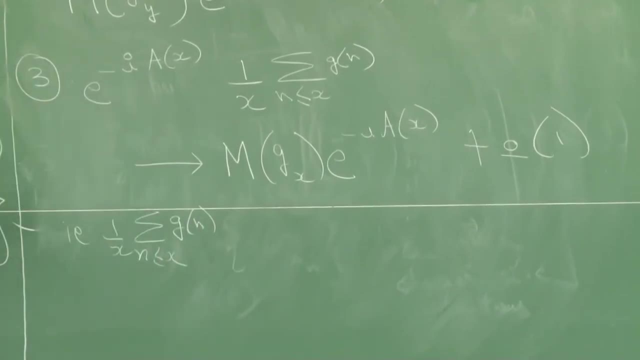 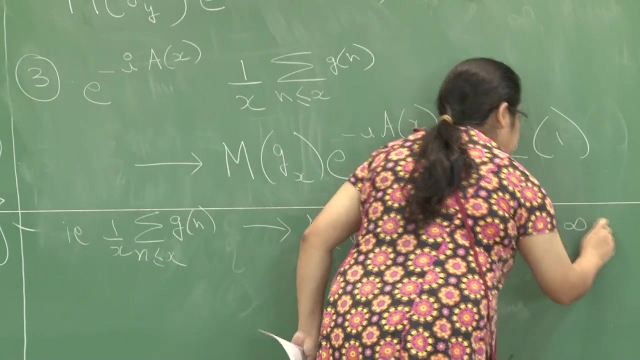 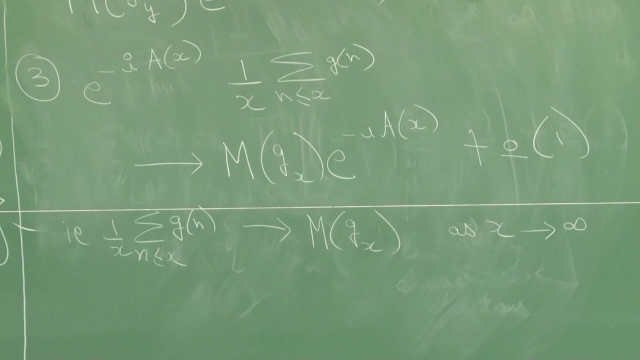 That is, which is the quantity that you are after. okay, this converges to M of g sub x, which is exactly what you were looking for, as x goes to infinity, and this proves the theorem. Okay, So to prove this theorem, now we first look at. so what do we have? we have this universal 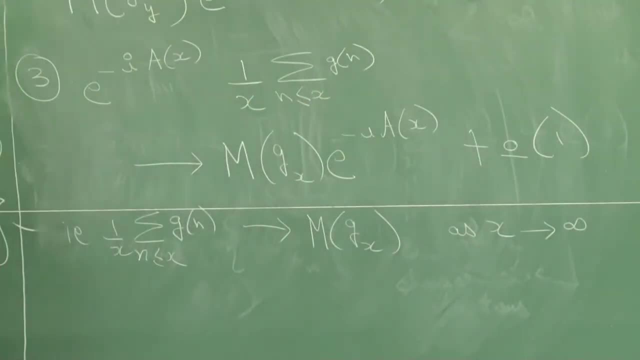 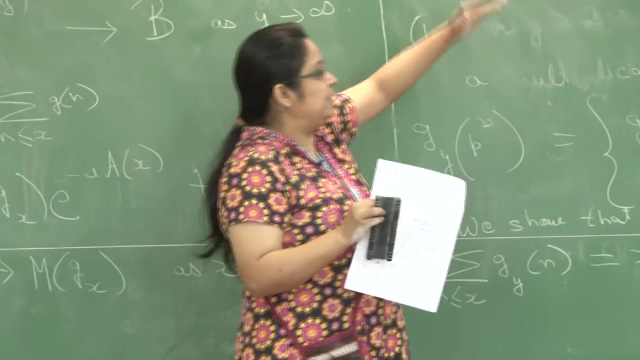 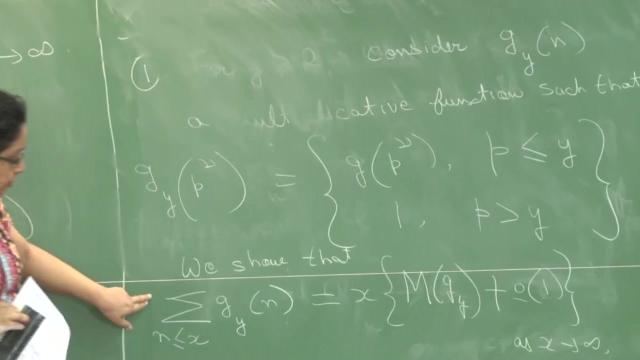 function g, which takes the values that make it a multiplicative function, values lying in the unit disc. Okay, So what we do is corresponding to these. we consider like let us call these local variance of your function g. g sub y is, and we prove this: corresponding mean value theorem for g sub y is first: 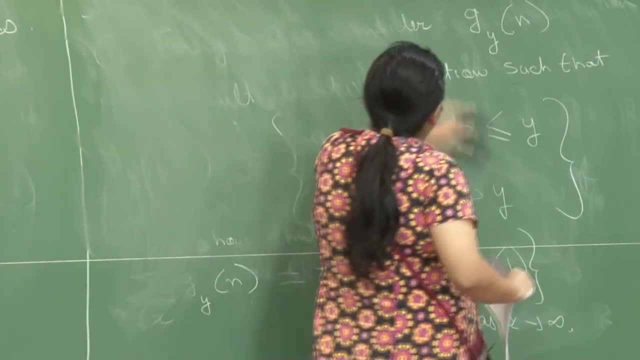 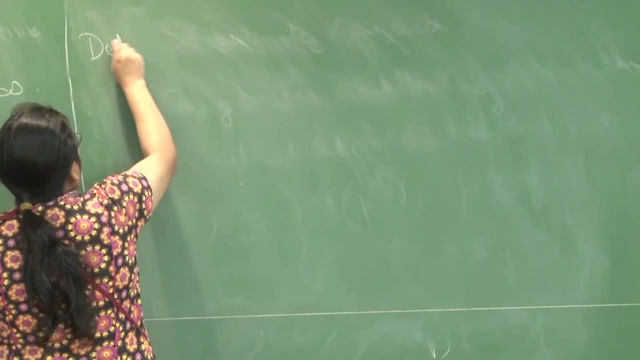 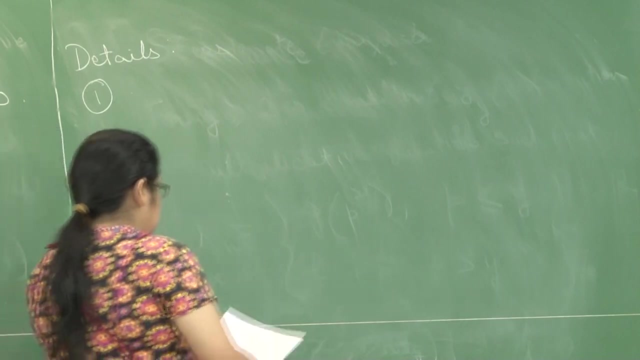 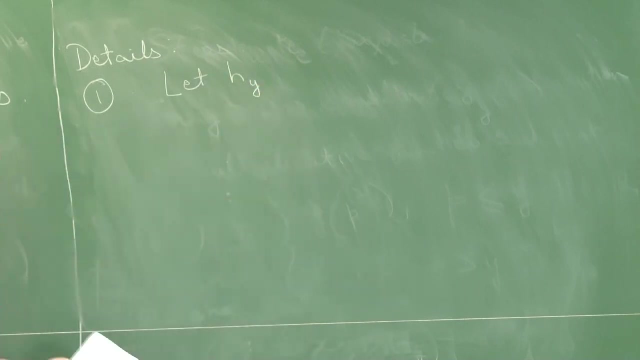 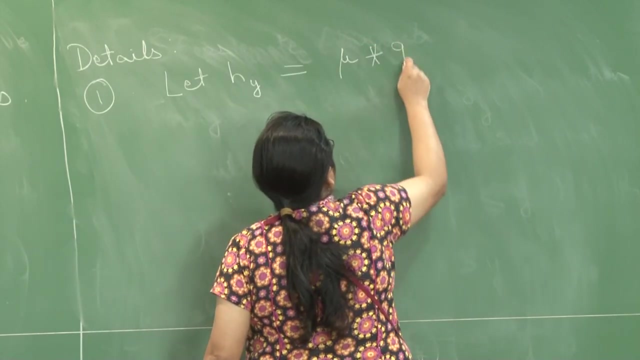 Now, this is a very elementary argument and, in fact, a very nice application of the Mobius inversion formula. So let us work this out details. so, step 1, let us do the following. Let us define h sub y as follows: okay, let h sub y be denoted as the convolution of the Mobius function. 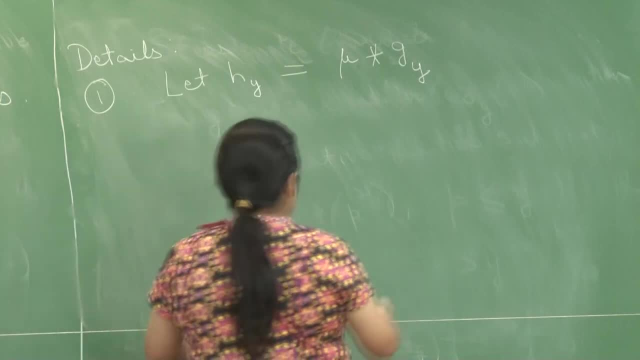 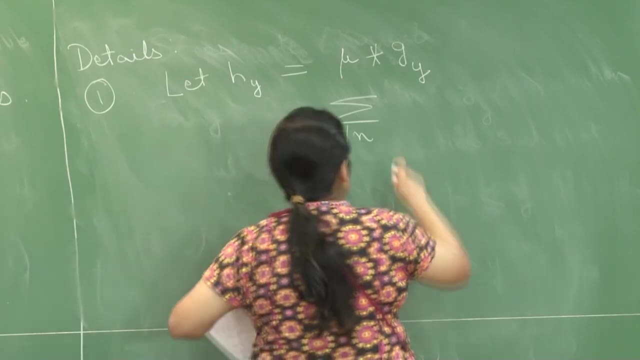 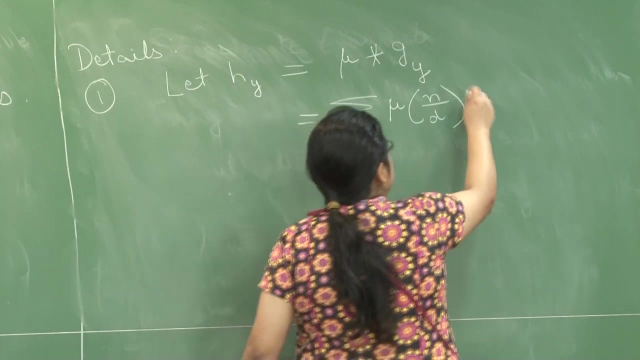 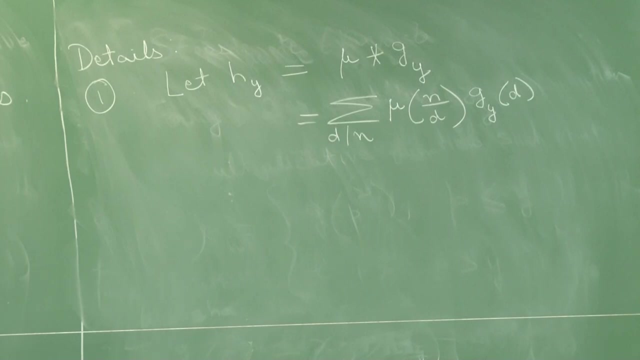 and g sub y. Therefore, what is this? This is the sum, as d runs over all the divisors of n, mu, of n over d, times g sub y divided by g sub y. Okay, So, in particular, this will immediately tell you that if g sub y is multiplicative, so is 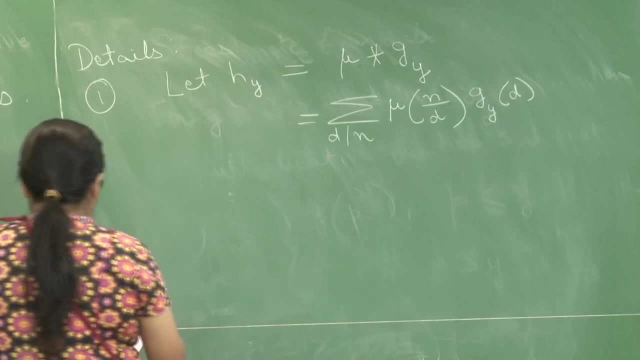 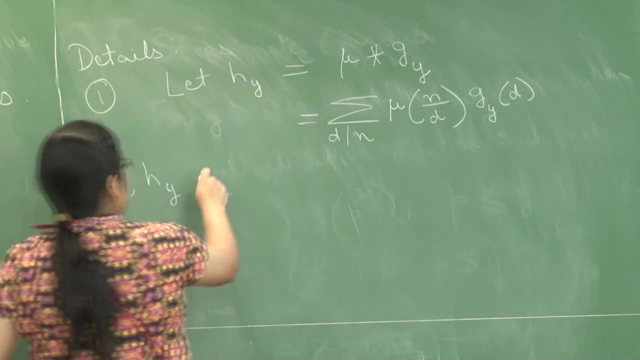 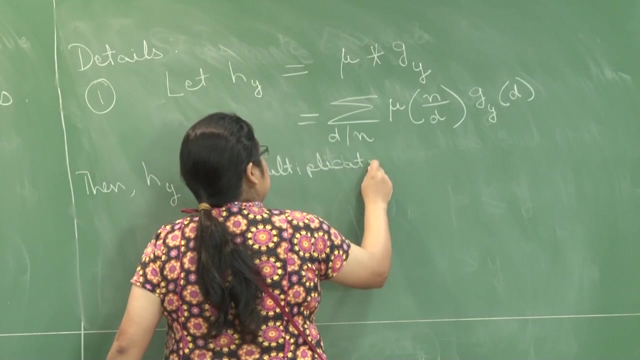 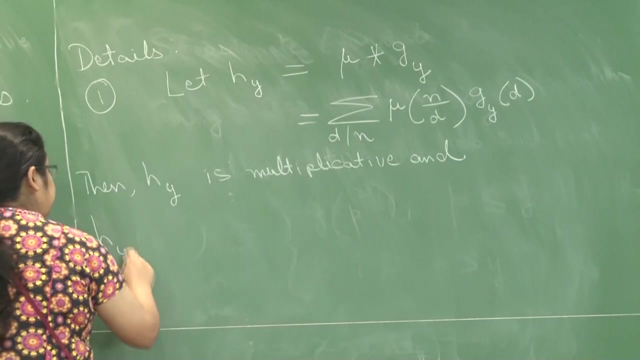 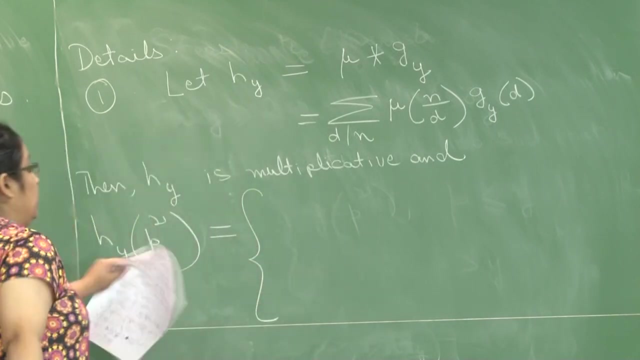 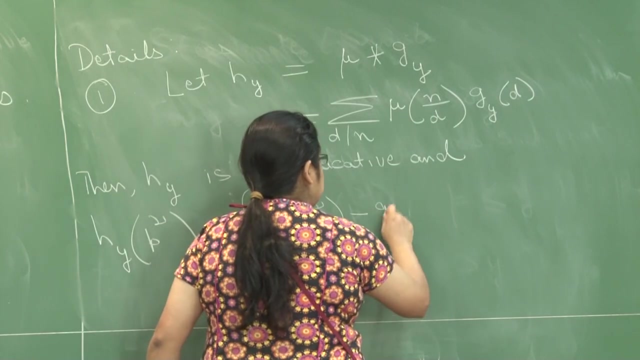 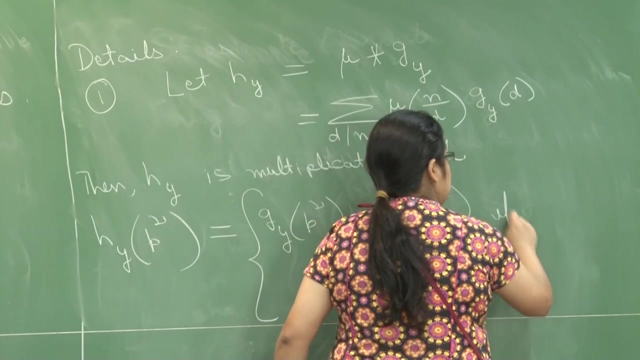 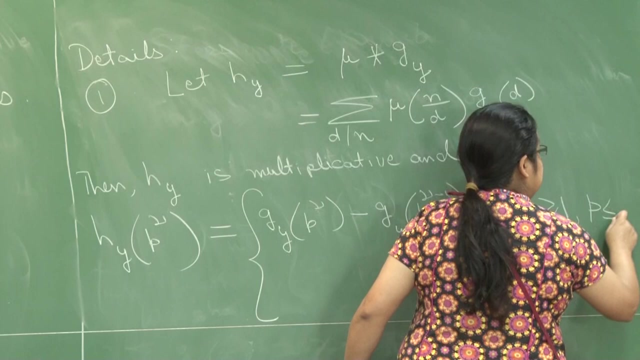 the convolution h sub y and what you also know, the values at prime powers. Okay, Let us consider the values of g, g sub y. Okay, mu is greater than or equal to 1 and p is less than or equal to y. okay, whereas if 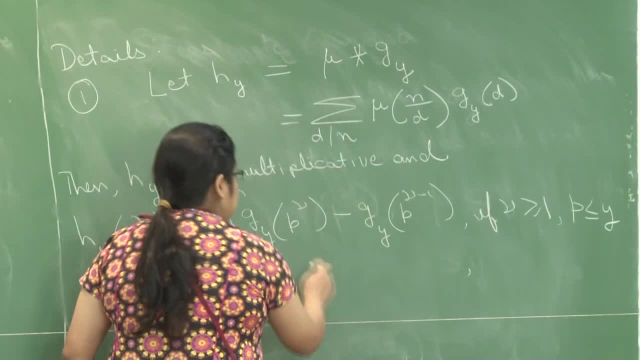 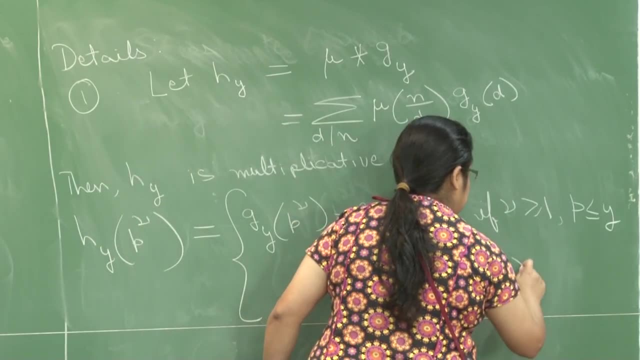 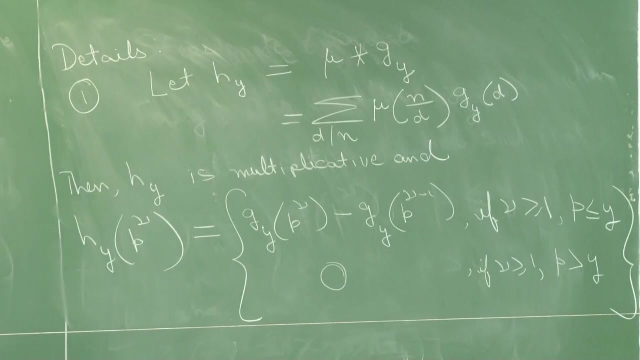 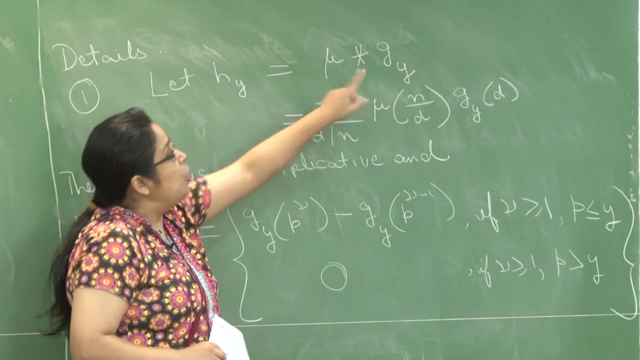 p is greater than y, this will just turn out to be equal to 0,. right Now? what is the significance of this? Now, since H sub y is the convolution of mu and G sub y, what does it mean by Mobius inversion? 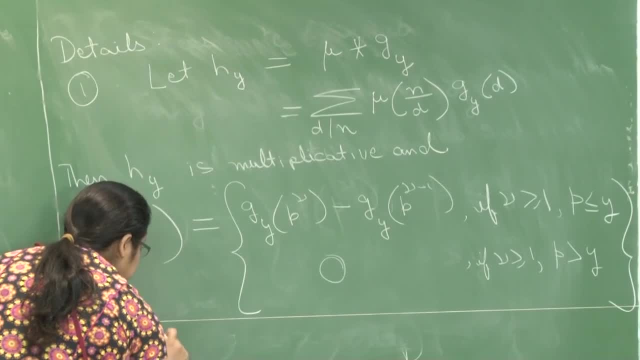 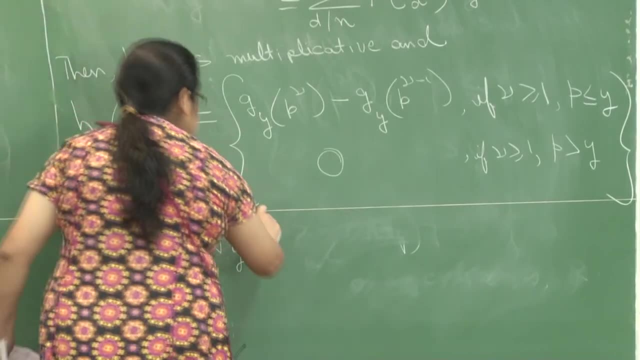 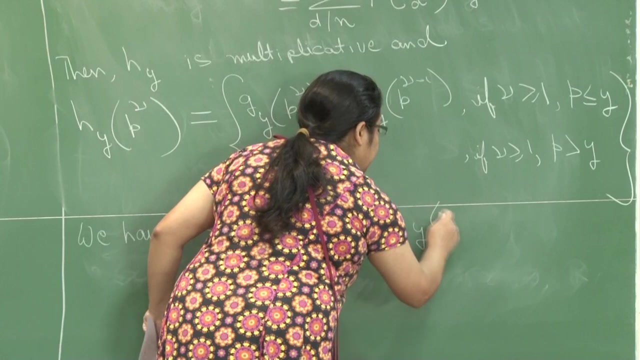 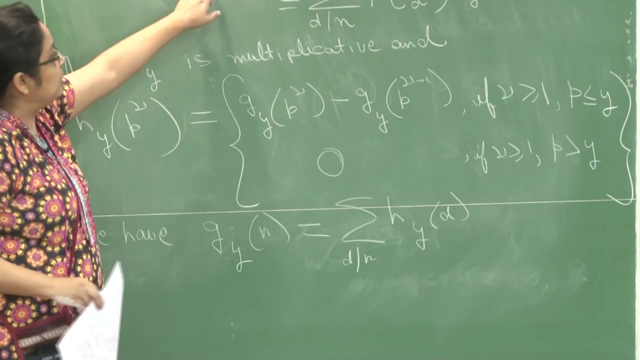 We also have that our G sub y of n can in fact be written as summation over H sub y of all those d's where d run over positive divisors of n. This is just following from our definition of H sub y and the Mobius inversion formula. 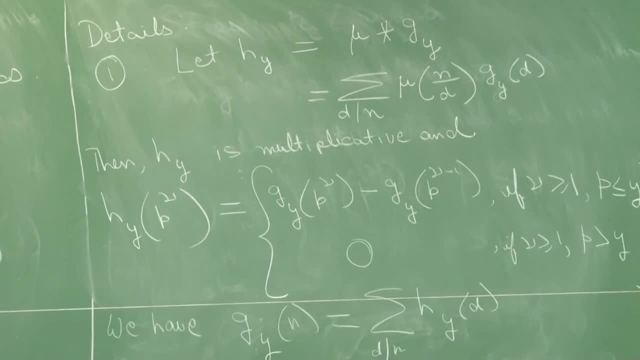 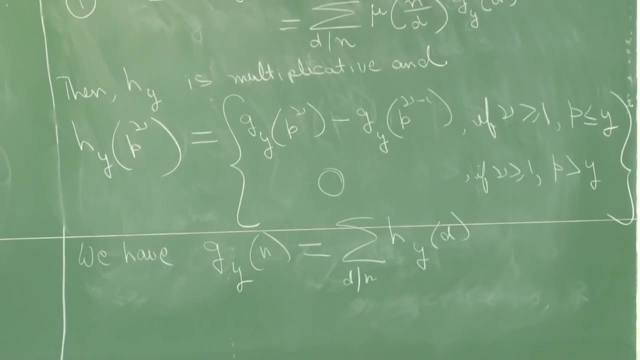 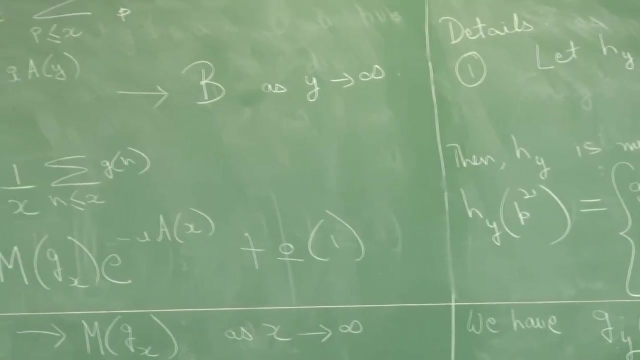 So with this? why is that helpful? By writing G sub y of n in this form, we find a nice simplification for the average order of G that we are looking for. So it turns out that summation n less than or equal to x G sub y of n. 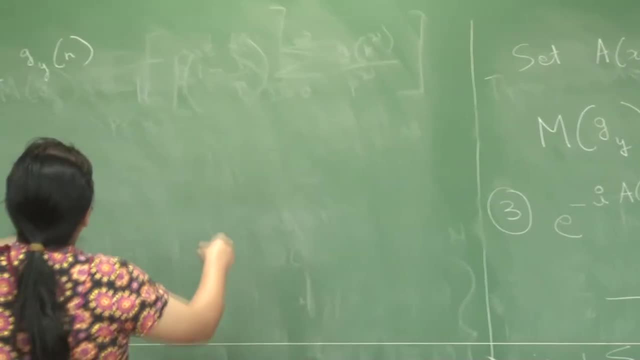 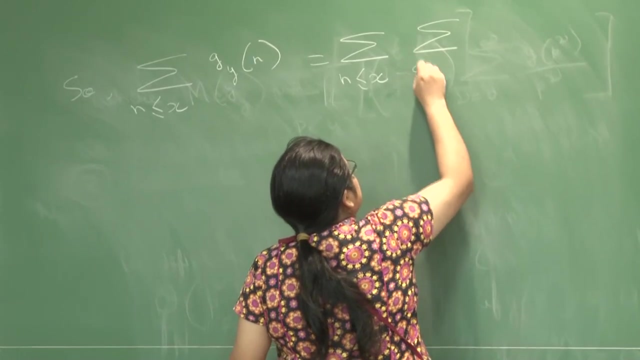 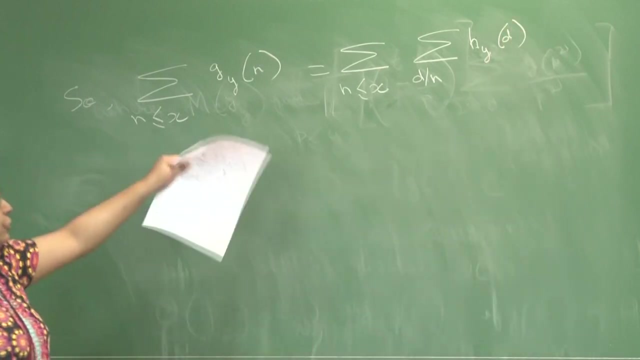 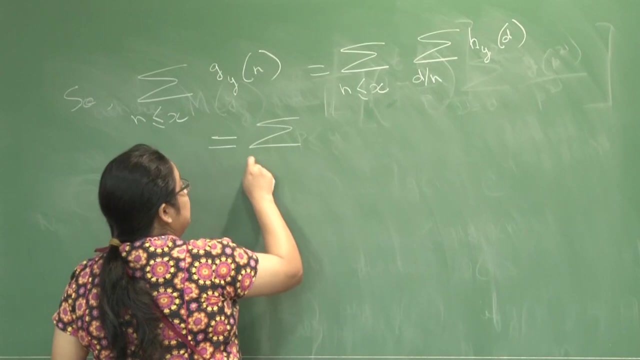 Okay, this is a kind of calculation that we have done several times in this course. So you have an inner sum running over and therefore you interchange this, and by interchanging it what you end up getting is: first, you run over all the numbers up to x. 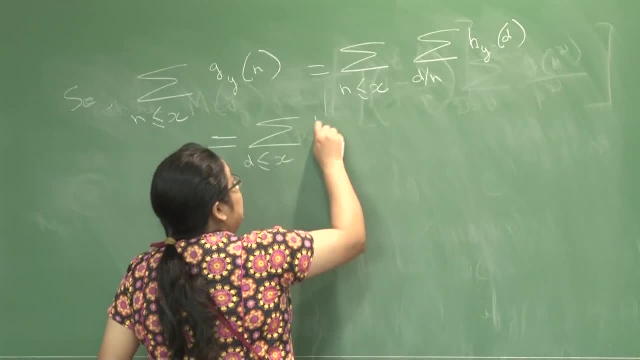 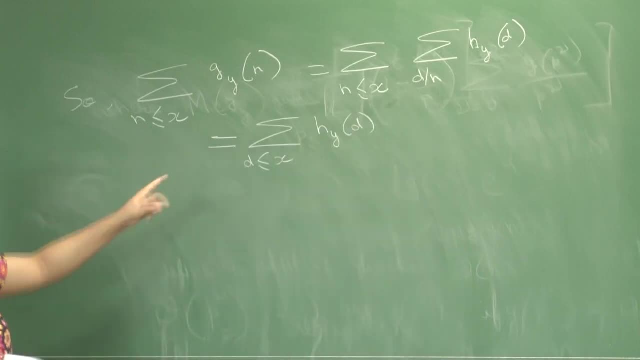 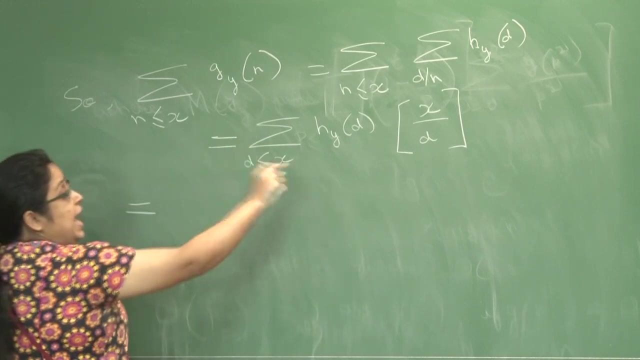 Okay, Okay, H sub y of d, and in the inner sum you have all those n's up to x which are multiples of d. In other words, you simply get the greatest integer of x over d. This is a routine calculation which we have performed many times in this course and therefore 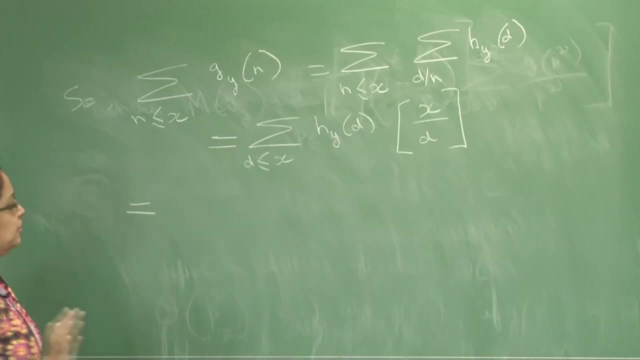 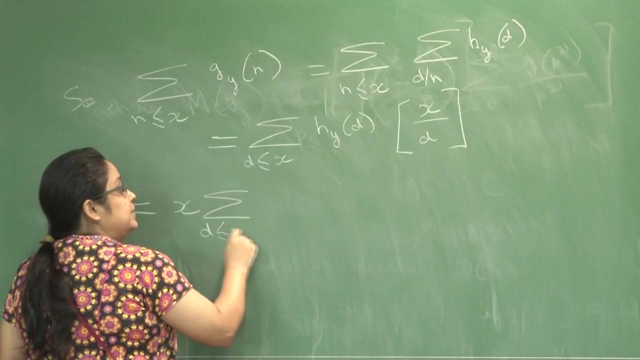 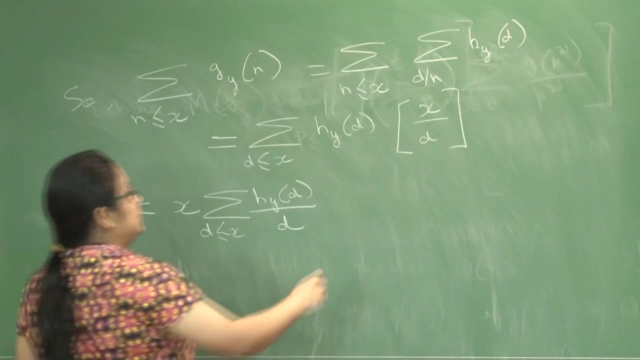 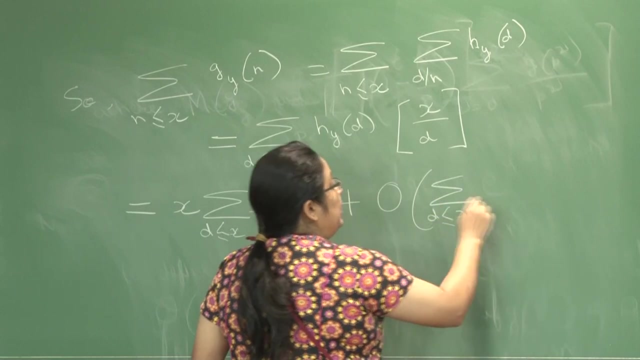 you can write this as x over d plus an error term of the form O of 1.. So you write this as x times. summation d up to x- h sub y of d over d plus O of summation d up to x- absolute h sub y of d. 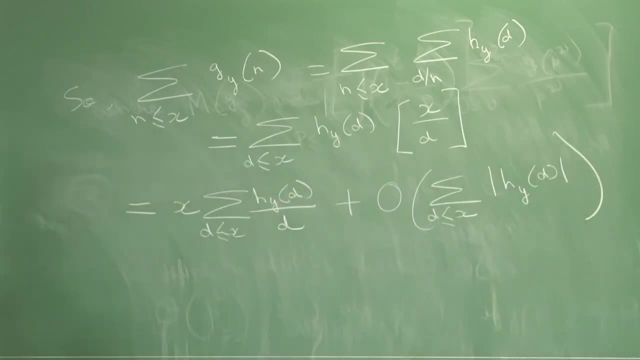 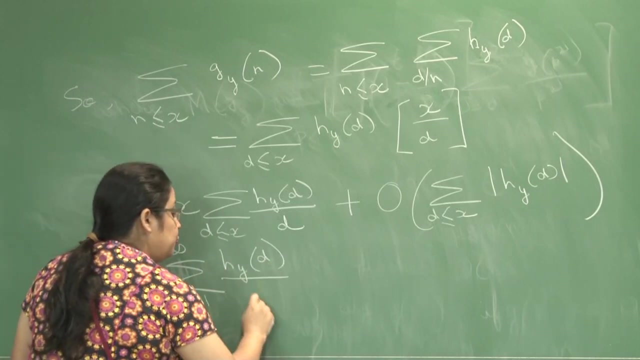 Alright, Now what we do is we write this as: d of x, D of x of x, absolute h sub y of d. Okay, Okay, We first consider all the numbers from one, all the positive numbers, So d going from 1 to infinity, h sub y, d over d. okay, 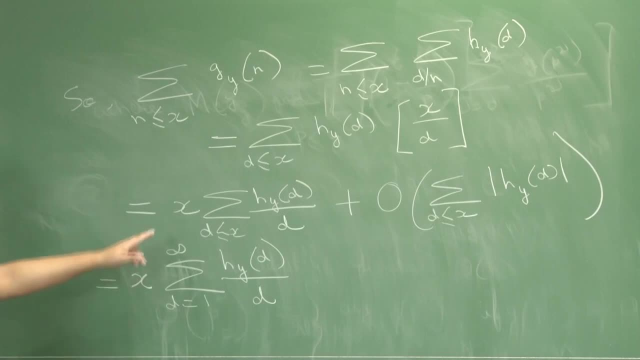 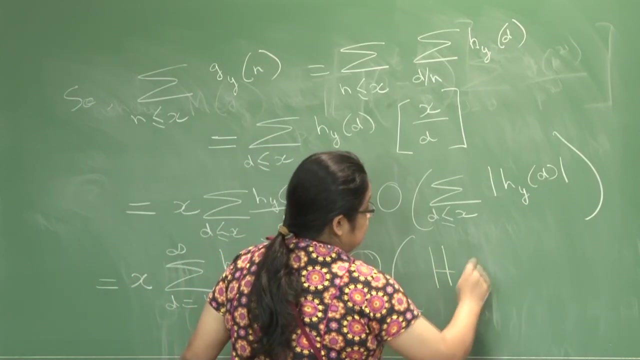 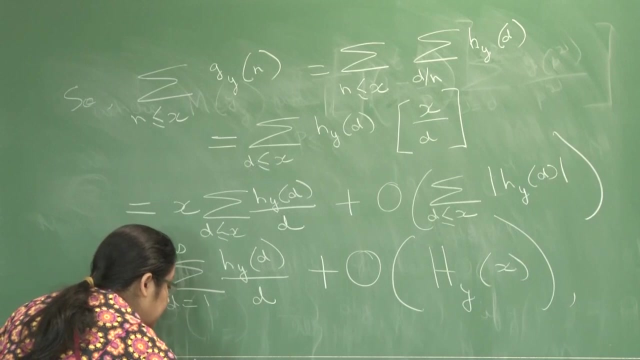 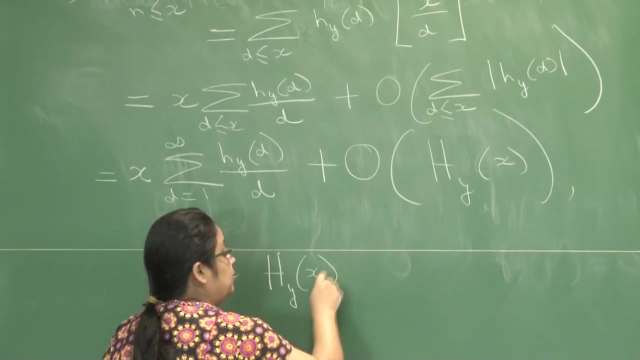 Then from this we have to remove those numbers d which are greater than x. So we have what we do, is we write this as plus o of another function, h sub y of x, where what is h sub y of x, It is first of all those numbers. 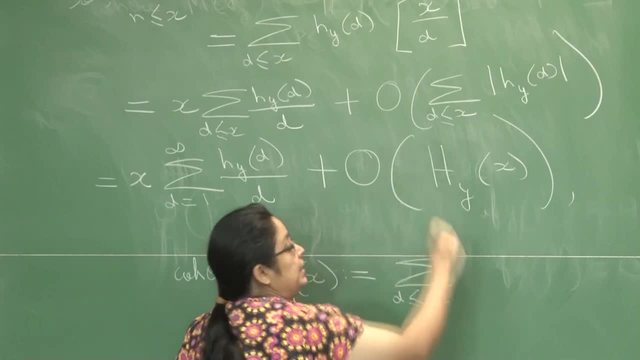 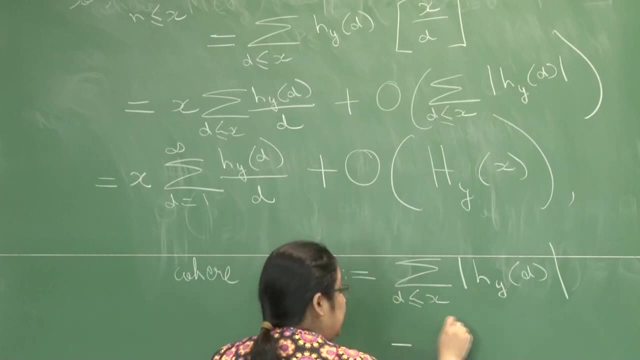 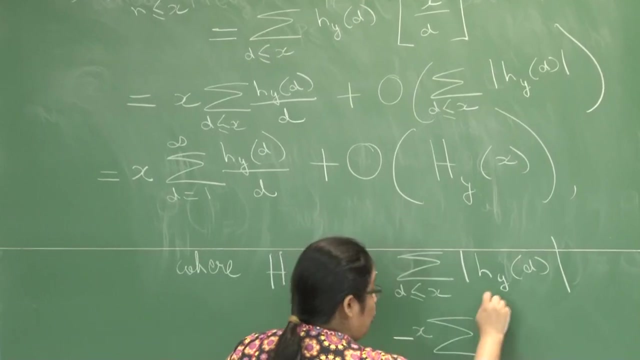 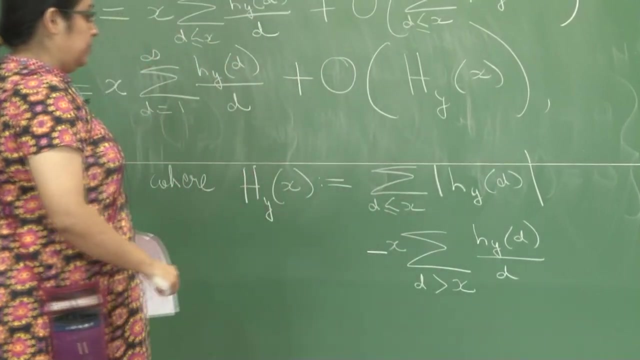 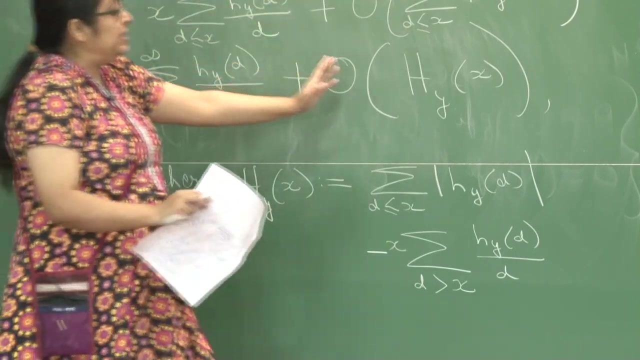 Okay, Those numbers running up to x, absolute h sub y of d, okay, minus I take x times d greater than x of h sub y of d over d. okay, And in fact, since we need this to be o, We- basically we need an error- estimate of h sub y of x. 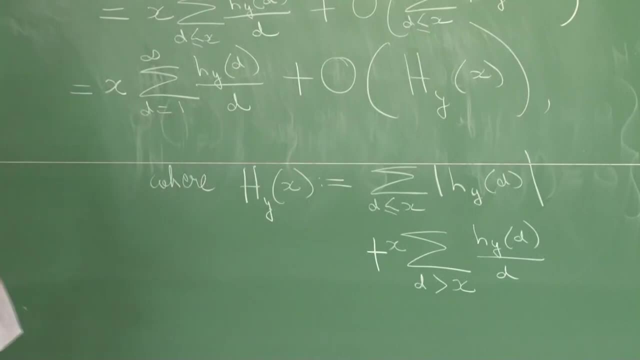 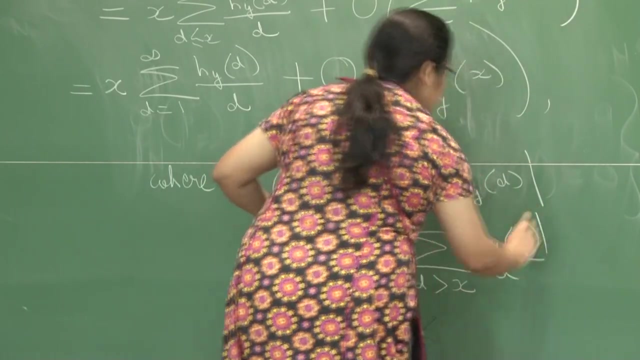 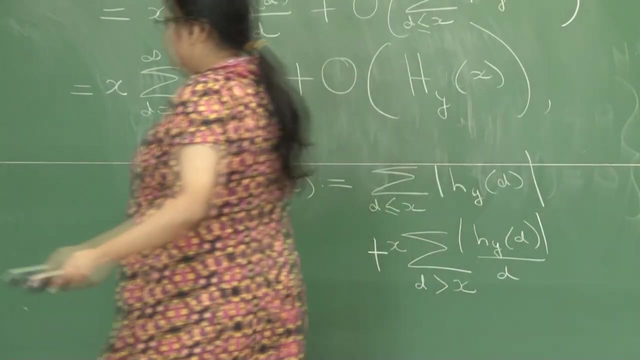 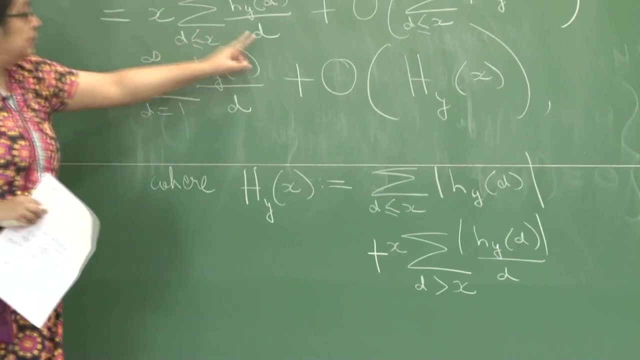 What we can do is that we can actually take this to be the sum. okay, And actually we have absolute h sub y of d is here. So what do we do next? We have to estimate what our h sub y of x is. 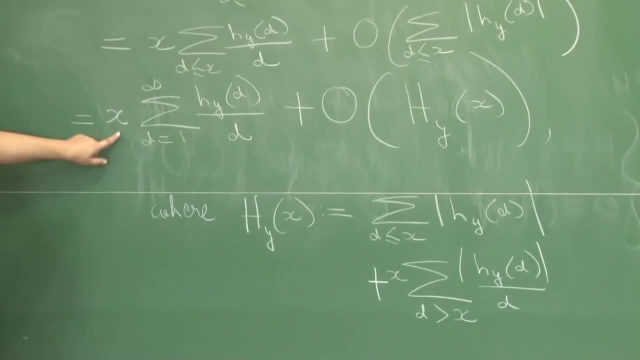 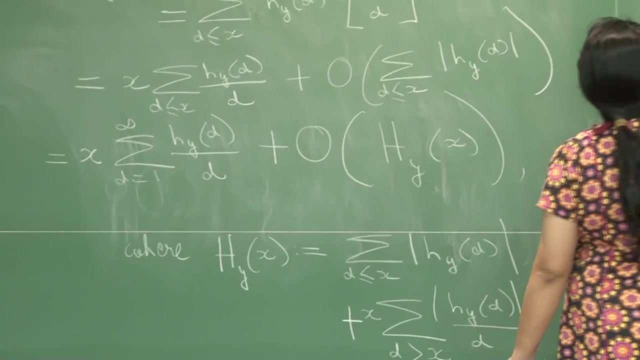 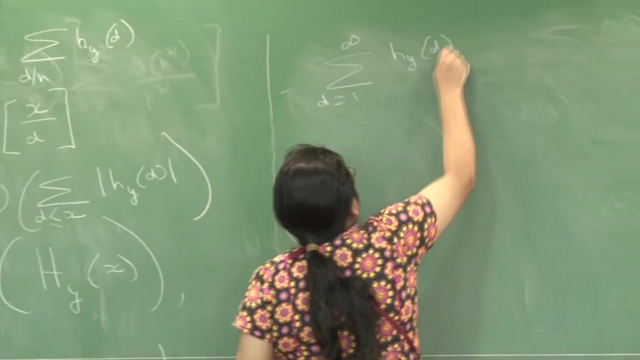 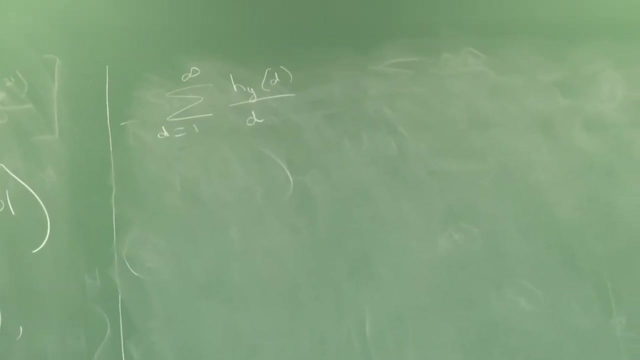 Of course we also have this term. Let us first just focus on this main term here. okay, Let us take our sum. So look at d going from 1 to infinity. h sub y of d over d: Now this is a multiplicative function. h sub y of d over d is a multiplicative function. 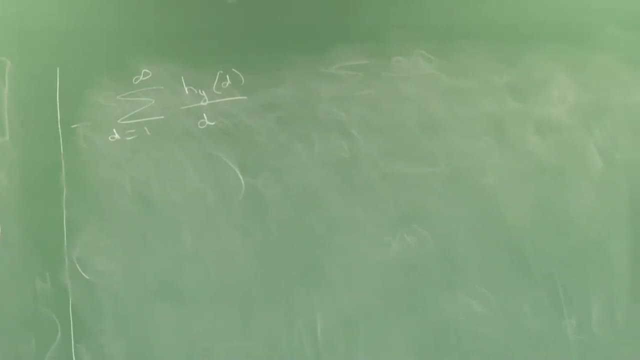 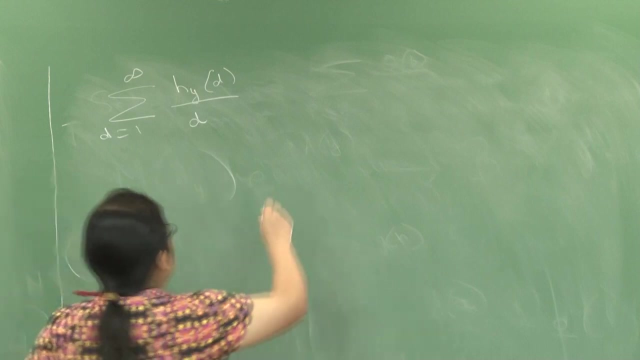 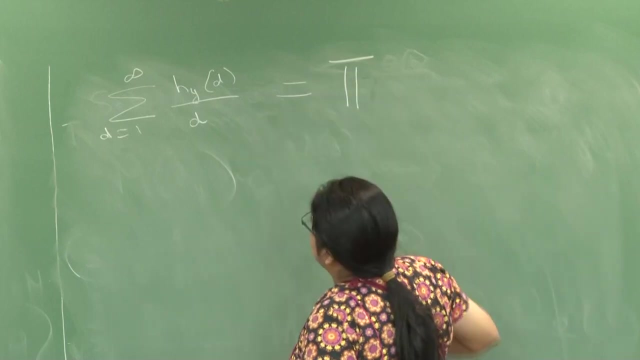 So we can write this in terms of an Euler product. Why did suitable convergence conditions hold? Now suppose, imagine that we do not have to worry about convergence conditions. What happens? Okay, so you have to write this as product of P up to y, and what do you have? 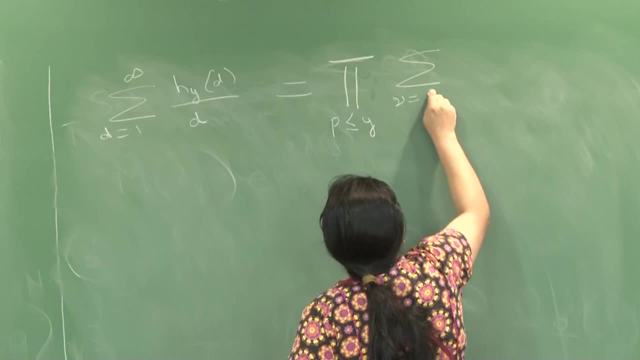 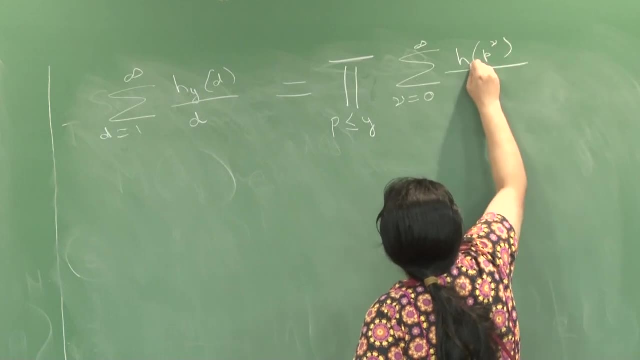 H sub y So mu going from 0 to infinity. H sub y So mu going from 0 to infinity. H sub y. H of p raised to the new. h sub y of p raised to the new. over p raised to the new. 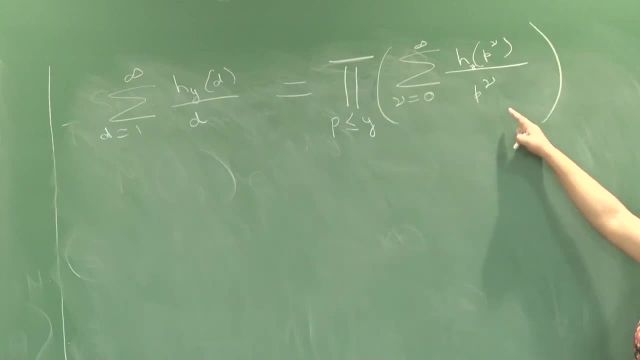 Now you see, the right hand side converges absolutely. okay, You can show that. So each of these sums converges absolutely because beyond a certain, yeah, so each of these converges absolutely, Since these are bounded above by some Law ofwives rule. 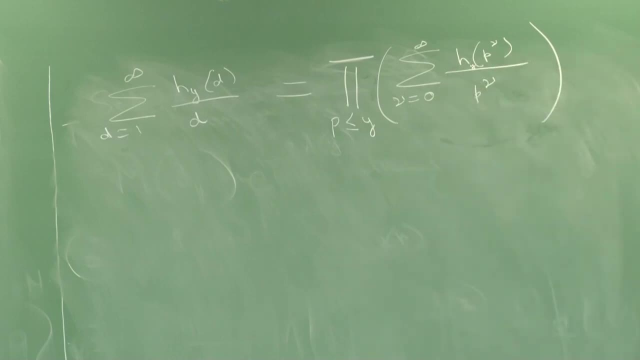 Okay, bounded above by some absolute constants and therefore their products, you have products over finite set of primes. okay, So the product also converges absolutely. therefore the corresponding sum also converges absolutely and therefore this Euler product is valid in this case. 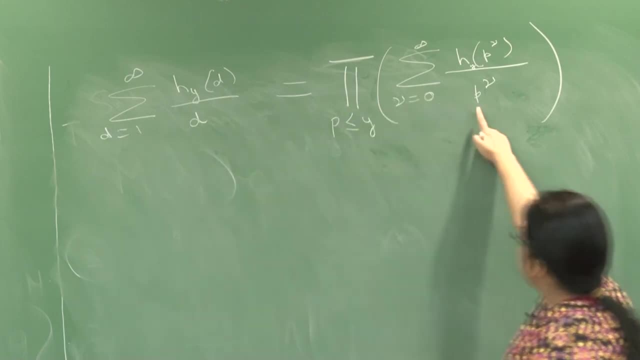 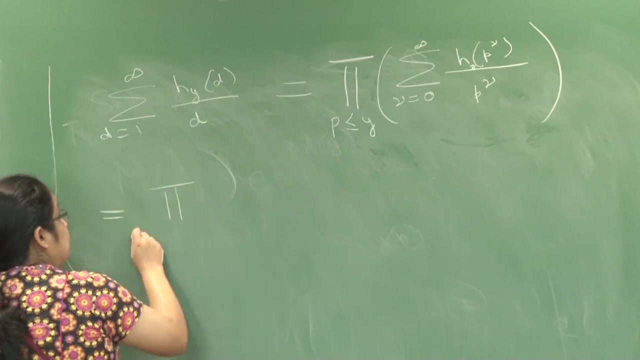 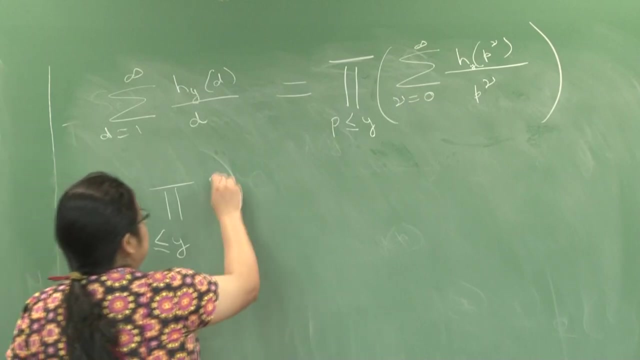 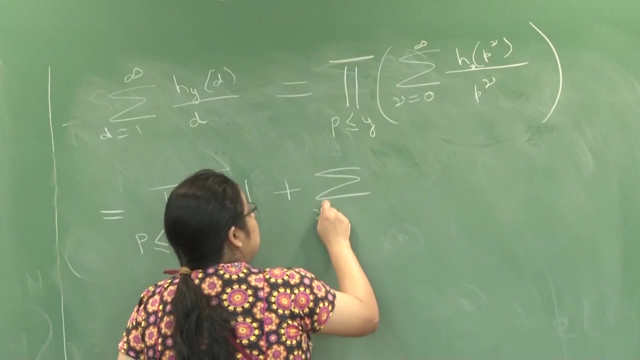 So if you want to study this sum, you just study the corresponding Euler product, which is what we do and we also. so what do we do here? We write this as product of all the primes up to y. okay, So for nu equal to 0, you just have 1, okay, plus nu going from 1. 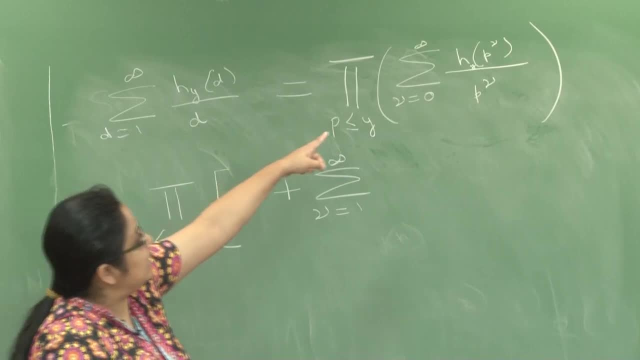 to infinity. But you already told me that you are going to write this as product of all the primes up to y. okay, So for nu equal to 0, you just have 1, okay, plus nu going from 1 to infinity. okay, So for nu equal to 0,, you just have y. okay, So the product of all. 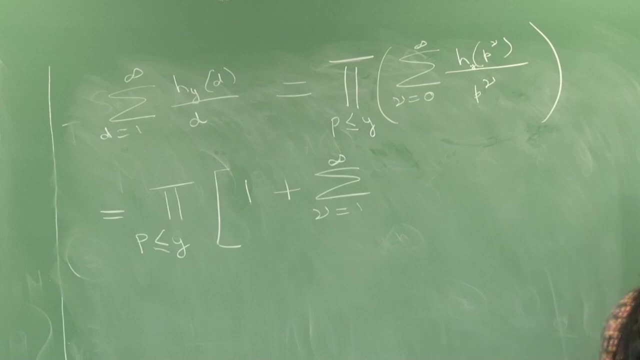 the primes up to y, tu rproimes up to y, and they are v to the minus num of the whole square, plus v to the x square. mu u cube alpha squared plus v to the beta square. so this is all about d rhythm, right? So you canоч10 the whole square system here there. 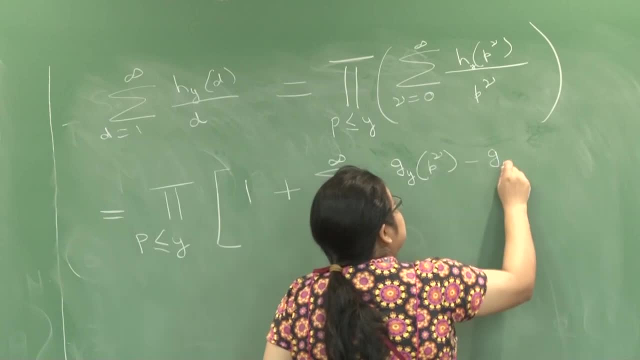 You can try to woven some simple Bayesian formula in 1, 0,. you can write such a formula to find out what function is seen in this particularis. Theному can be written as this: that what fa of P raised to the nu can be written as this: and thed knowing that your f sub y. 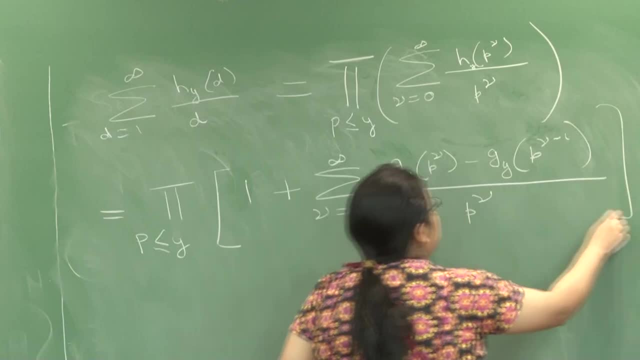 of P raised to the new can be written as this: So G sub y of P raised to the nu minus G sub y of P raised to the nu minus 1 over P raise to the new. Okay, these also convergent absolutely.